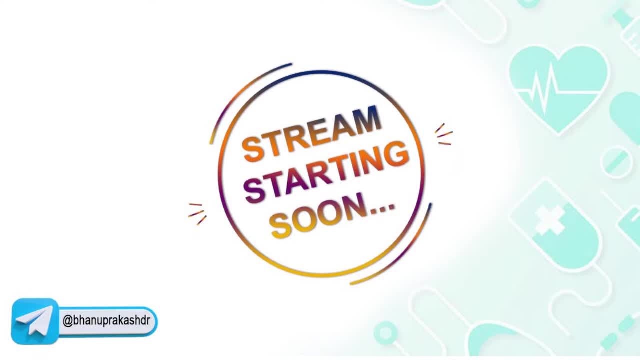 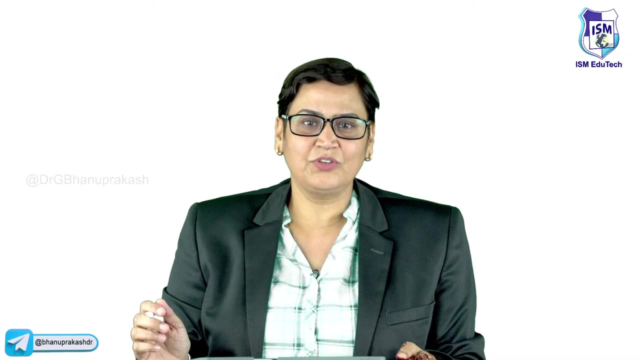 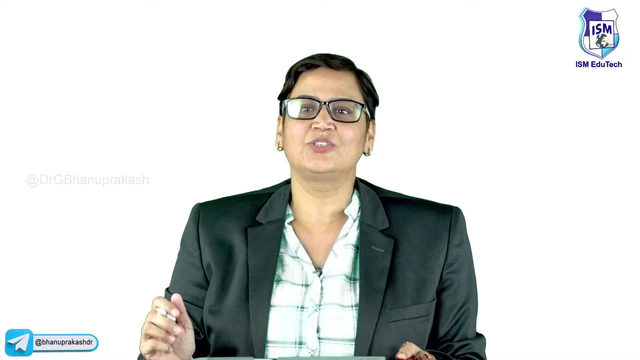 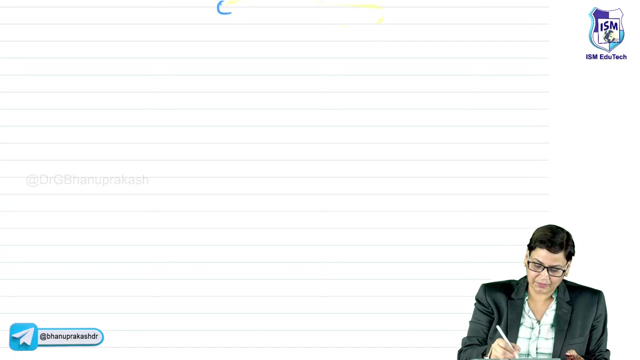 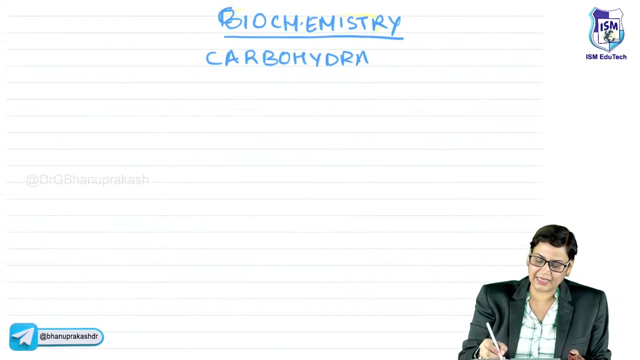 Thank you, Thank you, Thank you. Before starting up with carbohydrates, as it is clear from the word itself, carbohydrates are what They are: the hydrates of carbon, Isn't it? Hydrates of carbon? So there are so many definitions about these carbs. 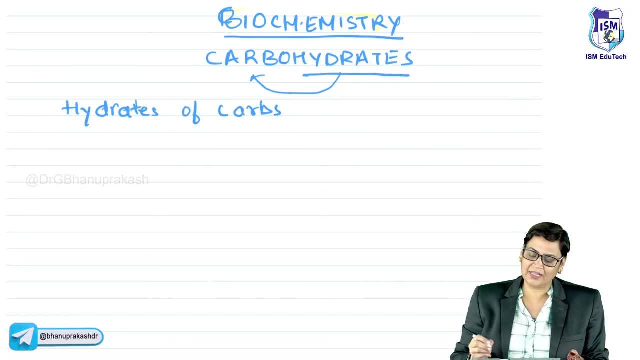 The earliest system of classifying carbohydrates was that carbohydrates are the ones which have carbon hydrogen and oxygen in the ratio 1 is to 2 is to 1.. But nowadays the widely accepted classification of carbs is that they are polyhydroxy derivatives of aldehydes and ketones. 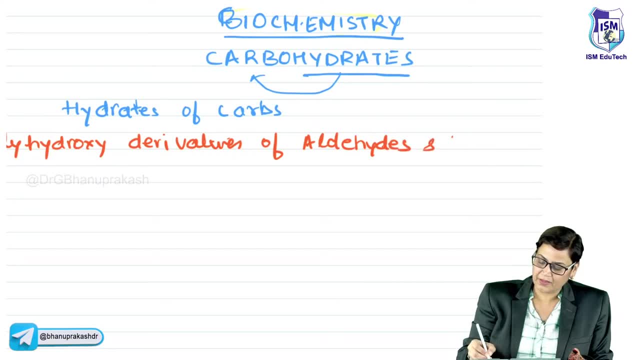 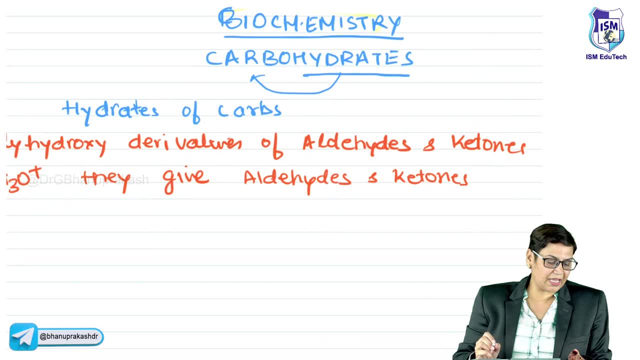 Since this is a live session, I am just waiting. if you guys have any problem, So you people don't hesitate to ask me in the chat box. Carbohydrates is a simple topic, but it is a complex one also, So we are here to tell you the complexity of carbohydrates. 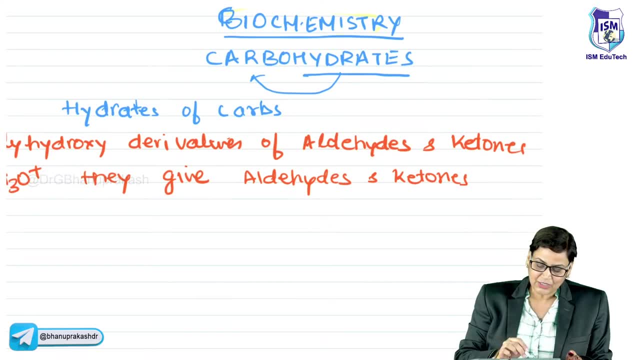 carbohydrates plus the simplicity of carbohydrates also right. so these are what polyhydroxy derivatives of aldehydes and ketones which, on hydrolysis, will give these aldehydes and ketones too. so that is why the first way of classifying them is that they are of two classes if they have aldehyde as the 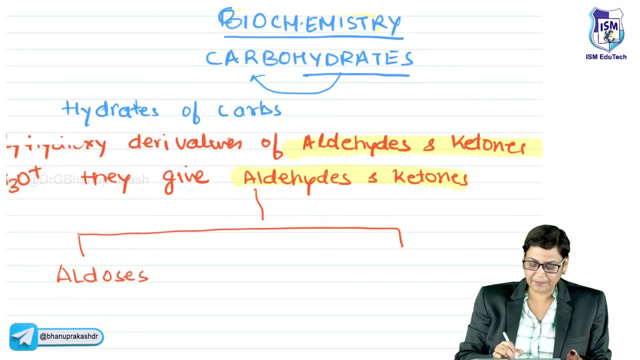 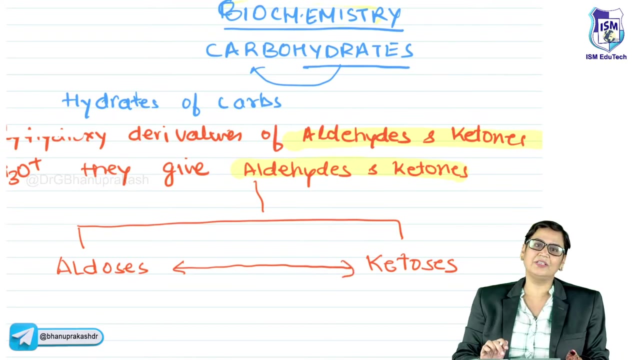 functional group, they are known as aldosis, and if they have ketone as the functional group, they are known as ketosis, and the interesting part about these is that these aldosis and ketosis are linked as isomers with respect to one another, and this is a very interesting 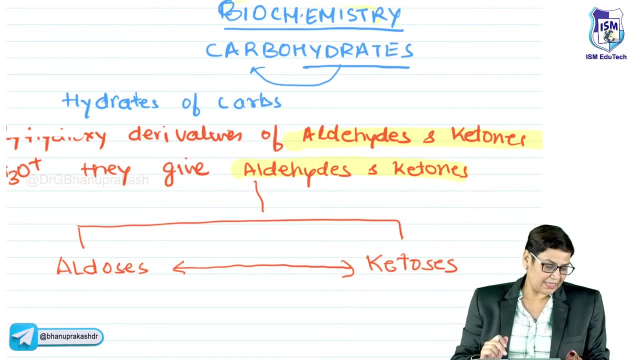 factor which takes place in the body- I can see Tamil speaker is better. this is. carbohydrates is a very generalized topic. it is for first-year MBBS students. it is for those students also who are preparing for their NEET exam, also those who are preparing for their INI CET, so it is a very common topic for all the 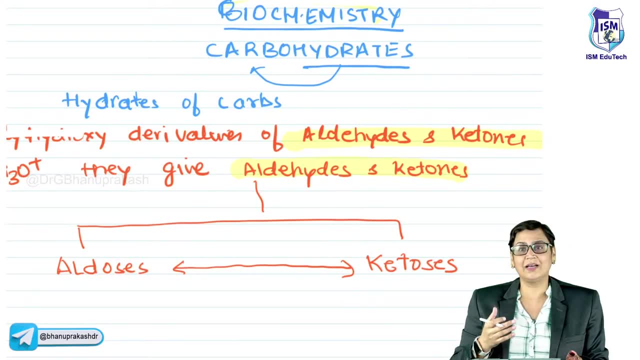 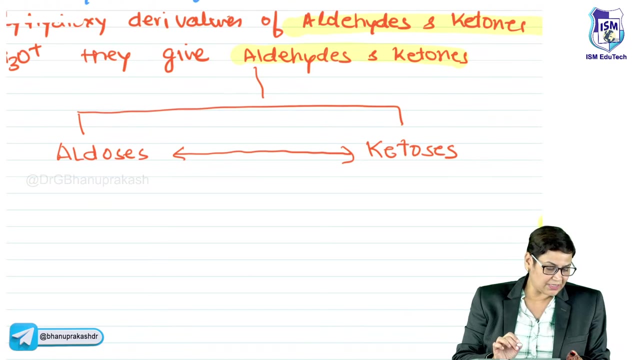 medical students. in fact, this is an important topic for those you know, future aspirin doctors also, who have taken medical as their subject for class in class 11th and 12th right. so LDL doses and ketosis, So L-dosis, Yeah, good evening. 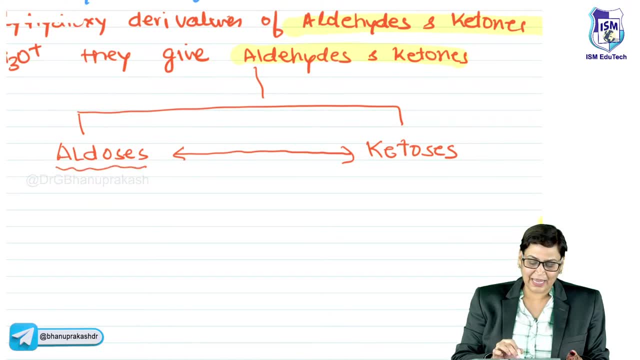 Nagesh, how are you? So? can anybody tell me L-dosis? What will be the principal functional group in this? The principal functional group in L-dosis will be always a aldehyde Right And for ketosis it will be a keto And it is so. 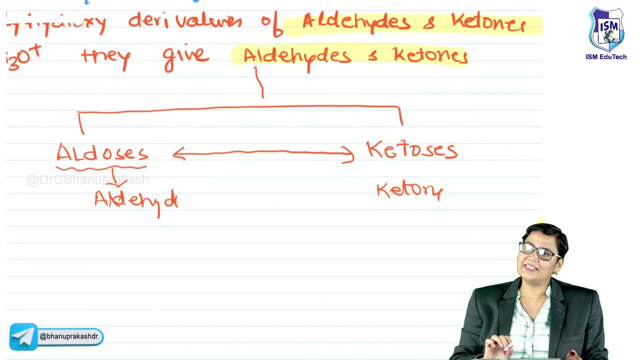 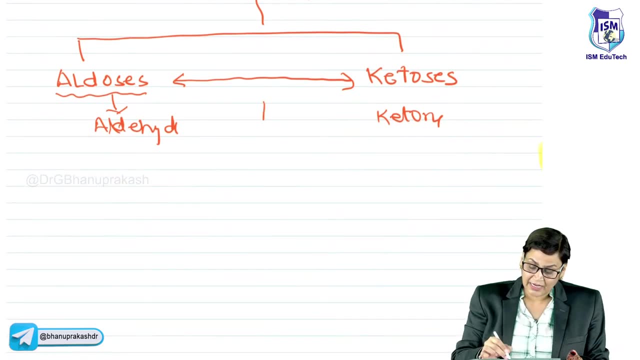 interesting that L-dosis and ketosis are linked as isomers and this reaction takes place in the liver also. Now, this is one way of classifying carbs. Now see, another way of classifying these carbs is depending upon the number of carbon atoms. So we always start a carbohydrate. 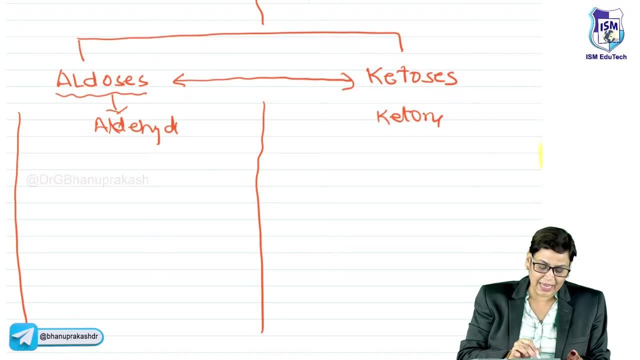 having three carbon atoms, which is known as a triose sugar, And the example of a L-dose triose is glyceryl aldehyde Right, And an example of L-dose triose is glyceryl aldehyde and ketose triose is 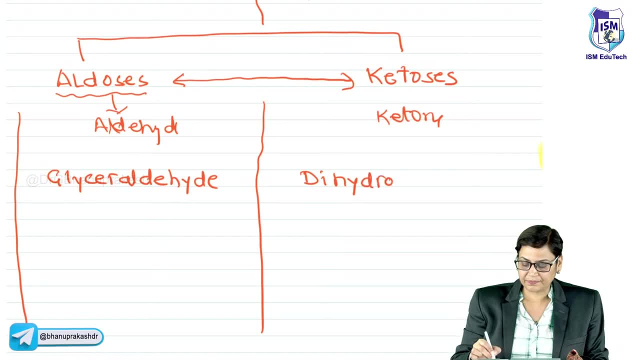 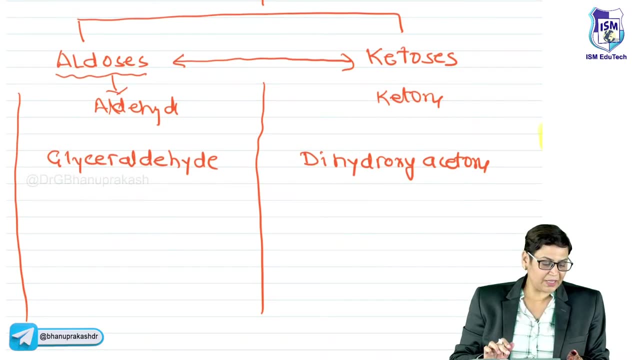 dihydroxyacetone Right. Very good Tamil speaker. I really liked your name, Tamil speaker. Okay, But you are speaking in English. That's nice, Right. Then coming over to if it has four carbon atoms. Four carbon atoms, that means it will be. 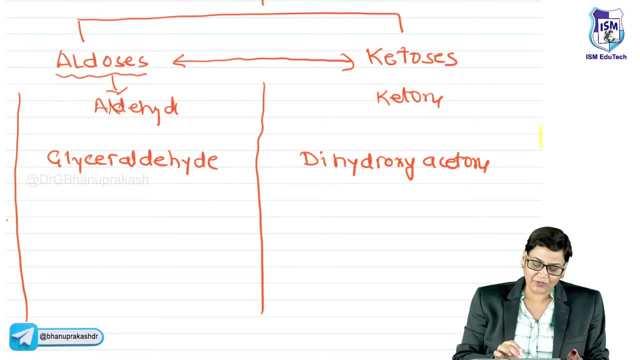 a tetrose- An example of a L-dose tetrose is erythrose and keto tetrose is erythriolose. And again, the interesting part is erythrose and erythriolose: they are linked as isomers. 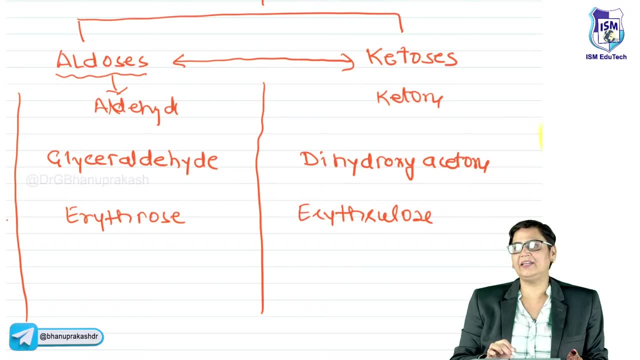 And these are the most important intermediates Of energy. Because why we eat food? obviously, carbohydrates are the universal sources of energy. You know me, people are fond of eating carbohydrates in the form of bread. is there, then, rotis? are there than these burgers and all? They are all carbs. 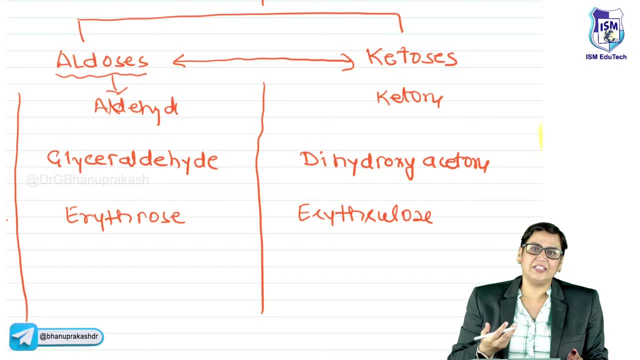 Right, So these are what These are energy giving. Then, coming over to five carbon atoms, it is pentosis. Now again example of pentosis. if I talk about aldopentose, the example is ribose. if I talk about ketopentose, the 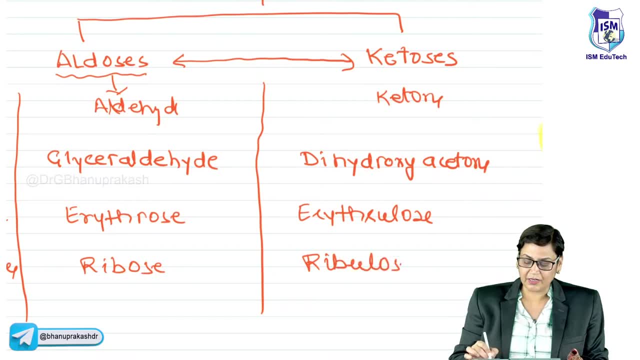 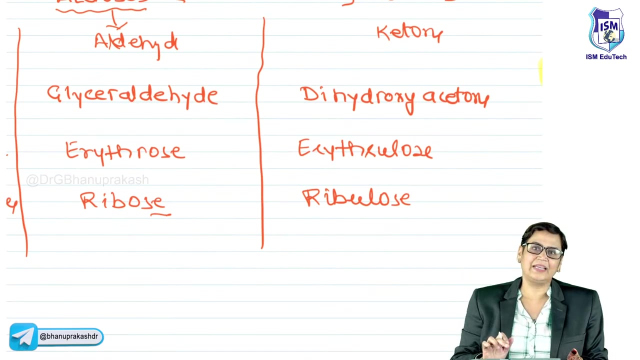 example is ribulose. now, all of you are familiar with DNA and RNA. ribose is the major constituent of DNA and RN. in DNA it is deoxyribose, in RNA it is a ribose sugar. again, ribose and ribulose are connected as isomers with respect to one. 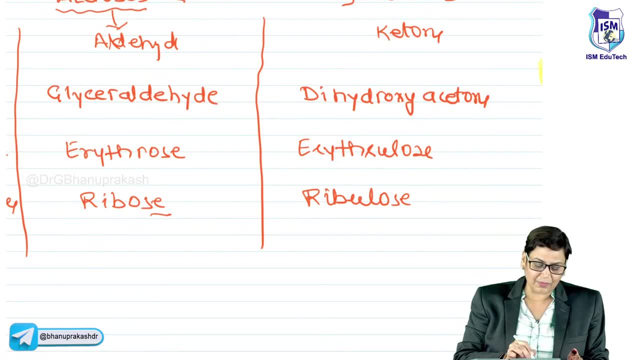 another. then, coming over to the next one, six carbon atom hexoses. elder hexos is glucose right and isomer of glucose is draco and fructose has more sweetening index than glue. fructose is a more sweeter sugar than, again, glucose and fructose. 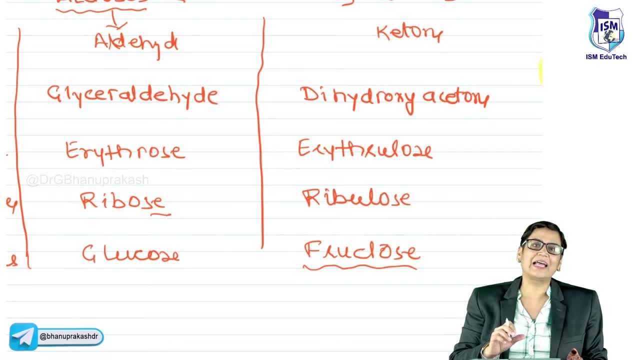 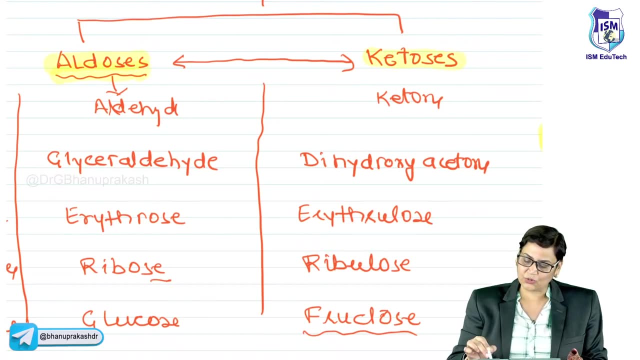 are linked as isomers. So this is one way of classifying carbohydrates as per their, first of all, the functional groups- You can see L-dose and Ketose- and then as per the number of carbohydrates. Then another way of the classifying these carbohydrates is as per their units, which 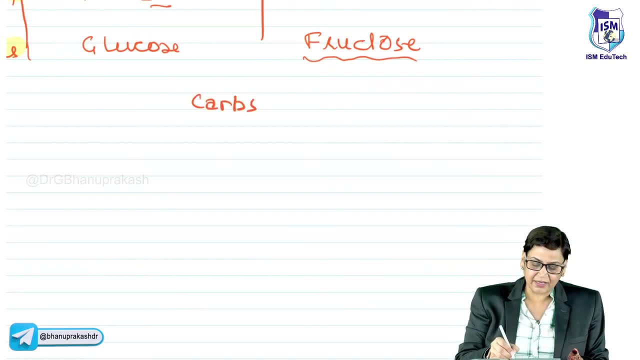 means that, as per their units, they are divisible into four major classes. Right, The most important, the simplest one is monosaccharide. Mono means single Saccharide. actually, saccharide is derived from, you know, because sugar, sugar is derived from sugar cane. 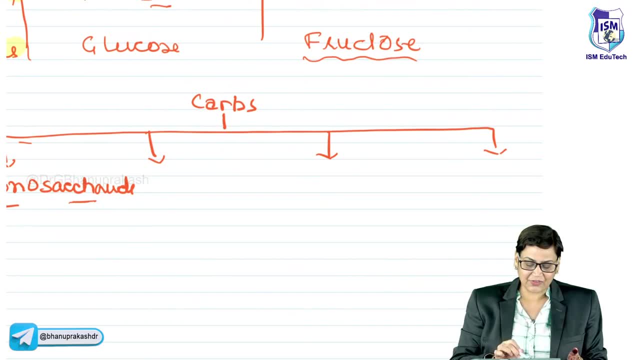 And the botanical name of sugar cane is saccharum, So that is why we always write saccharides. Mono means single, Then if we talk about two, it is disaccharide. Is any sugar have more than one L-dehyde and ketonic group? Yes, of course, But the principal. 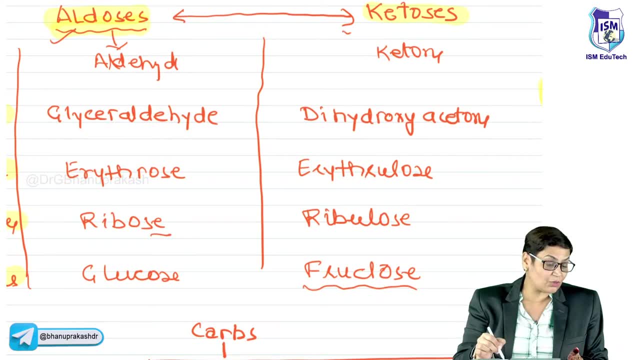 group will remain the same. Principal group will be in L-dose and Ketose only. It cannot change. Depending upon, the carbon atoms will change. I mean speaker. can I get your original name please, If you don't mind, Or otherwise? 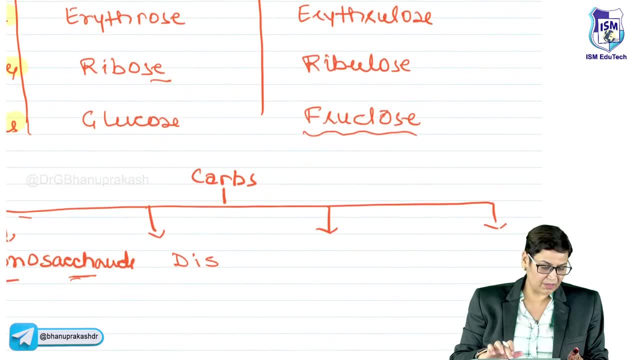 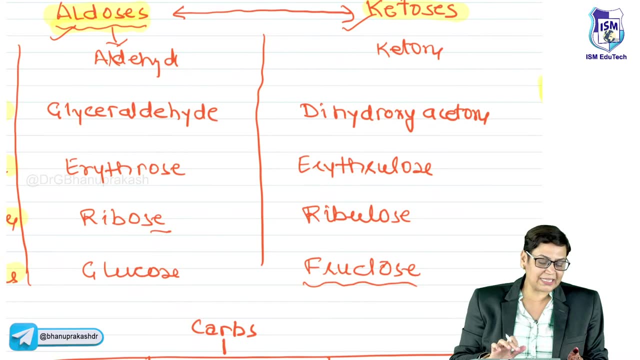 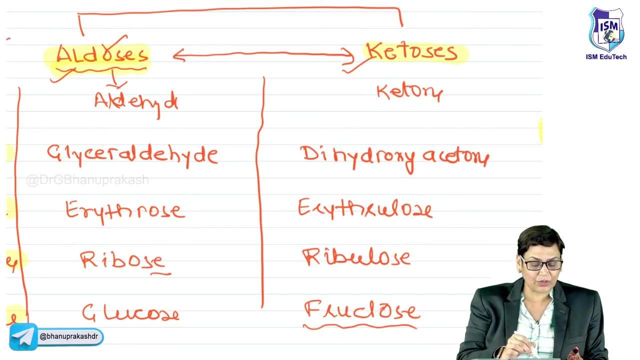 can I call you TS? Okay, Sanjay. So, Sanjay, beta, what I am trying to tell you here is: your question is: L-dehyde is the main functional group. I will just show you the structures, also open chain structure, Then you will see L-dehyde. C-H-O cannot be two, But yes. 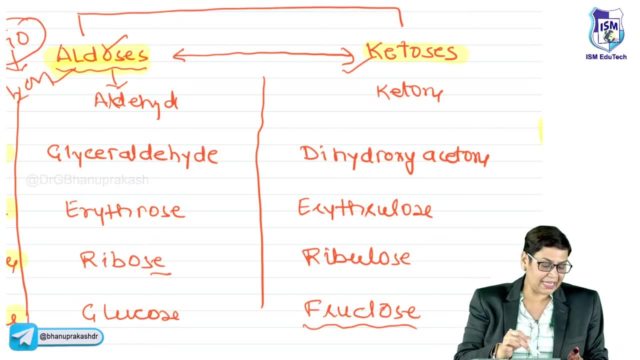 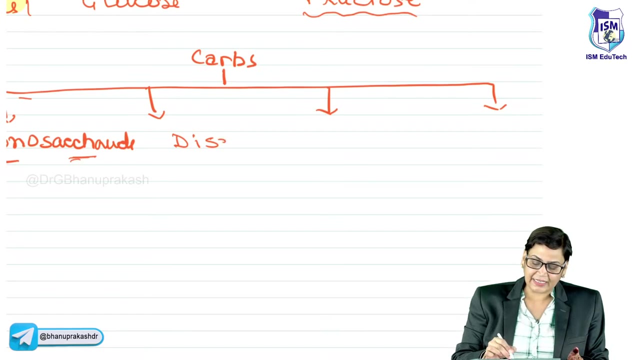 C-H-O and C-H-2-O. C-H can be there. So this is an L-dehyde and this is what This is: an alcoholic group, Clear, So yeah, So, depending upon the number of units, monosaccharides are there, Then disaccharides. 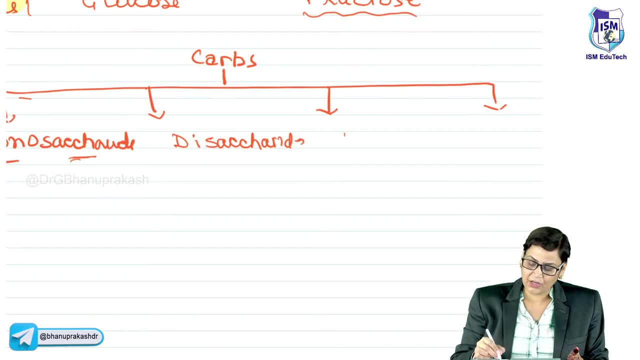 are there Again, it is clear: diamine A2.. Then oligosaccharides, Then comes polysaccharide. So in this section of chemistry of carbohydrates, we are going to discuss each and every unit one by one. What is this biomedical significance? How much we have to eat, in what quantity we? 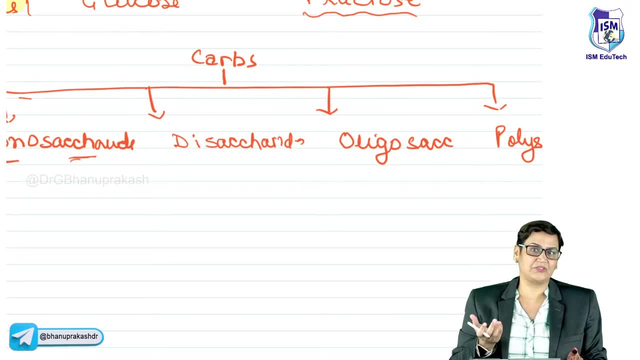 have to, Because ultimately, you know, we are studying biochemistry. Biochemistry, it is the chemistry of the biomolecules. What is happening inside our body when we are having this much of carbohydrate? Because nowadays, you know, this diet plays a very, very important. 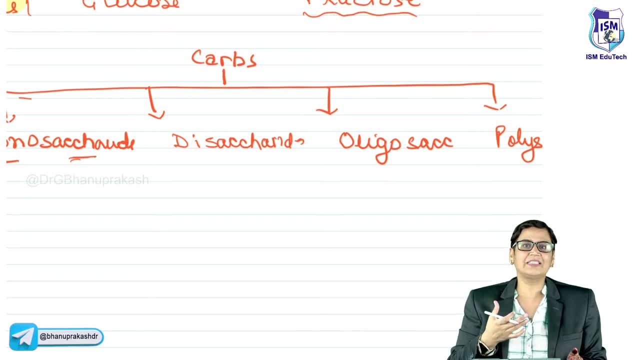 role in our body. In fact, it plays a very, very important role in our body. In fact, it plays a very, very important role in our body. In fact, it plays a very, very important. Diet is the one which is actually regulating the entire body, isn't it? So how much carbs? 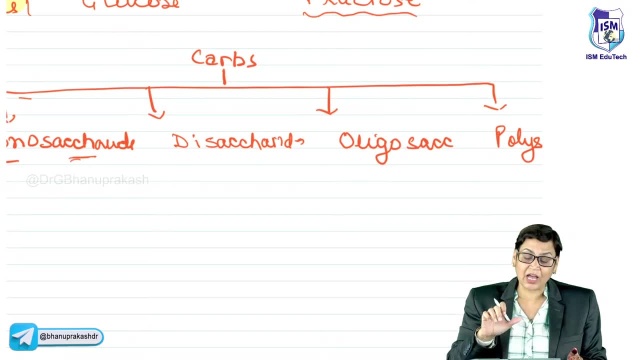 we have to eat How much glucose, we have to eat How much fructose, Because we cannot go to the shop and we can ask for glucose. no, We can ask only for a particular dish, How many carbs it is containing, How much calories we are consuming, What role it has. 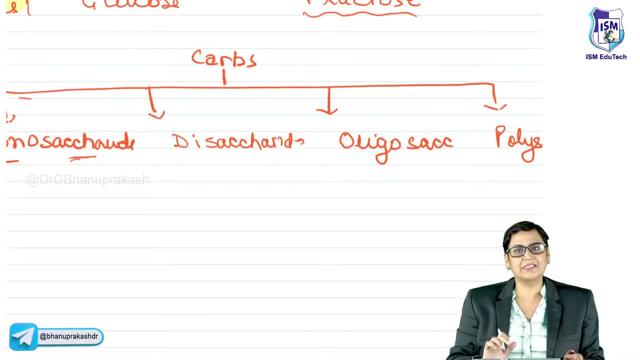 to play in the body. That is all what we are going to cover in this. So chemistry is very, very important to understand biochemistry, Because I have seen most of the students saying biochemistry is a volatile subject. you know, it just evaporates, just goes off if you try to understand the chemistry. because 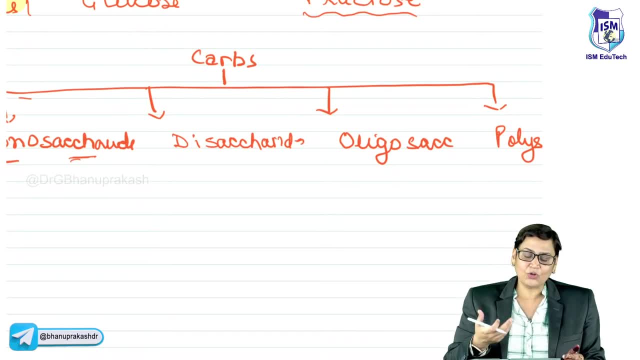 whatever is happening, it is happening inside the body, so automatically you know. it's all your perception of mind how you take it. so it is the chemistry, what is happening inside the body, because if anything goes wrong it leads to diseases and being a doctor, we should know what kind of disease it leads to. so 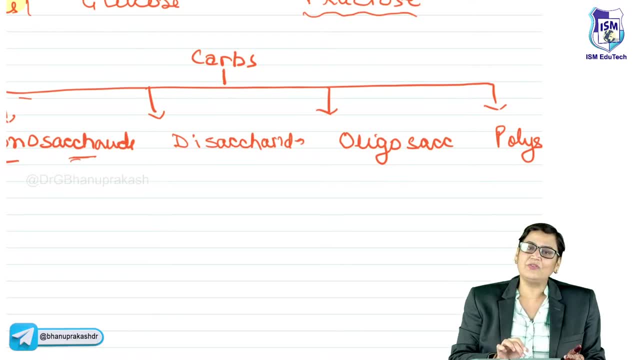 that we can regulate right. so that is what we are going to study: what are monosaccharides, what are disaccharides, what are oligosaccharides, what are polysaccharides? so mono means single, as it is clear from the word itself. 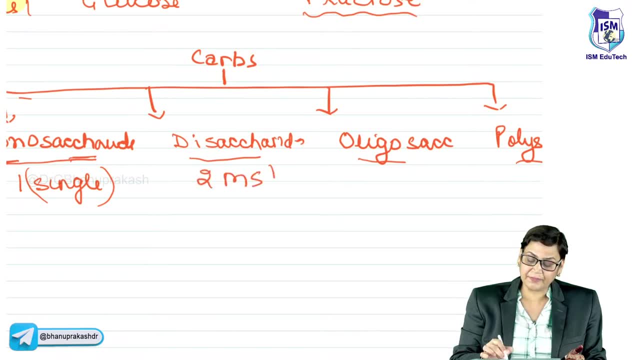 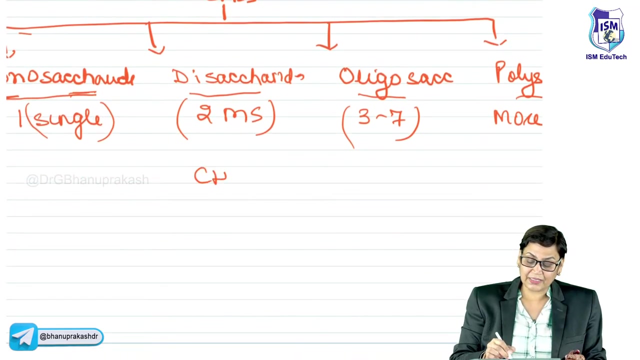 di means when two monosaccharides combined, oligo means when three to seven monosaccharides combined, and poly means many, when more than seven combined. so these are the two different ways of classifying the carbone. now the topic of today's session is chemistry, so we will be studying the chemistry of 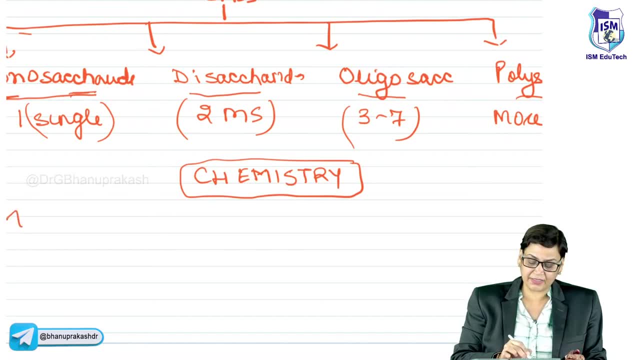 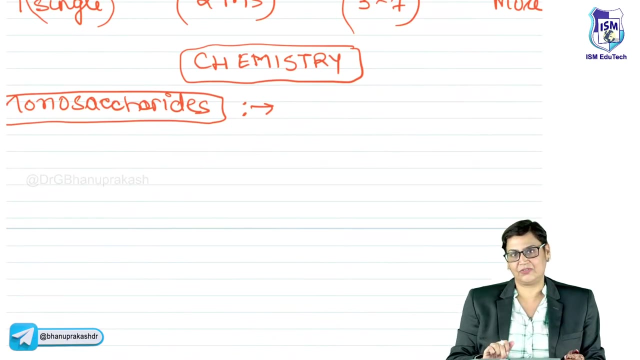 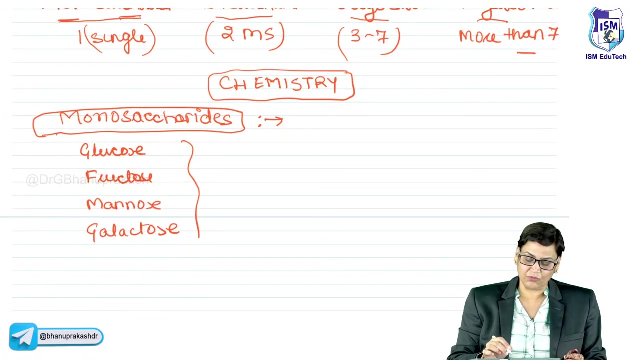 first of all, the monosaccharide. right now again, what all we are going to study in the chemistry? first of all, what are the example? the examples of monosaccharides are glucose, fructose, mannose, galactose, right, what is the chemistry means? what kind of? what are their structures? 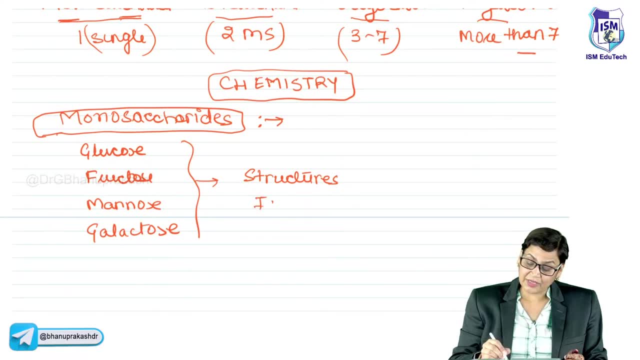 corpied of hands, what kind of isomerism is present in them? because always remember- here we are talking about the body, and always remember one thing: everything tends to go in a stable conform, like if two. right now you are attending my lecture. some, some people must be, you know, just attending the. 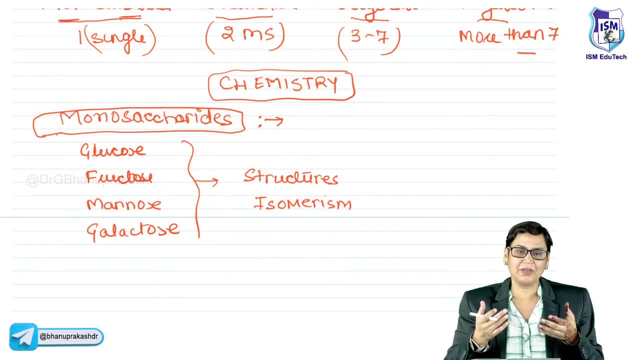 lecture, like sitting some means. everybody tries to go in a comfortable position, some people, like you know, listening to the lecture while lying down. some people table and a chair. so same is the case with these all: glucose, fructose, mannose and galactose. they always tend to go in a stable conformity. that is what is the structure and isomerism all about. 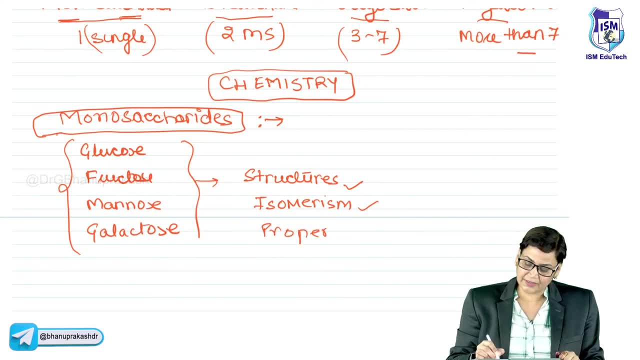 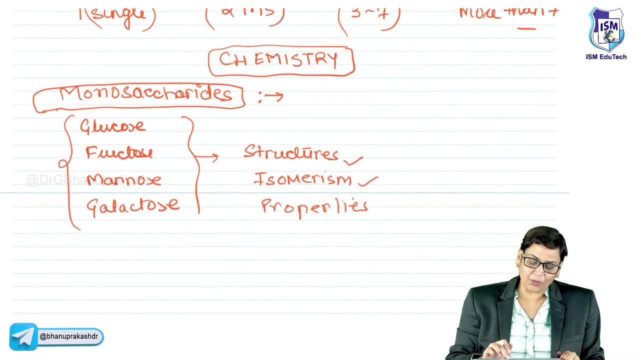 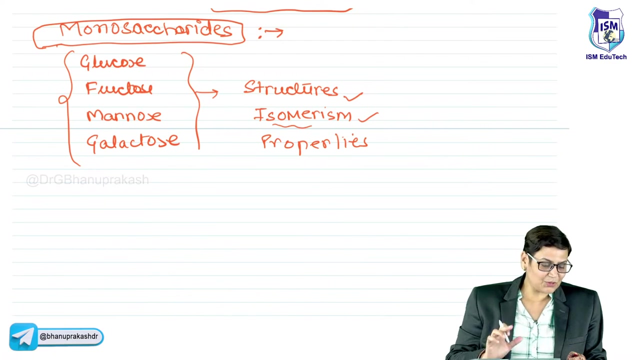 then we are going to study the properties. yes, i will come to the optical rotation behavior. optical rotation will come in the isomerism. yes, apple mania. what is your actual name? can you please tell me your actual name, if you don't mind, because apple mania seems to be, because i am also using an apple. 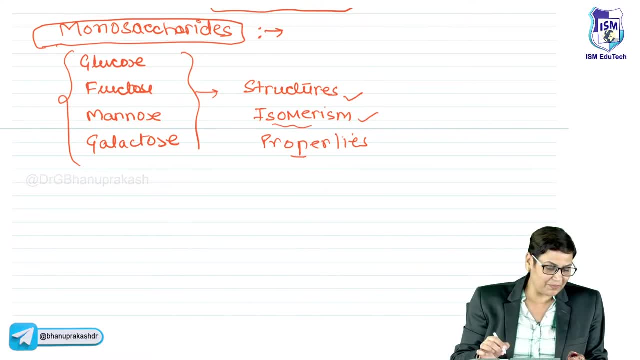 thing. so you know it will create confusion in my mind, so please share your actual name. yeah, it's my pleasure, sanjay. yes, okay, so optical rotation, we will be discussing in isomerism, it will come right. so, structures: we are going to study isomerism because everything depends on the structure. and then what are the? 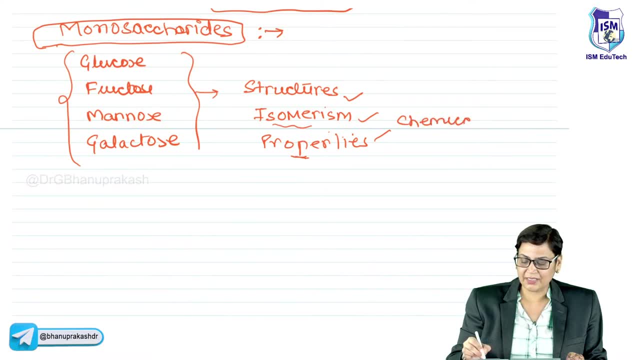 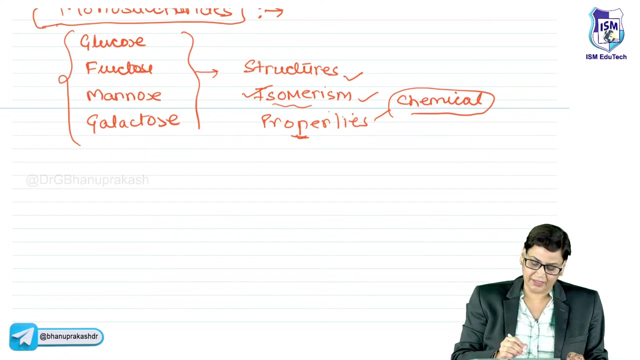 properties, whether. what are the chemical properties? mainly, we will be focusing on the chemical properties, right, sagar? okay, sagar, right. so now, first of all, we will start up with the isomerism. on my isomers. all of you are familiar with isomers. you have been studying isomers from donkey's years. 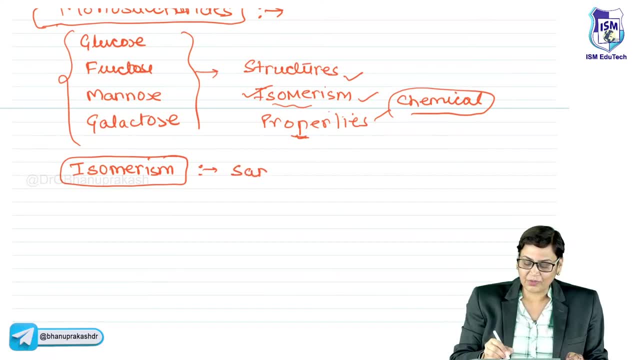 isomers are what the? the isomers are defined as those compounds which have a same molecular formula- you- but exactly different structural form. oh, as in its Entity, bent брrendan to efferently. Let's say, for example, if I talk about glucose and fructose, you know C6H12O6.. 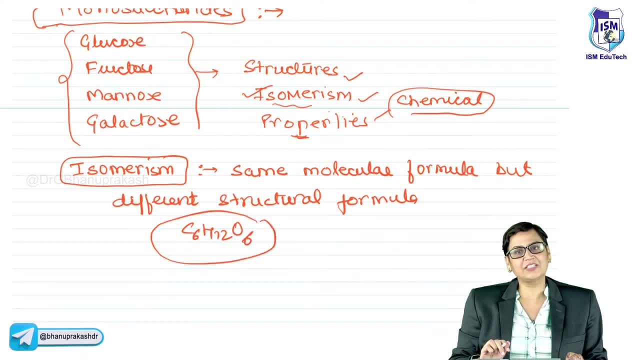 In fact, if I talk about all, they all have C6H12O6.. But what is the difference? Because whenever we talk about the body, there will be a difference. There will be a difference in the metabolism of glucose in fructose, in mannose and galactose. 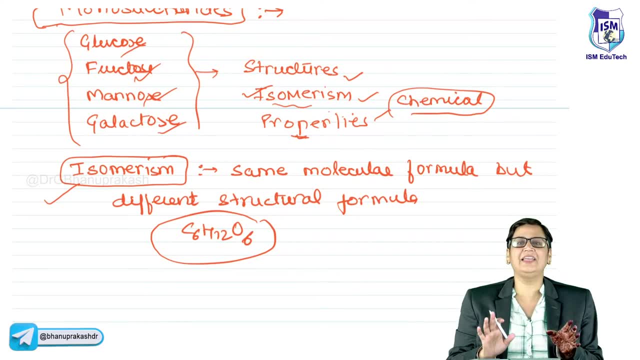 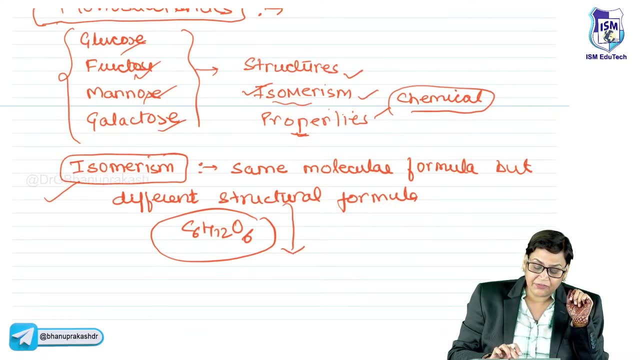 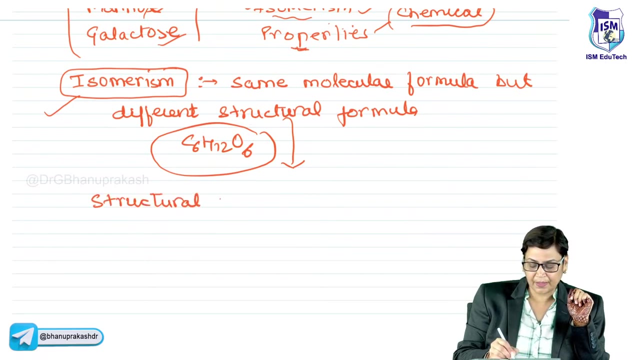 Right. So isomerism is simple. This is a widely accepted definition. Just keep it that way: Same molecular formula, but different structural formula. If they have a different structural formula, they are known as structural isomers. It is simple. 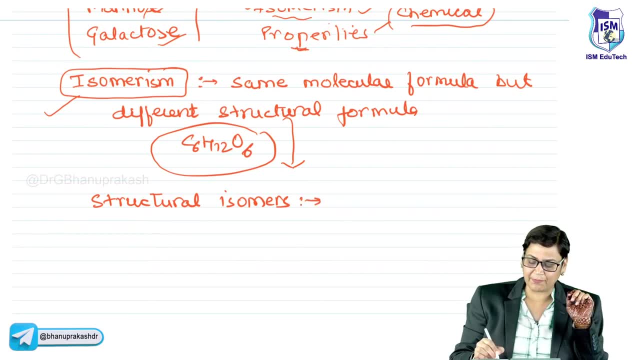 Very plain and simple Structural isomers. example is you can say glucose, fructose, Because glucose is, It is having an aldehyde as the functional group. So I can say glucose is what Glucose is, a aldohexose. 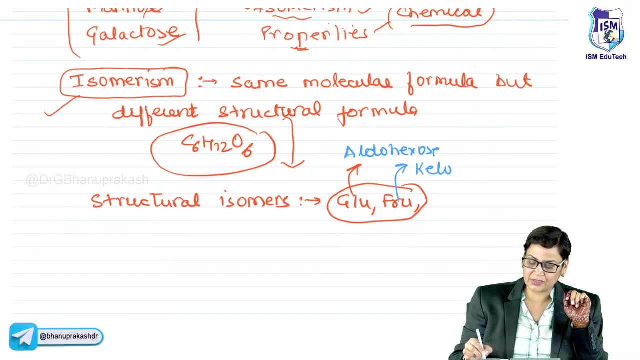 And fructose is a dohexose Right. Yes, they are the functional. Very good, Sanjay. They are the functional isomers also. They are the structural isomers also. So why functional? Because there is a change in the functional. 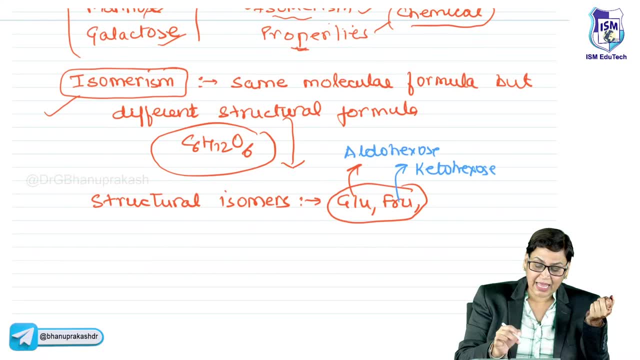 Right. Then second important Type of isomerism, which is actually very, very important from examination point of view, Also stereo isomer. Now see Stereo. Stereo means isomerism, simple, Same definition, But if they have a different orientation, as per in the space. 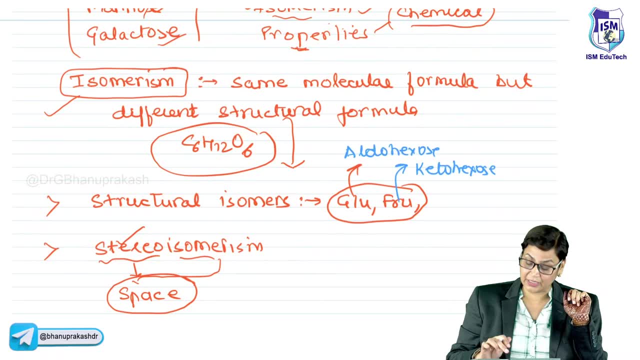 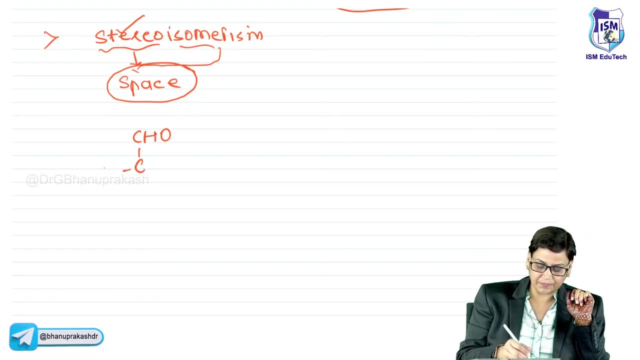 Yes, That comes from Stereo isomerism, Because if I show you the structure of glucose, See glucose is having this structure As such, you don't have to mug up the structures In case, if you can mug up, 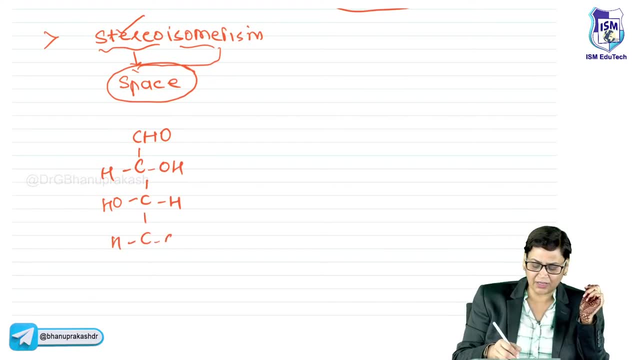 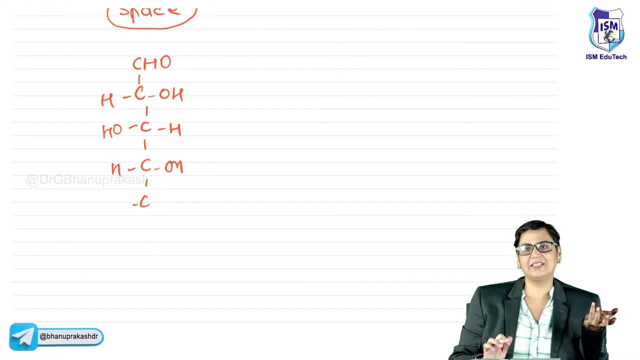 Well and good, But I won't suggest you, You know, don't get panic if you don't remember the structures, Because ultimately, once you get anything in the body, What is happening inside the body That you have to remember? 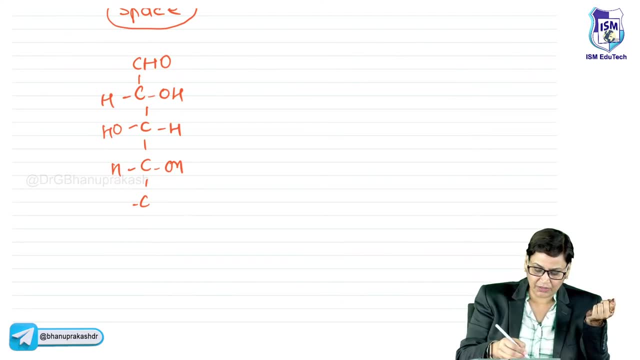 Okay, So this is 1, 2, 3.. 1,, 2,, 3,, 4,, 5. 6. Right, This is having an LD height, as it is clear: 2., 3,, 4,, 5 and 6.. 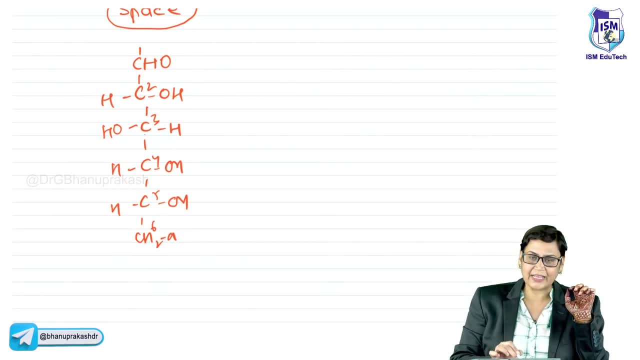 Now see, Just for your this thing: Hexo sugar, 6 carbon atoms, Right, Aldo hexose. LD height as a functional group. So it is a aldo hexose. Okay, So this is the structure of glucose. 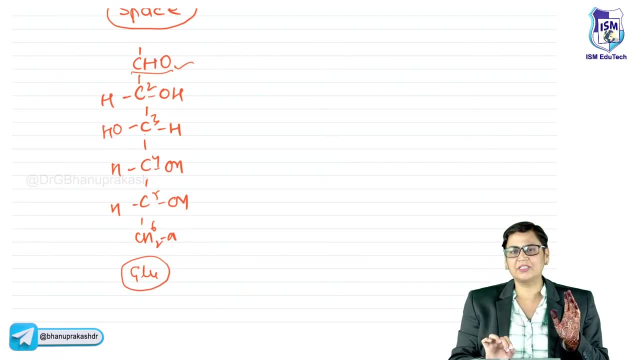 Now you must have seen. All of you have studied. You know chemistry. You have been studying chemistry from class 9.. So you must have studied this D, glucose. We write it like this, So from where this D comes from. 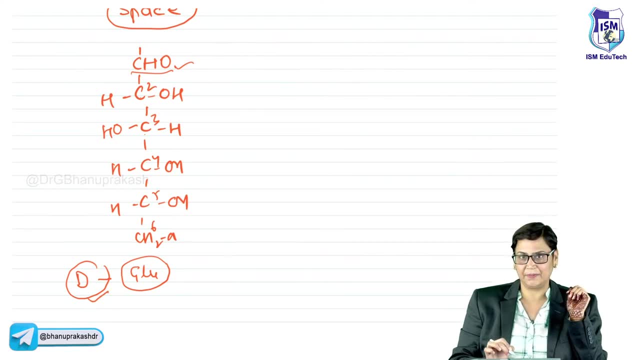 Have you ever given a thought From? what do you mean by this D? I will ask you, Sanjay Sagar, Can anybody tell me Now? I know you will say dextro or levorotate. This D is actually the orientation in the space. 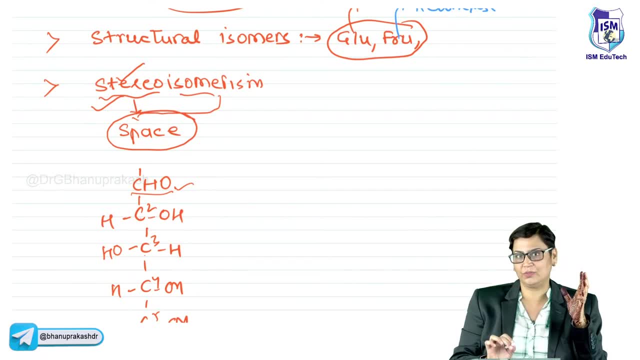 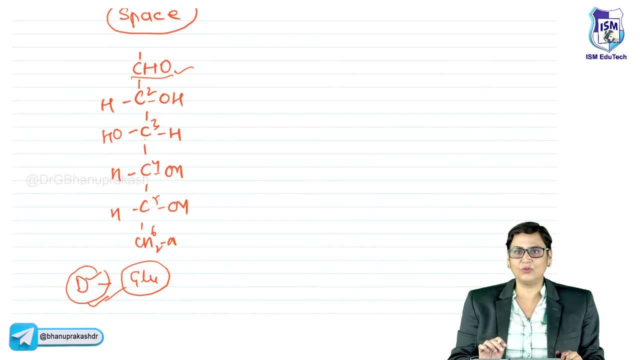 And these are known as stereo iso. I will come to that Now. how can we, just by looking at the structure of glucose, We cannot say D glucose, Isn't it? We need to have a standard molecule With which we can compare glucose and assign a configuration. 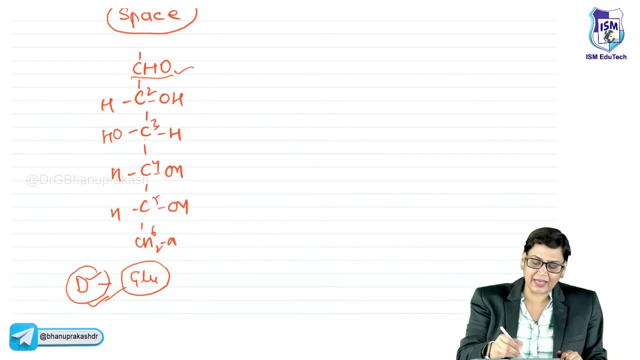 So that standard molecule is glycerol L. Just try to understand this concept. It is very simple: Glycerol aldehyde. Now tell me: Yes, very good, Sanjay. Fifth carbon atom has OH on the right hand side. 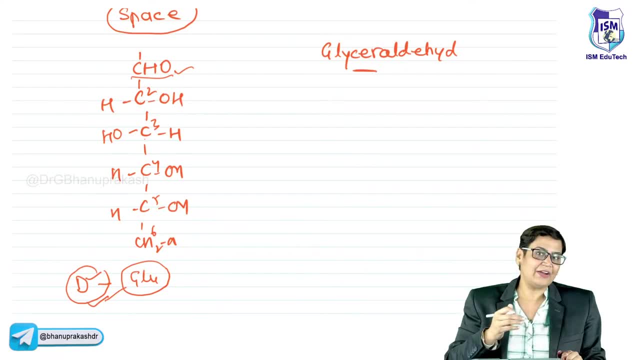 But how we came to know that it is D? We have to compare this structure. It is something. Cis and trans is all together different. Don't go haphazard, Just move step by step. This is same side. Trans is opposite side. 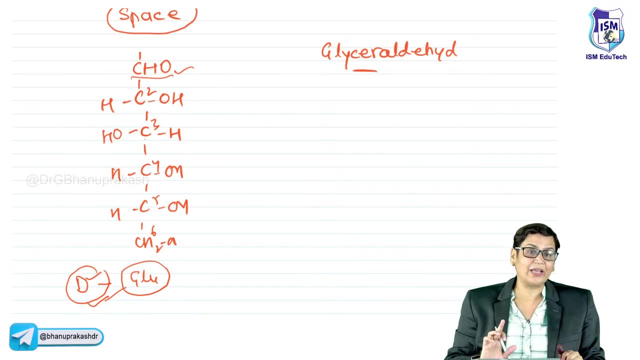 I am coming to that. Here. we are talking only about stereo, isomeric, Okay, So don't get deflected by different terminology. I just come to that. See, if we talk about glycerol aldehyde, all of you know. 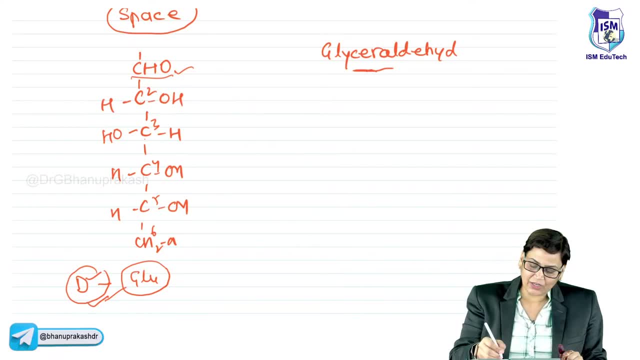 Yes, Very good, Nagesh, right. So glycerol aldehyde, if I talk about, I can write the structure of glycerol aldehyde like this: Yes, very good. And CH2OH, If I say first of all, let's look at this carbon atom. 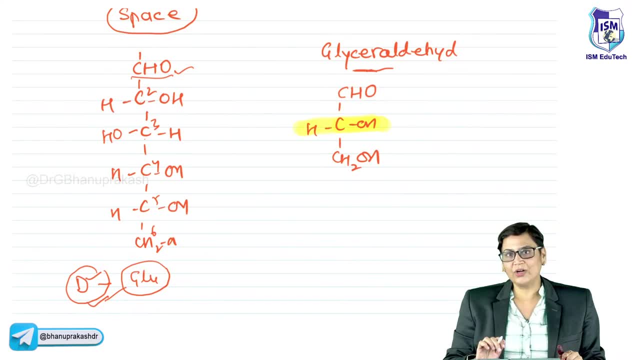 This carbon atom. Okay, you know what is the significance of this carbon atom. This is a chiral carbon atom, first of all. Now, what is a chiral carbon atom? It is also known as a asymmetric carbon atom. And now see, with this D terminology only, there will be so many terms which will come up. 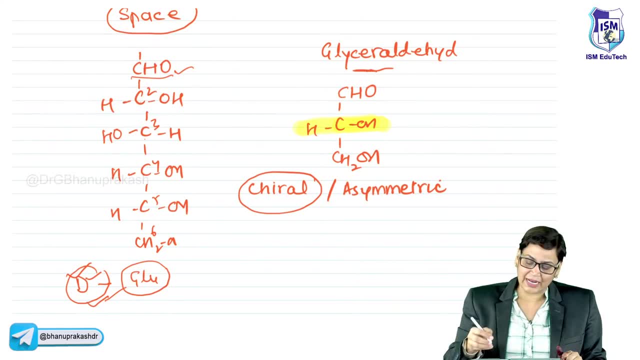 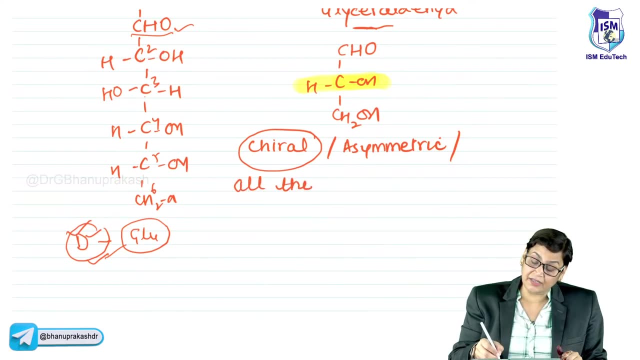 Right, So this is a chiral carbon atom. This is a asymmetric carbon atom. It is defined as that carbon atom on which all the four substituents attached are different. Four substituents Attached are different. So if they are different, what is the significance of that? 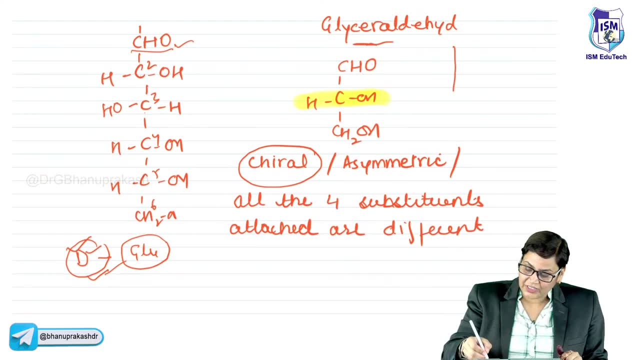 Right, They are going to form a mirror image which will be non-superimposed, Isn't it? If I make a mirror image of this, I can write it like this: Yes, very good Mirror image. Mirror image will be there, but it will be non-superimposable. 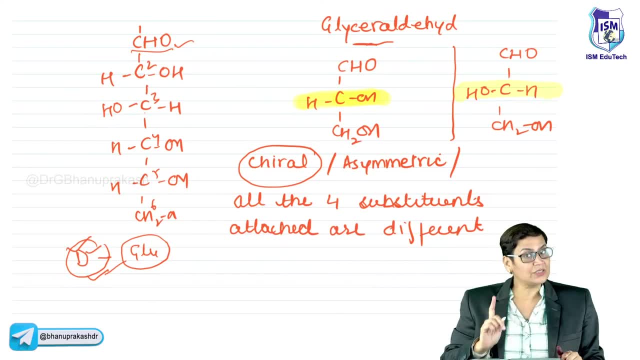 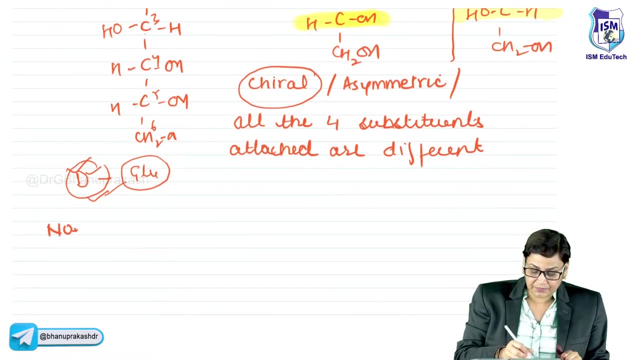 And always remember one thing: that those isomers which can form a non-superimposable mirror image, Non-superimposable mirror image, They are known as what They are known as. Yes, very good, Nagesh Enantiomers. 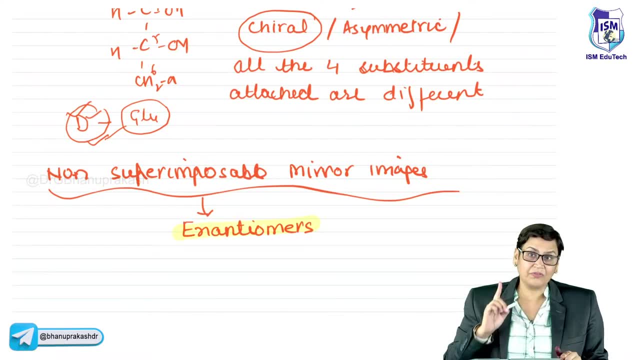 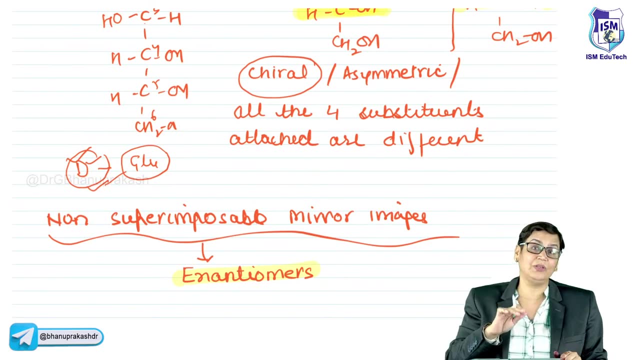 So always remember, whenever enantiomers we are talking about, first thing we have what will come into our mind. They will have a chiral carbon atom. Chiral carbon atom means all the four substituents attached will be different or they are going to form a non-superimposable mirror image. 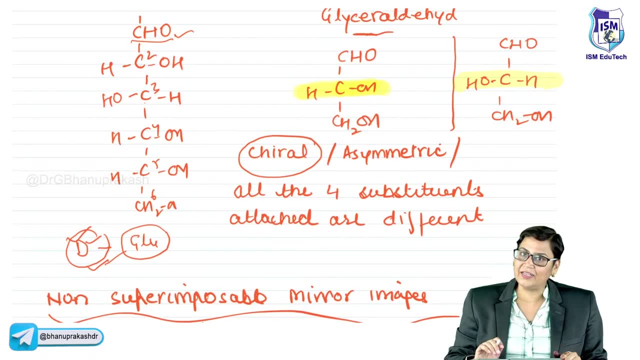 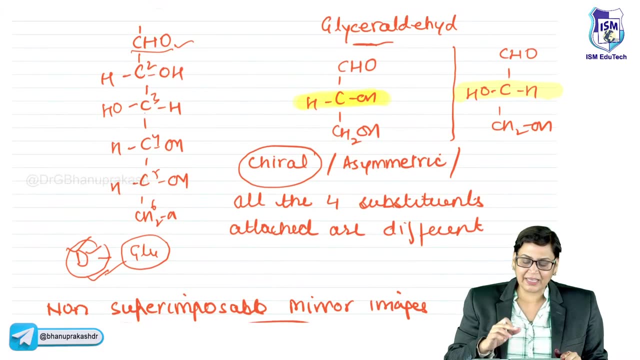 But my question was- this was okay about chirality- My question was why we call glucose as degrease. Why do we call glucose as degrease? Now see, what happens is in chemistry There is a term called Kiliani-Fisher synthesis, which means that from a three carbon atom sugar we can generate up to six or seven. 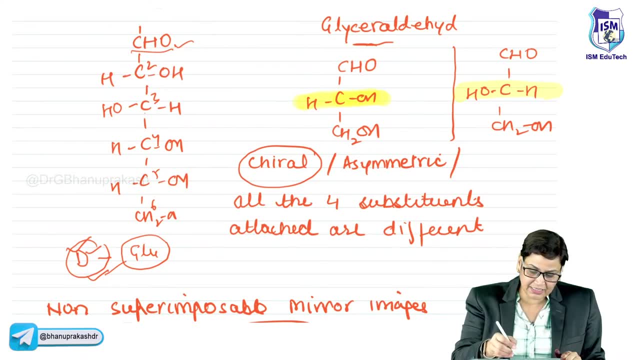 So here what we are doing is the second carbon atom. I'll just repeat it again: This second carbon atom is going to behave as a second last carbon atom in successive sugars, means, if glucose has six carbon atoms, The fifth carbon atom, which is the second last, we will stick to the position where OH group is present there. 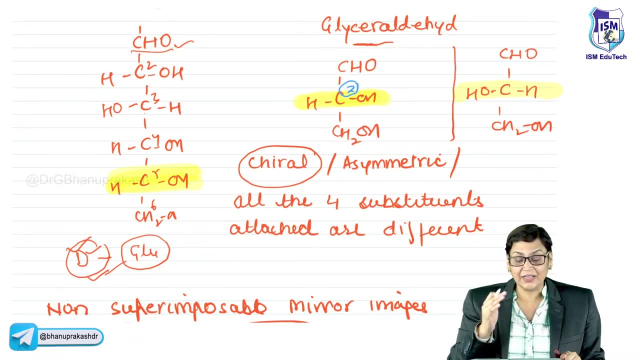 Now here you can see that OH group is present on the right hand side. Here OH group is present on the right hand side, So this form of glyceryl aldehyde is known as T-glyceryl aldehyde, and when OH group is on the left hand side, it is known as L-glyceryl aldehyde. 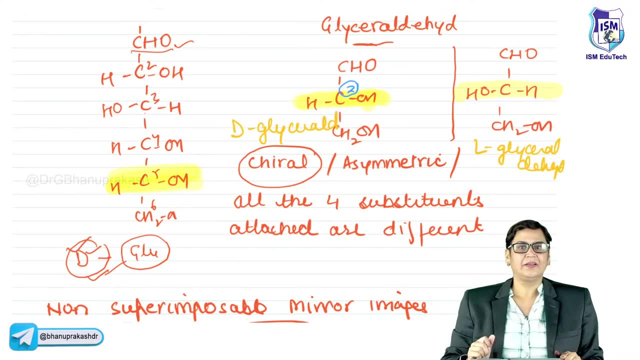 Right. So one thing is, let's just, you know, revise it. When OH group is on the right hand side in glyceryl aldehyde, we call it as capital D glyceryl aldehyde. When OH group is on the left hand side in glyceryl aldehyde, we call it as L-glyceryl aldehyde. 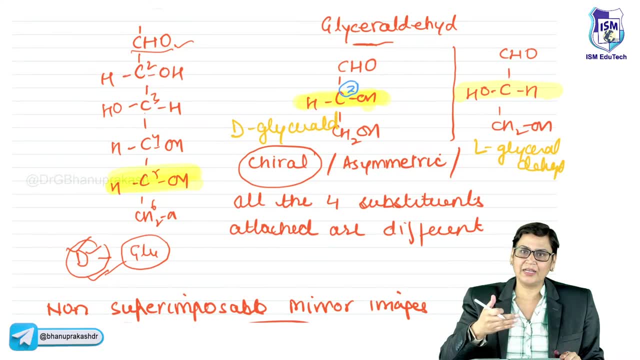 As we move to successive sugars, like three carbon atoms we are discussing four, five, six, seven and so on. the second last carbon atom will always be given press. So if we compare the structure of glyceryl aldehyde with this: 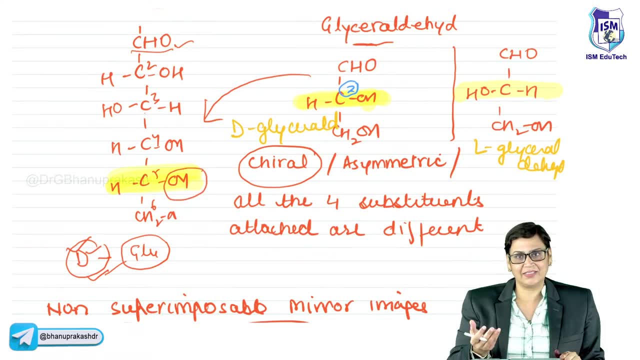 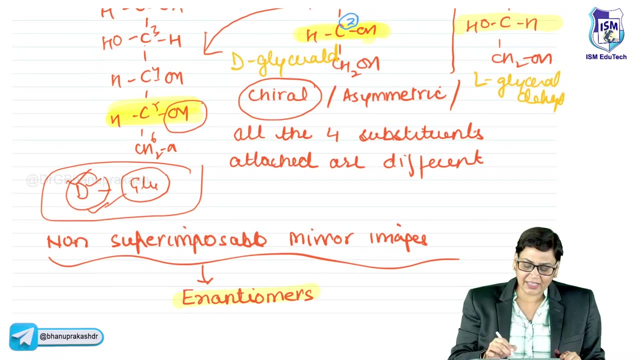 we see that OH group is on the right hand side and that is why we call glucose as D-glucose, And this is again a very interesting thing. In hospitals also, we get glucose in the form of dextrose, So always remember D for dextrose. 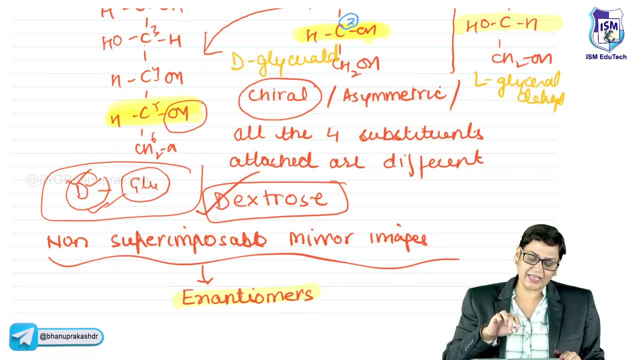 D for D-glucose. A question arises: why D-glucose? Because glucose is stable in, So we always say that it is always D. I'm not saying L-glucose does not exist. L-glucose do exist, but glucose is most stable in D form. 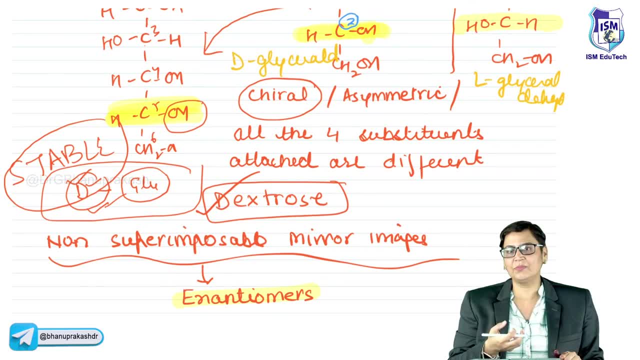 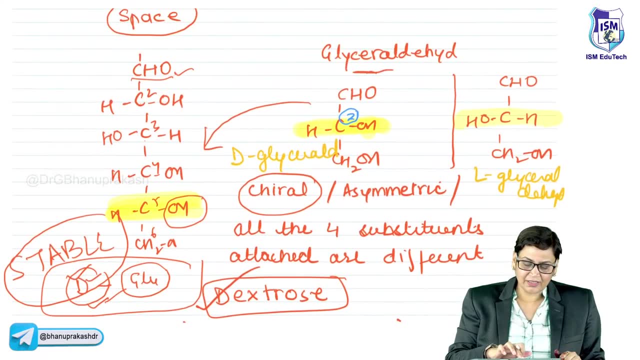 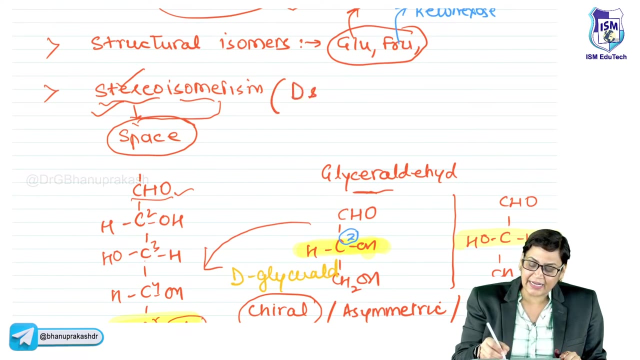 So whenever we talk about our body, everything tends to go in a stable conformation. So obviously, glucose will be stable in D form. That is why it is known as D, And these are what These are- stereoisomers. So we can say that stereoisomers made D and L are enantiomers. 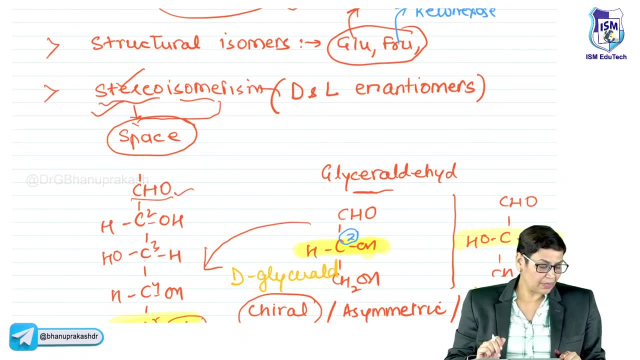 Right, Or they are stereoisomers. Now the question is a very interesting question. Let me see What's the origin of enantiomer specific chiral interactions in molecules. Let us see: Chiral carbon atom is the one just now. 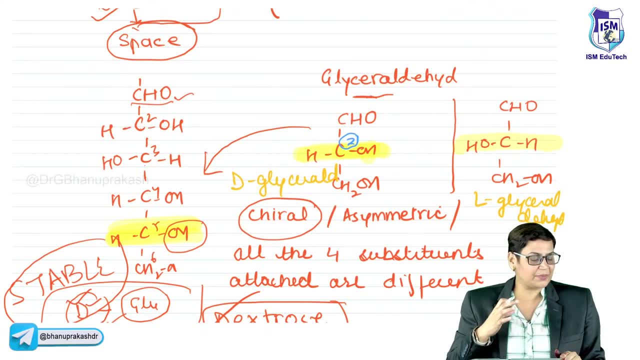 I told you, as you have studied, you must have studied in chemistry about rectus and sinistrous configuration E and Z. There are so many configurations, like whether it is right, whether it is left. So what is this all about? It is all about the. 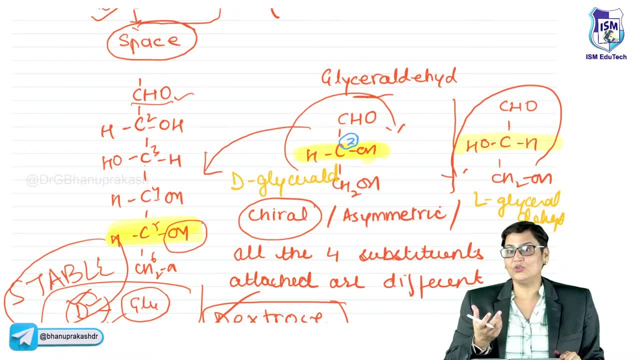 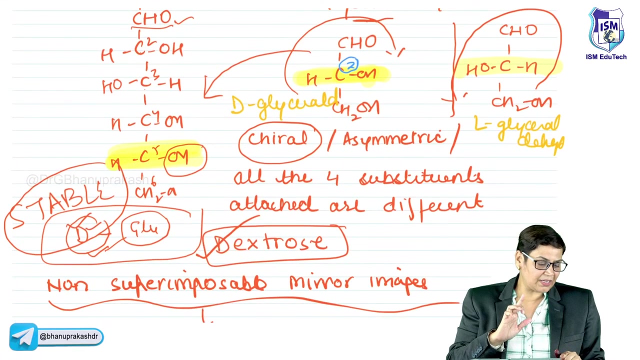 Stability. What is the stability of the molecule means in what state it can exist for a longer time. That is what is chirality all about. That is what is D and L isomers all about. Is it clear, Sanjay? Okay, So always remember one. 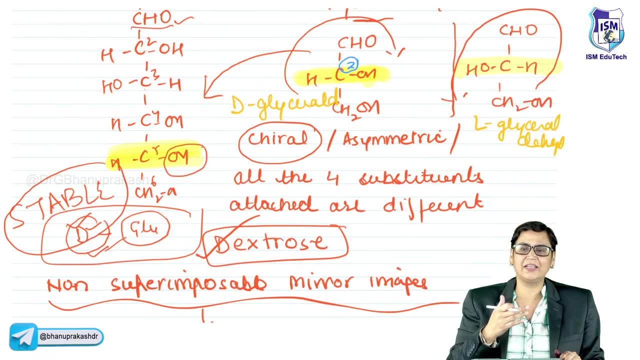 Yeah, because you know, if I talk about chemistry, you know you have studied about chair conformation Is there? board conformation Is there. this is their trance: is there to everything. times to tends to fit in a stable conformation. So whenever we talk about glucose, 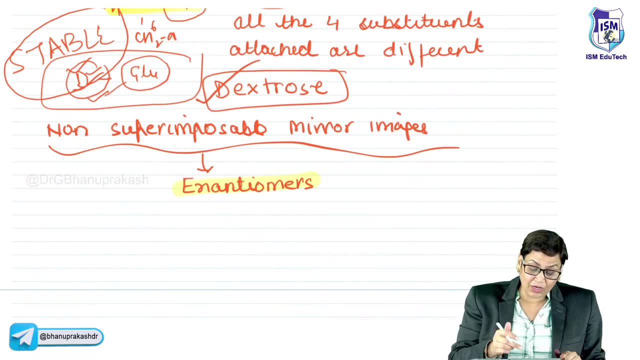 it has to be in capital D form. Similarly, if we talk about fructose, Fructose is stable in Okay. one more hint I will give you: Okay, my pleasure, The apple Mania am okay. So what we can say is: fructose is liver rotatory. 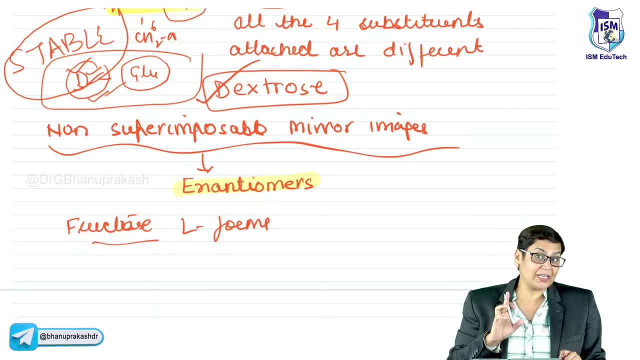 It is stable in L form. We can put it that way also, but don't get confused between small D, small L and capital D and capital L. This I just want to highlight again and again Whenever we talk about capital D and capital L. 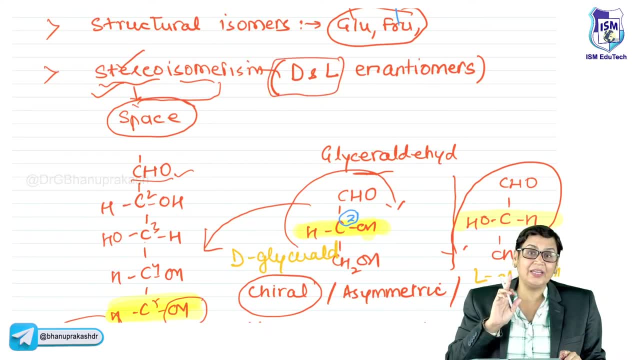 they are in response to the orientation in the space, Always remember. So we always talk about Glyceryl aldehyde as well. So it is always capital D and capital L, This same thing. You are going to My pleasure Such a big compliment. 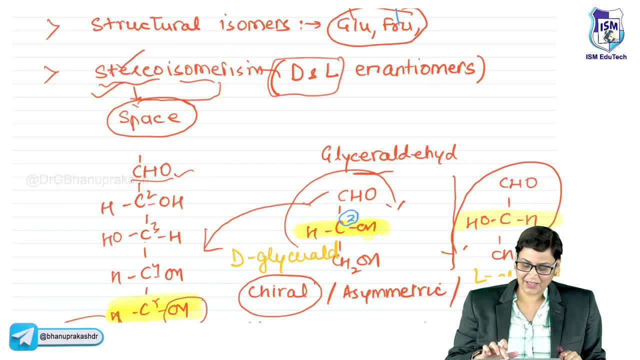 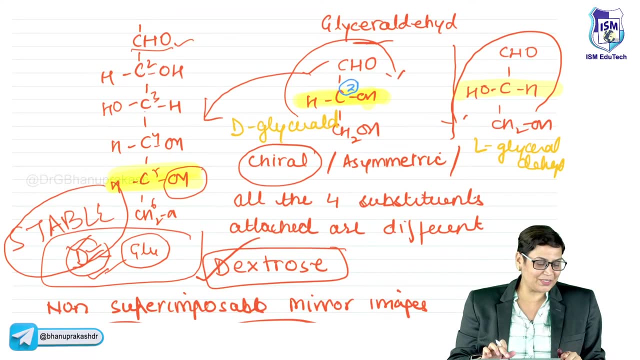 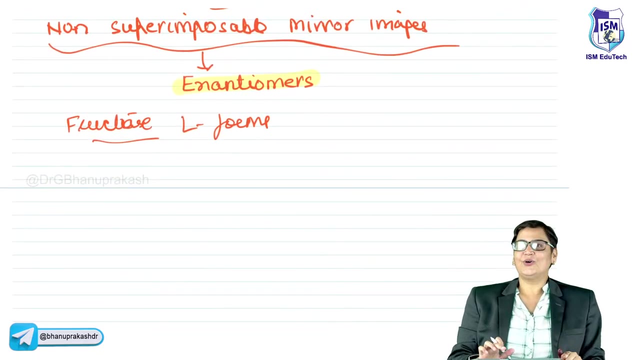 You have given me. Thank you so much. Right, So Apple Mania has given me mother of biochemistry. Thank you so much. So sweet of you. You made my day by saying this compliment. Okay, So always remember. stereo isomers in space. 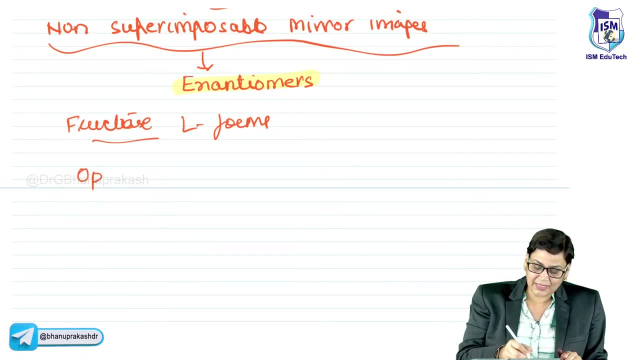 Now I'm coming to another term: optical isomer. up now. See in science, If we seen, a 99% of the problem is solved by just looking at the spelling on, by looking at the word, What the word has to say: optical, optical, something related. 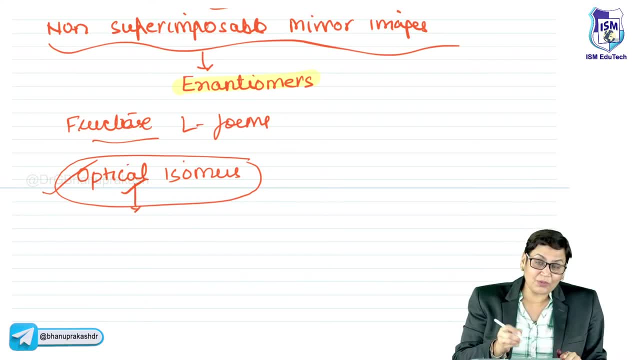 Isn't it stereo, something related to space? So optical isomer, isomers definition would be the same, but optical means in terms of optical Rotation. Right now, optical rotation, How we measure. there is an instrument which measures, it is a polarimeter. This is again a very important question. 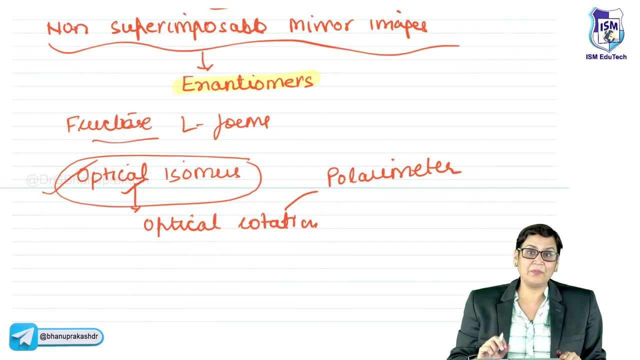 Most of the students get confused between different type of meters, especially MBBS students. Calorimeter is their, calorimeter is their polarimeter is there to see again You have to go to the spellings. calorimeter means measuring the color, because I have seen 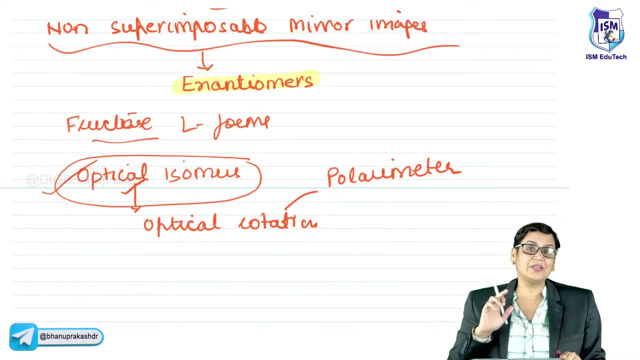 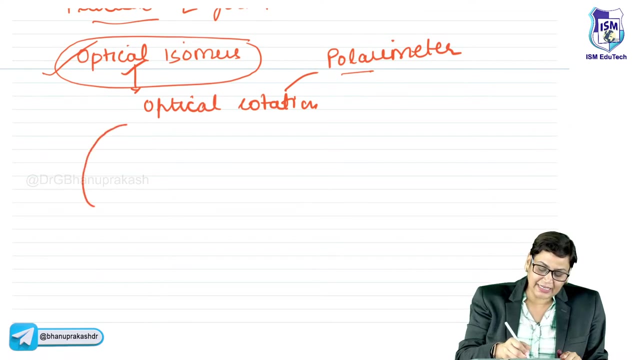 If the pronunciation is wrong, the entire thing goes wrong. Calorimeter is measurement of the calories, So there is a difference between a color and a calorie, Isn't it? So Polari means polarimeter means optical rotation, So if a molecule is rotating the plane of polarized light in a right direction, 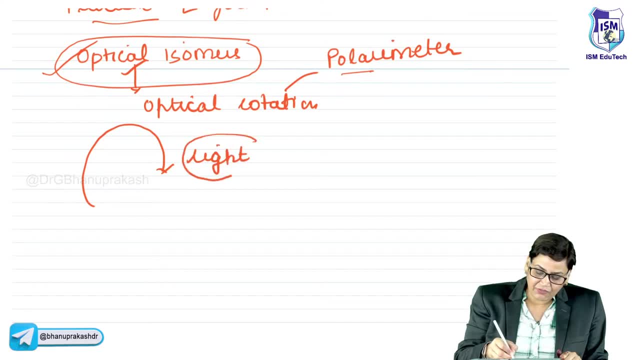 if it is rotating. I'll repeat it again: If a molecule is rotating the plane of polarized light in the right direction, we call it as dextrorotatory, Denoted by small d or plus sign Right. and if it is rotating in the left direction, again. 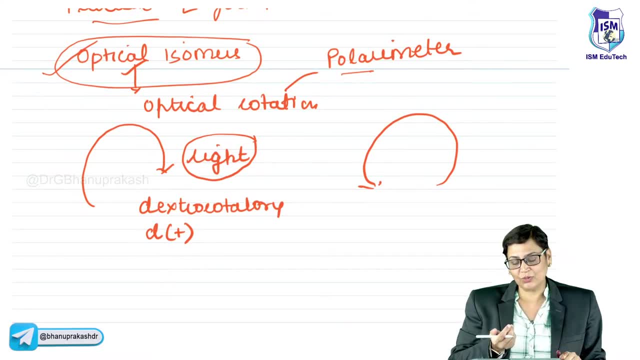 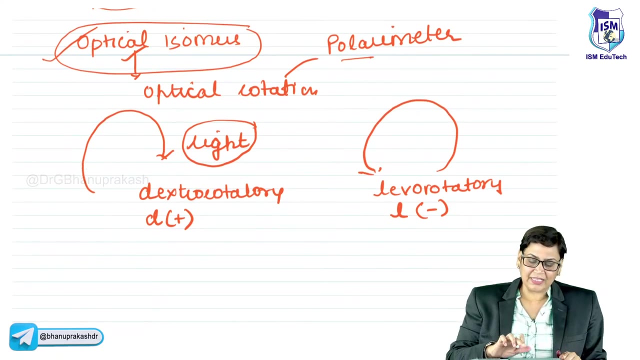 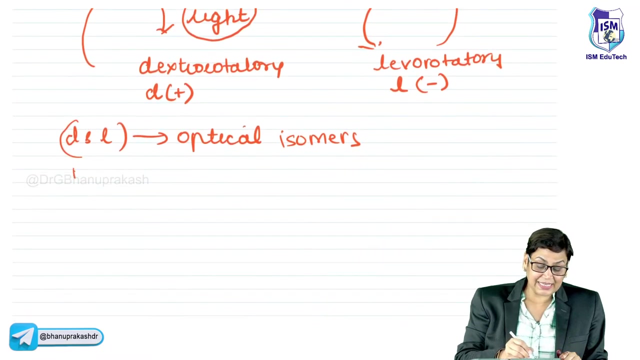 depending upon the stability of the molecules, orientation of the molecules. It is levo, Or denoted by small l, And negative Right. So these are what. so I can say D and L are what they are: optical isomers, Right, and if I talk about D and L means capital. D and L, they are stereo isomers. 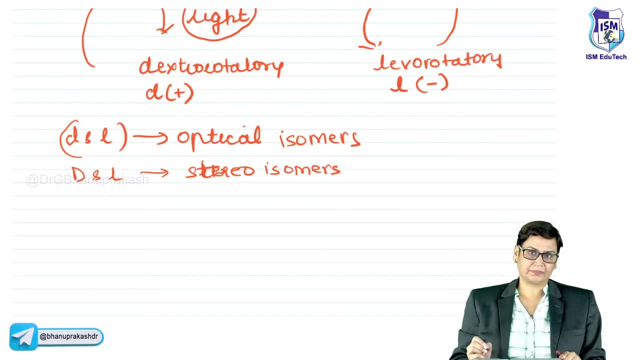 This is the basic. Now another twist is there If we mix the two. If I say mix means Now the term dextrose. Yes, Very good question. Dextrose is going to represent capital D, Because glucose is most stable. 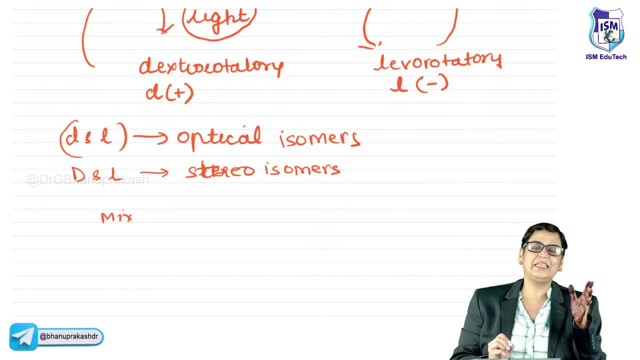 I'm telling you again and again: He means dextrose, D means capital D or D glue. Just remember it. like Right Now, if we mix the two means, what are we doing? We are making a mixture. That means D and L. 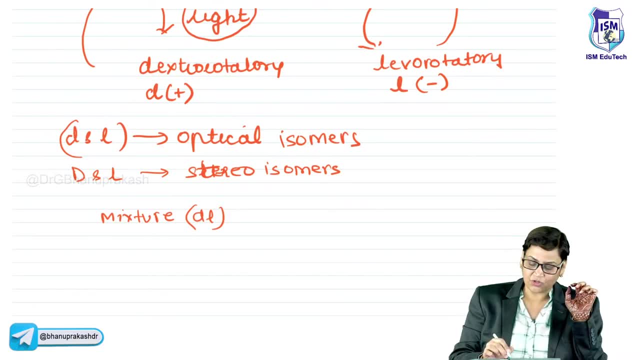 Okay. So if we talk about the optical rotation, the optical rotation means Positive will nullify the negative, So it this will be optically inactive. one thing Right. and when it is a mixture, it is known as a racemic mixture. 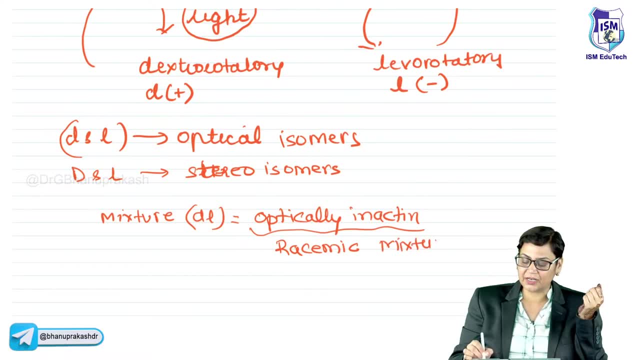 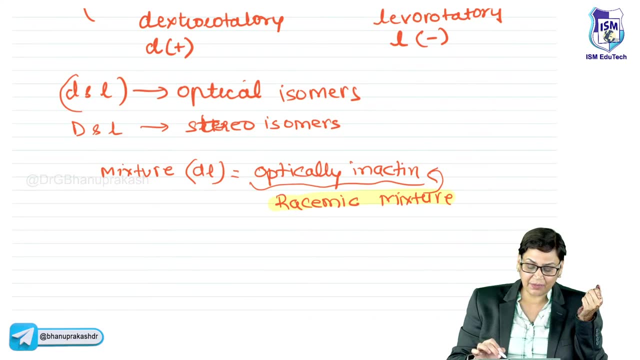 So always remember: racemic mixture is optically inactive. This is also a very, very important question. Racemic mixture is optically inactive, But if we compare small D and small L, they are optically inactive Because they are optical isomers. So they will be optically inactive. 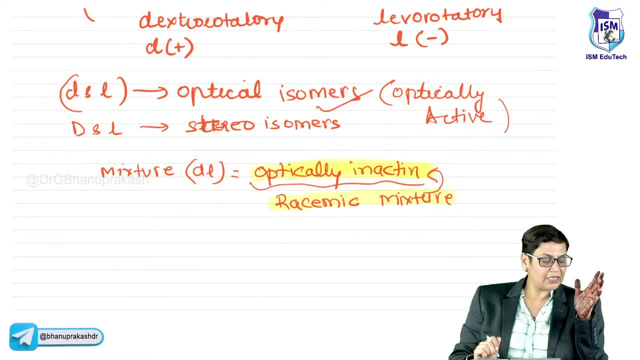 Right Now, the difference between optical isomers and stereo isomers is clear to all of you. This is very, very important Right. Optical isomers are those in which you can say they have a tendency to rotate the plane of polarize Whether it is in right direction. 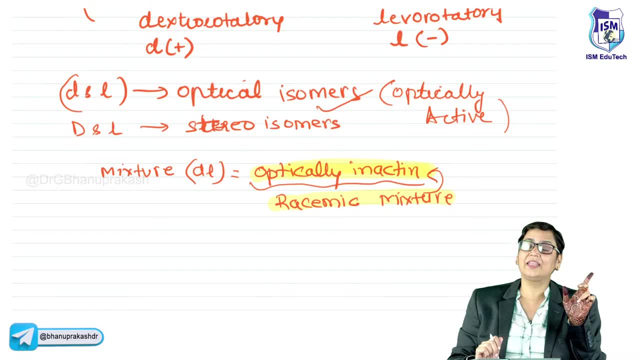 whether it is in left direction and stereo isomers are, they are always measured in terms of their position of the plane of polarize. This is the position of the OH group and I told you in successive carbohydrates Suppose, if I talk about a seven carbon atom sugar. 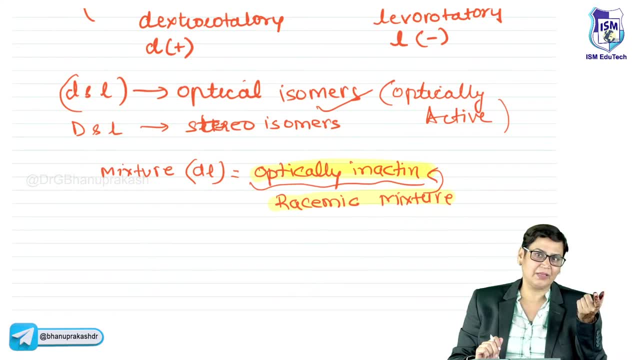 which is Cedoheptulose. you have to see the second last carbon, Wherever OH is, whether it is on the right hand side, whether it is on the left hand side. So suppose, if it comes as a image based questions, 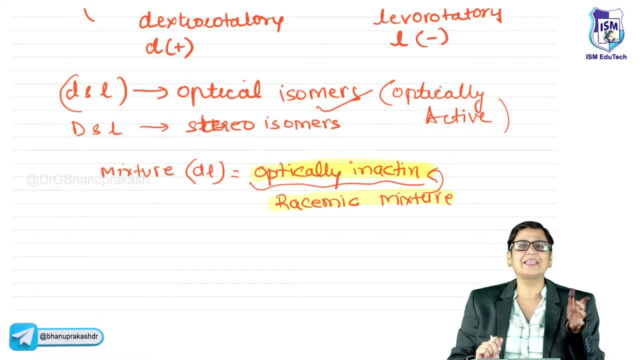 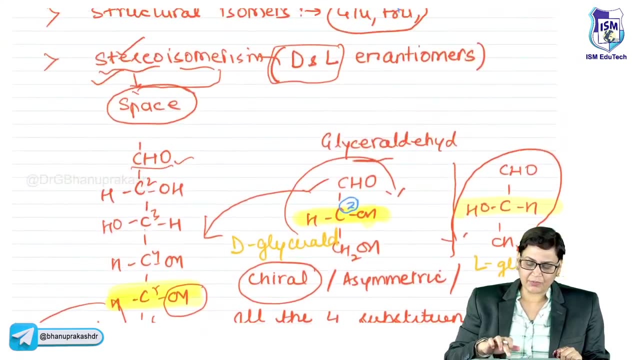 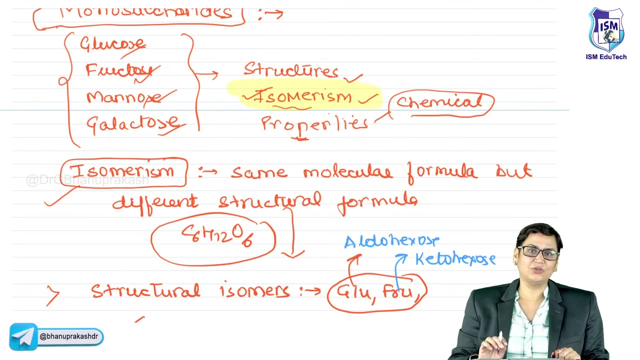 we say: chances are very bleak, So you have to always focus on the second last carbon. Okay, So this is what. this is a very important property, Property of monosaccharides, that they have a tendency of undergoing isomers, Whether it is stereo isomerism. 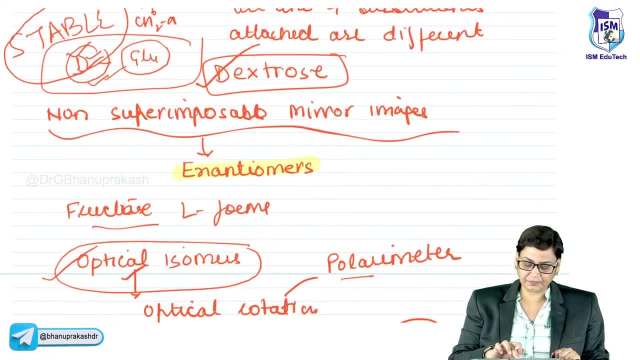 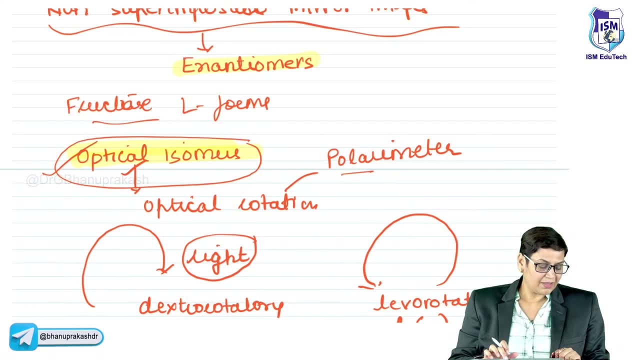 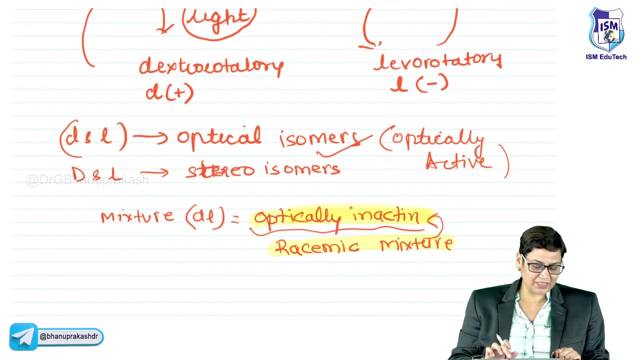 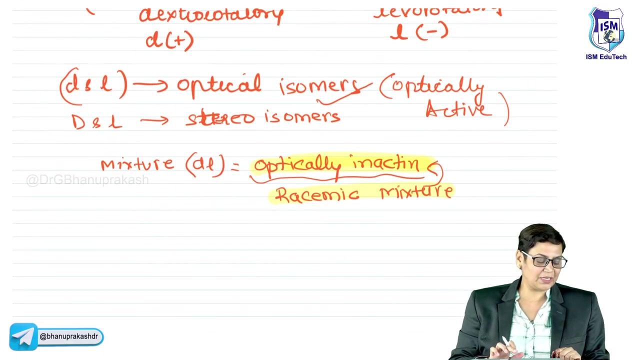 whether it is optical isomers, Because here we are mainly. Thank you so much. I am also sending love from India. Thank you so much, Dr Allah. we have just finished up with the classification and I have just discussed about the isomerism. 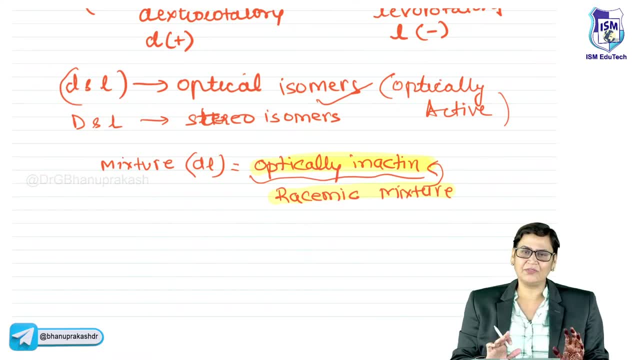 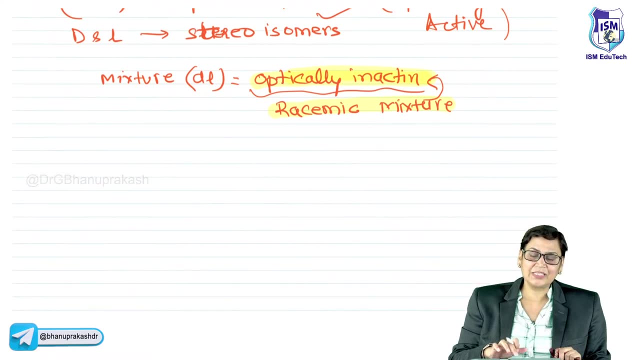 So if you have any problem, you can ask me now. Abhi, we have just started up with a very simple topic. Okay, So these are what? optical isomers and stereo isomers After this, because here mainly, we will be concentrating on the biochemical aspects. 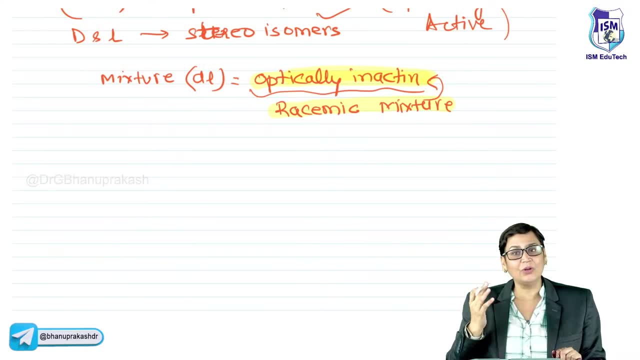 Otherwise, if we teach- if I start teaching isomerism, it will take whole night. you know it won't finish also, but here we have to only stick to that. isomers, Which are, play a very, very important role in our body. 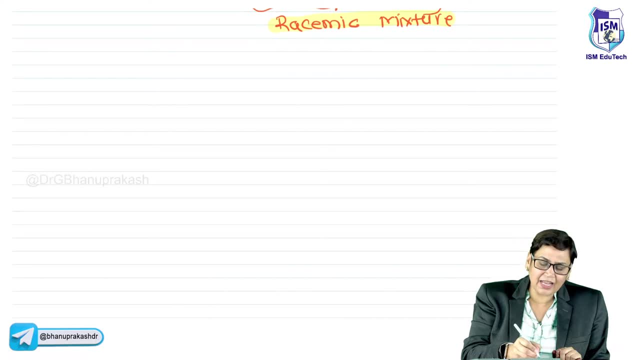 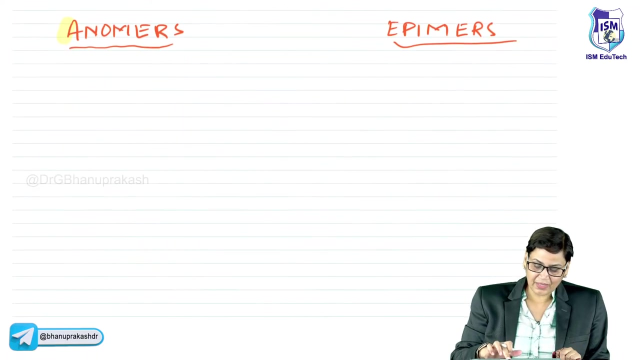 Right Then, moving on after this, there are two very, very important terms. One is anomers And second is epimer. Right Up now, What are anomers? What Anomers are defined As- yes, very good, anomers. 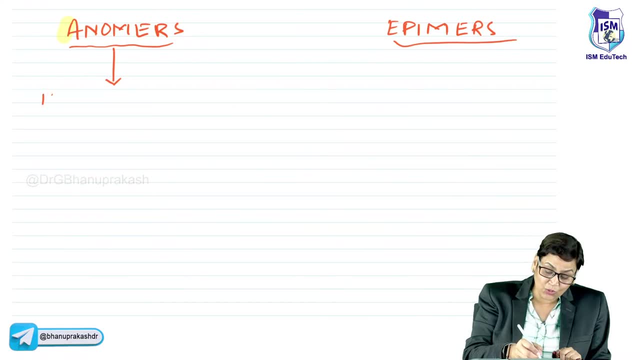 Very good, Nagesh. anomers are defined as those isomers. Now see how we differentiate isomers, which differ only at C1, which is bearing the functional group. So how do we define Anomers? Anomers are defined as those isomers. 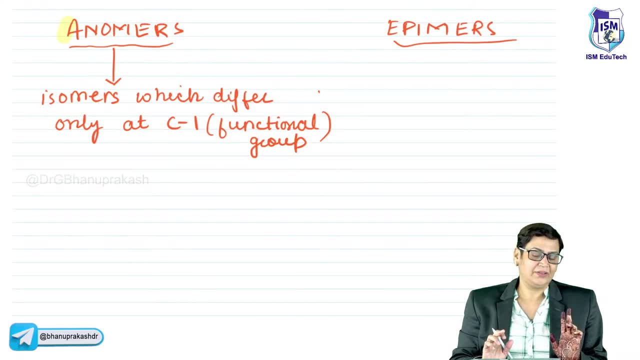 which will be differing only at carbon-1.. Right And carbon-1, by chance, it represents the functional group. Okay, So now what happens is: and if we take the definition of epimer? Yes, Dr Allah, this is whatever I'm teaching you in biochemistry. 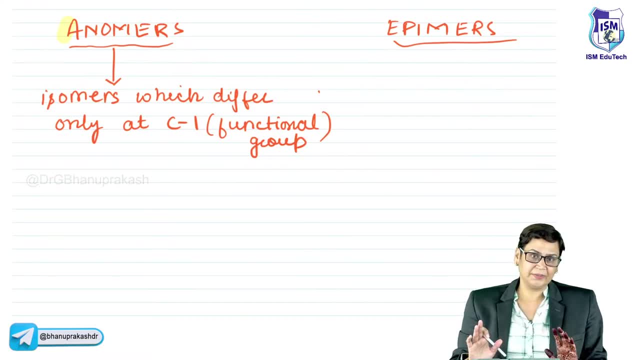 This will be more than enough for a first-year MBBS student. This I can give you in guarantee, Because I am focusing on each and every minor topic. Obviously, major topics, though, I will be touching up, but minor topics also, I am discussing in the classes. 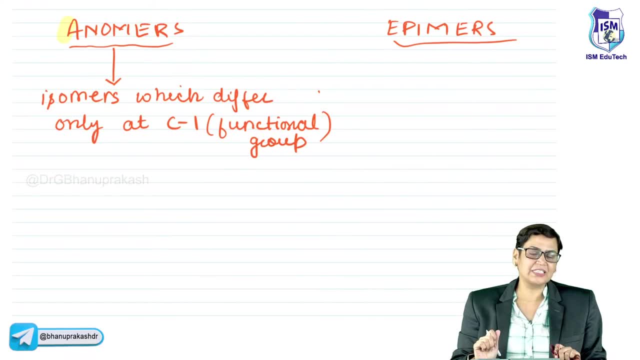 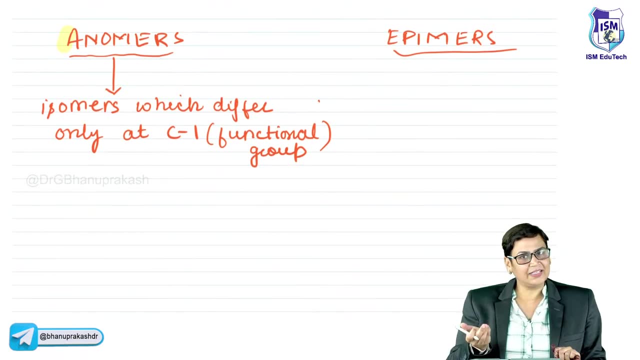 So you can tell your other friends also to attend the classes. These classes will be very, very beneficial for all of you. Okay, So anomers differing at C1 epimer are the isomers which differ At any other position, At any other position. 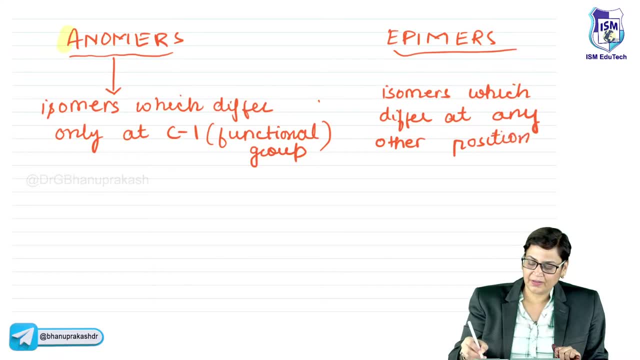 Except C1.. To see how interesting it is, If they are differing at C1 position they will be known as anomers. Now if they are differing at any other position, be it C2,, be it C3,, C4,, 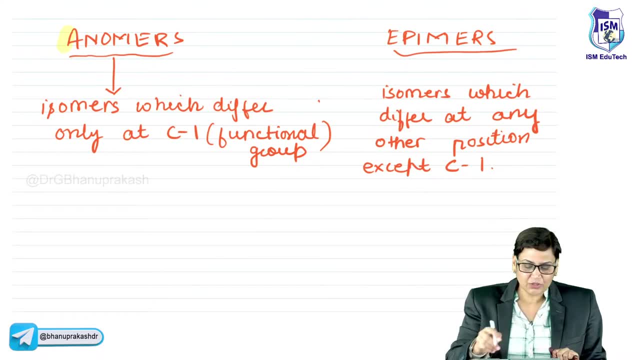 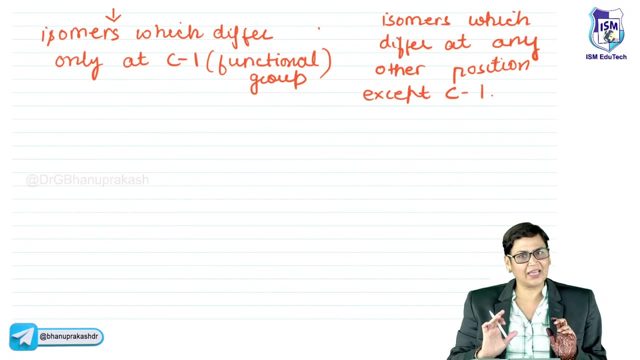 C5, they will be known as epimer. Okay, So this is the basic difference. Now I'll just give you a you know little bit knowledge about the structures, Because, again I am telling you, don't focus on the structures more. 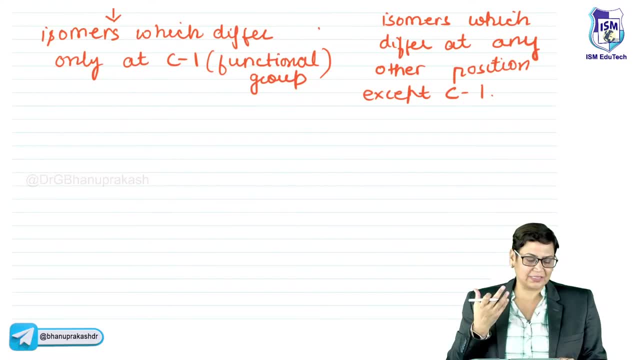 but little bit knowledge you should have, Because starting- say this, is your, just you know- beginning of the career. You people have already studied chemistry in your class 11th and 12th. So if you make a chemistry base for biochemistry, 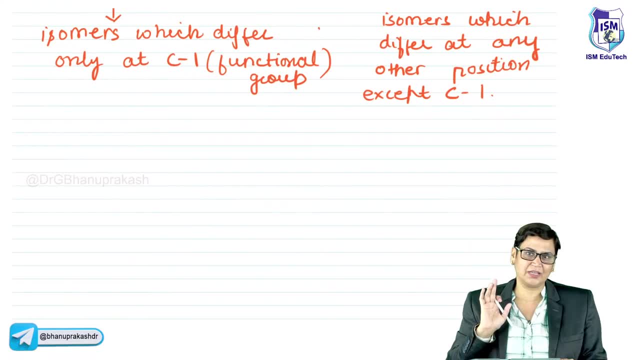 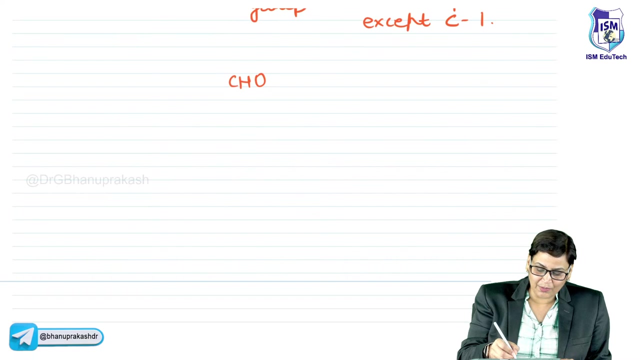 you won't find any problem in understanding the subject And obviously you will be focused to what is happening inside the body, So it is more more interesting, Okay, So first of all, if I talk about now, see, all of you know about this. 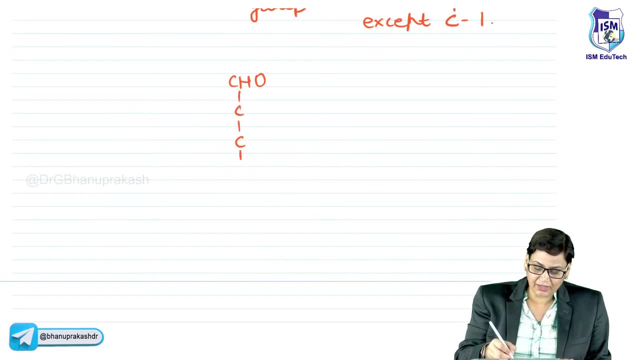 I'll just write the structure of glucose again: 1,, 2,, 3,, 4,, 5, and 6.. Okay, OH At third position. always remember OH is here. H HOH, HOF. 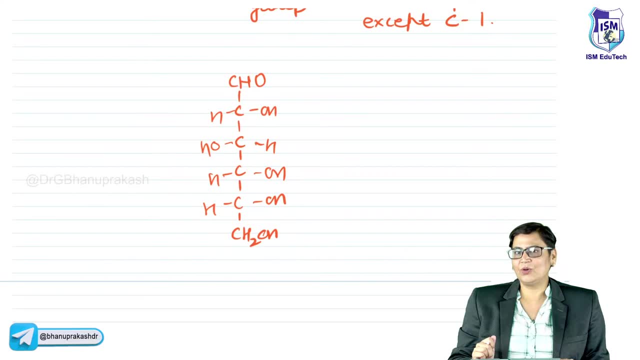 Okay, Now see, you must have studied about acetyls, ketones, Isn't it? What is the basic difference between an aldehyde and a keto? So many things you have studied in your, you know, maybe in 11th or 12th. 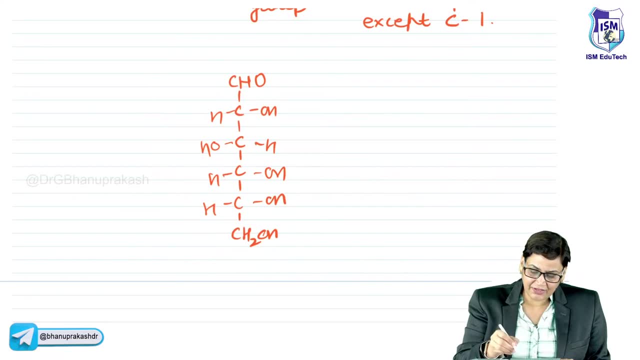 Now, if this aldehyde is there, I can write this aldehyde Like this: CH double bond O. Similarly, I can write it like this: I can write it like this also: Rest. I won't repeat, It is but obvious. 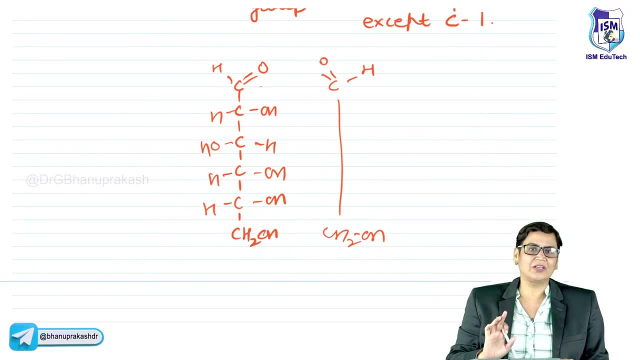 Right, This is what this is known as a open chain structure of glucose. Now, just now I told you everything tries to go in a stable conformation. So what is happening is there is a reaction between the first carbon atom and the fifth carbon atom. 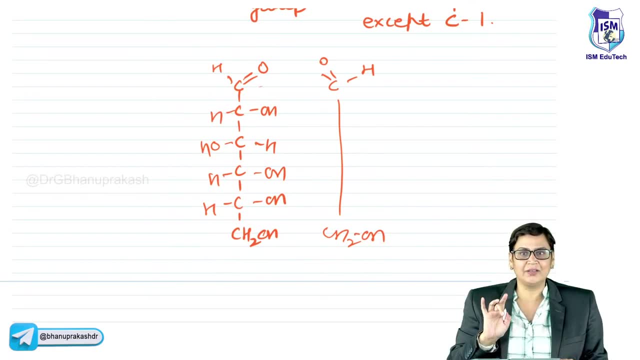 So reaction means loss of a molecule of water which we know, we, which we call as, as condensation also. So I can say that reaction can be between first and fifth from this side and reaction can be this side. 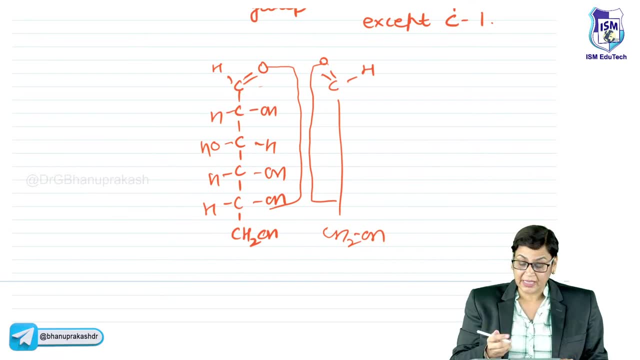 Isn't it Wherever double bond O is there, because water is what H2O. So if the reaction is like this, or if I say loss of water molecule is from here, I can say that it will have this type of structure. 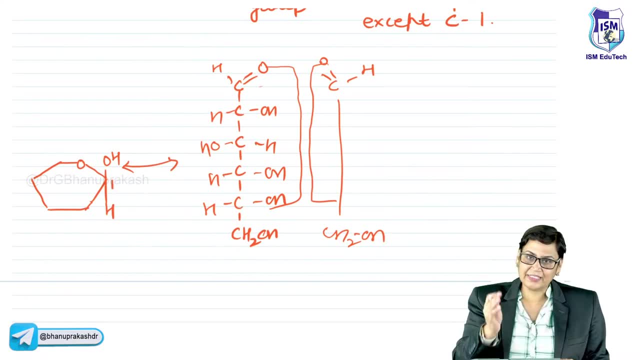 This will be the first carbon atom. If I say it is like this, it will be like this: Right, Rest. everything will remain the same. So this will behave as the first carbon atom. This will behave as the second carbon atom. 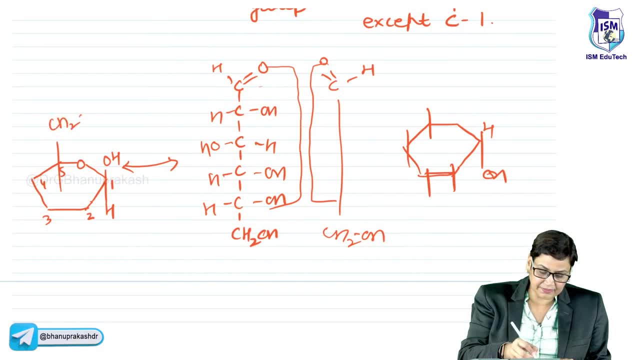 third, fourth, fifth and HH. See Sanjay beta. there is no confusion. Just remember one thing: hemiacetyls and acetyls. Hemi means partial acetyls, acetyls means full acetyl. So 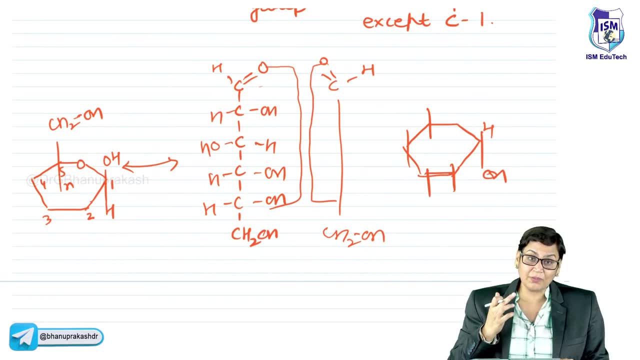 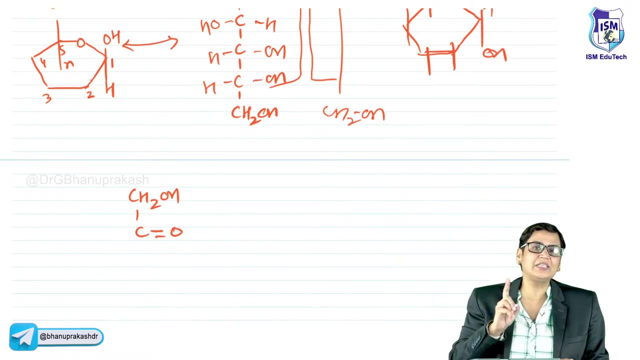 that depends on the functional group, how the reaction is taking place. Because, if you remember, if I talk about a ketonic group, ketonic group is always placed like this, If you remember, because ketone is never given first position, carbonyl carbon is having second group. 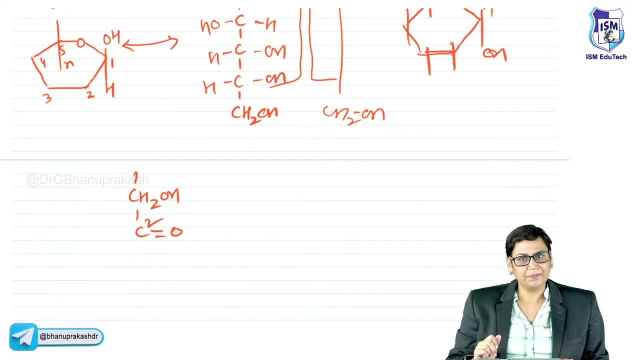 So, depending upon that, acetyls and ketones are produced, but that is not a part of biochemistry, So we won't be touching that aspect, Otherwise you people will get confused. Okay, just remember one thing, See, 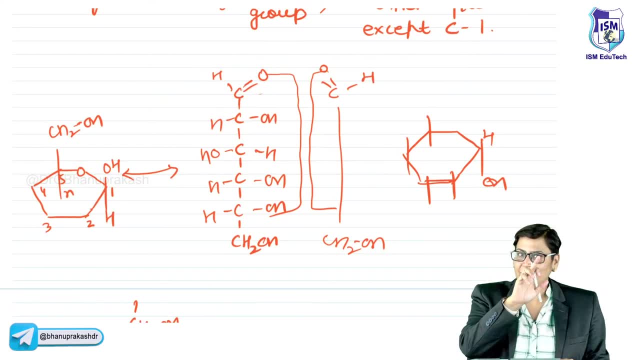 there is lactam ring formation. Okay, so it will be like either from this side or this side, So change will be only at first position. Rest: everything will be same. I'll just write it once. I'm just writing it. 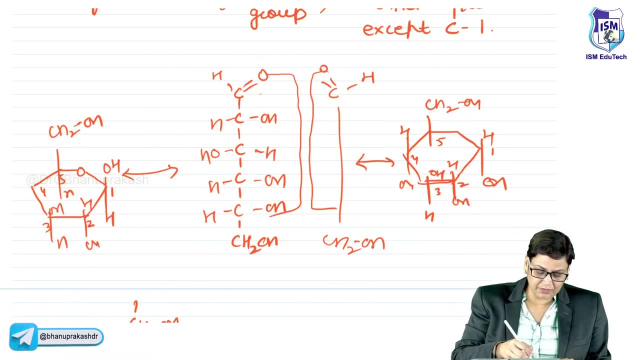 Hello, I'll write it Here also. but even if you know, try to make these structures at home. It's very easy. No complexity is there? What I'm trying to tell you here is: this is a resonance, basically resonating structure. 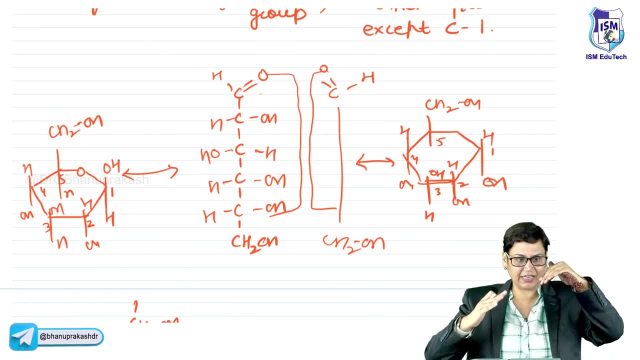 Double bond O is present here. Double bond O is present here. If the reaction is like this, this will result. If the reaction is like this, this will result. or, in a simplest language, the change will be only at carbon one. You can see if I talk about this carbon one. 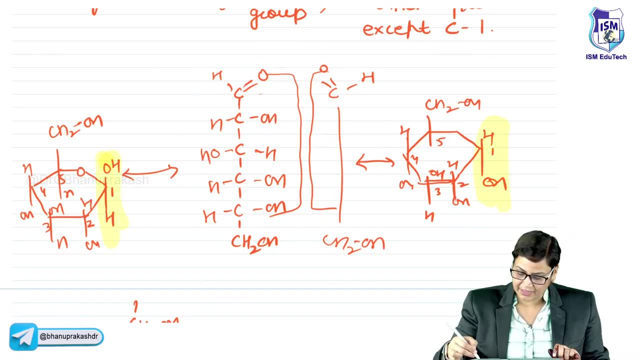 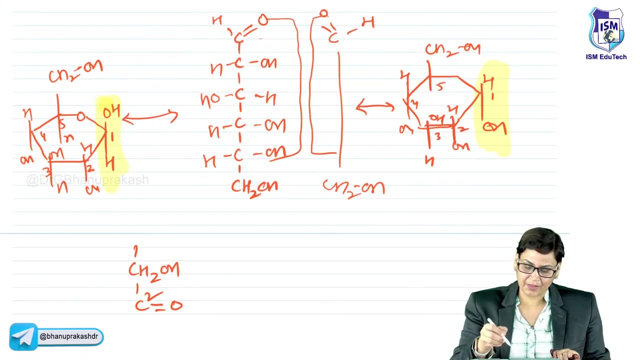 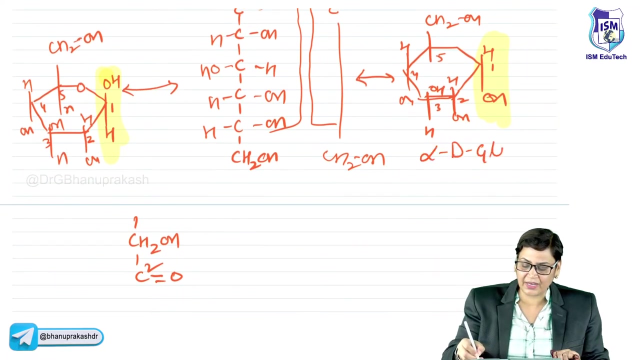 you can see that The difference is only at the OH position, Isn't it Now see? if OH group is below or if OH group is placed downwards, we call it as alpha, Very, very important- And if OH group is placed upwards, 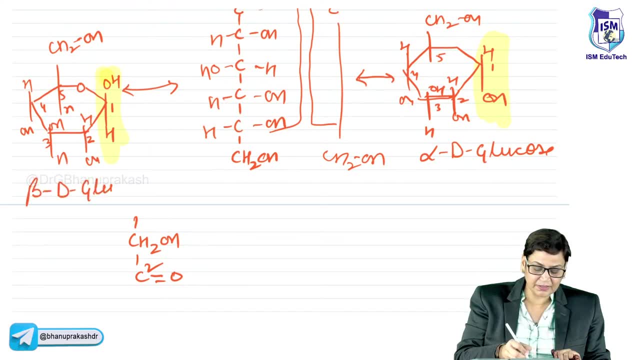 we call it as beta Two cores. So now you tell me the change is at which carbon atom. If I talk about alpha and beta, by just looking at the structure can you identify the change? The change is taking place at which carbon atom? 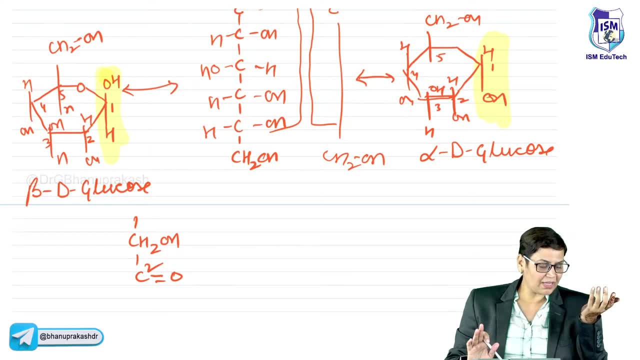 One, two, three, four, five, six. Yes, very good, Nagesh, Send one, isn't it, Sanjay Sagar? First position for change? Hey, first carbon atom. If you look at the right hand side. 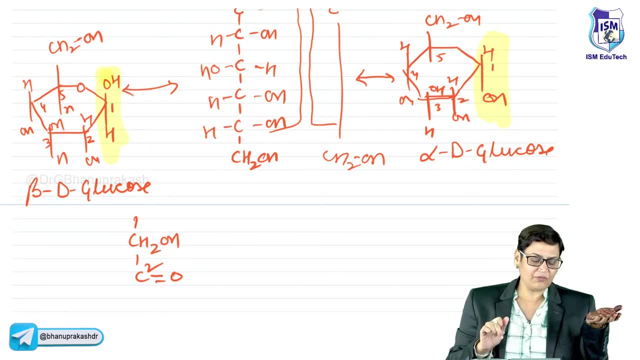 OH group is placed downwards, I call it as alpha D glucose. If OH group is placed upwards, it is beta D glucose. Now, coming over to this, this I will say it is a open chain form of glucose. So can I say that open chain can be converted into alpha glucose. 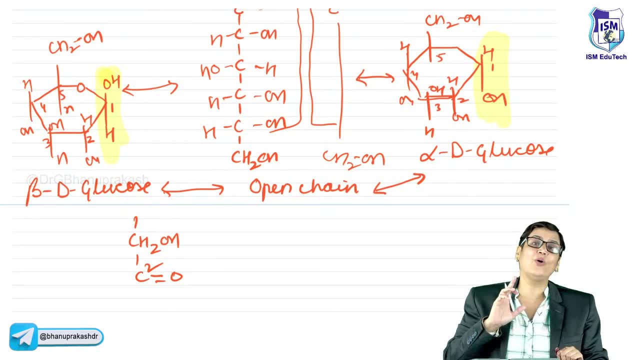 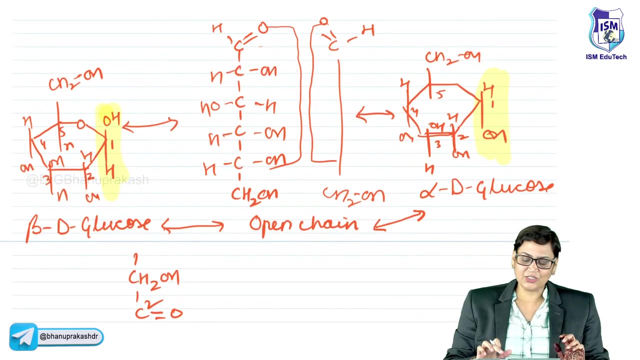 Open chain can be converted into beta glucose, or all the three forms are interconvertible with respect to one another, Yes or no? So this is the very simple concept. It is very simple, See, there is nothing in it. The reaction is taking place only at the first carbon atom. 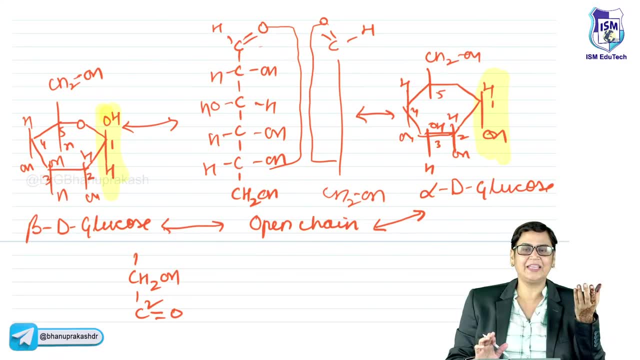 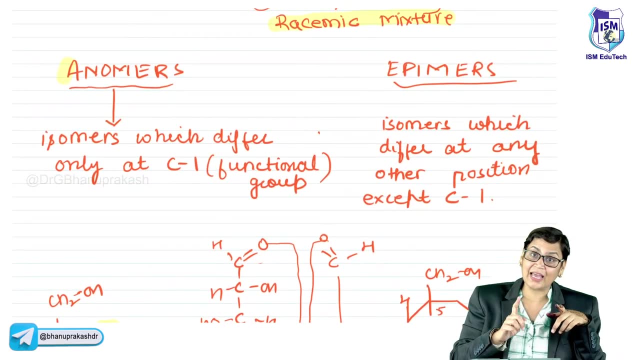 That is what I told you. no anomers, anomers. what are anomers? Anomers are the isomers which are differing only at C1. and what is C1?? C1 is representing the functional group. It is not the reaction. 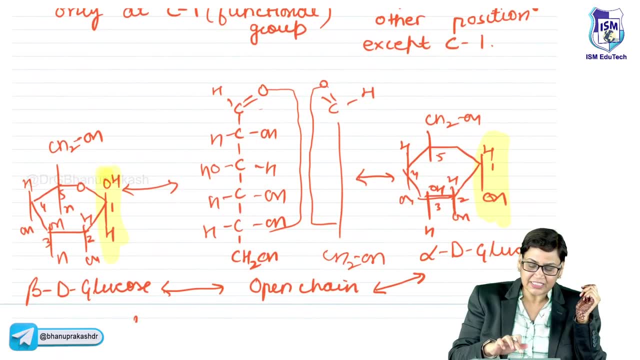 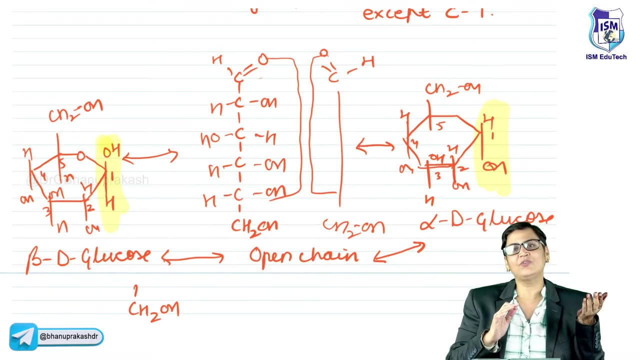 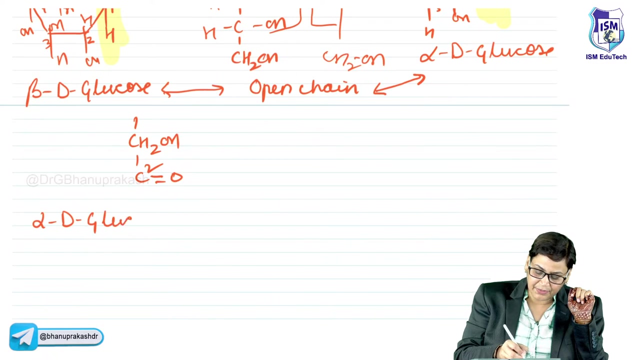 C1 is not a reaction, C1 is a function. So C1 is the reaction. That is the reaction, the functional group. Now, in this functional group, if water molecule is lost from the right hand side, or if the water molecule is lost from the left hand side, it will result into either alpha D-glucose or beta D-glucose. So my point here is that alpha D-glucose and beta D-glucose are differing only at C1, so they are known as anomes. 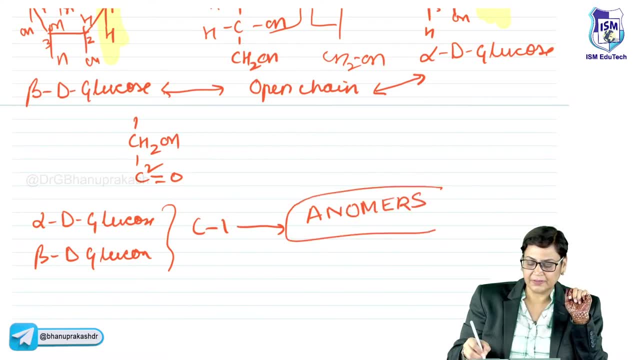 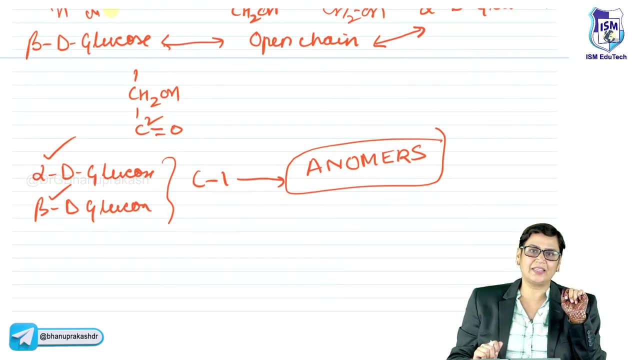 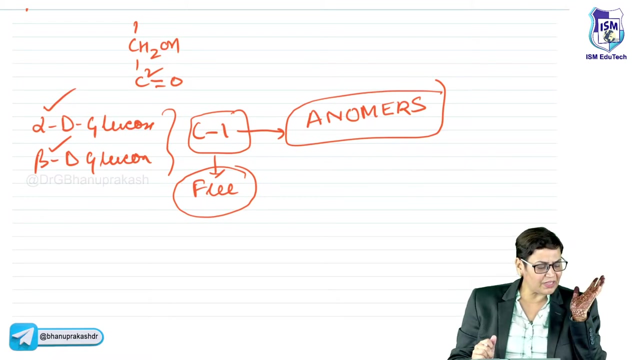 Now you tell me if anomes are there, whether this C1 is free or not. Free means whether it is free to react with something or not, Yes or no. I want an answer from you people. Don't hesitate. whatever is there in your mind, just speak up. I just want to see how much you are understanding. 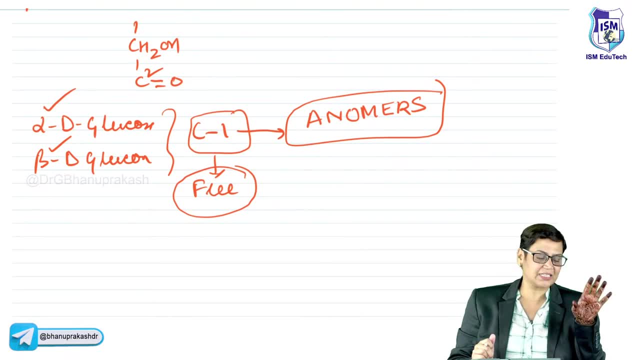 My question is- I will just repeat the question. My question is: just now I told you, anomers are the isomers which are differing only at C1 position. C1 is the functional group. Now my question is whether this C1 is free or not, Whether the functional group is free or not. 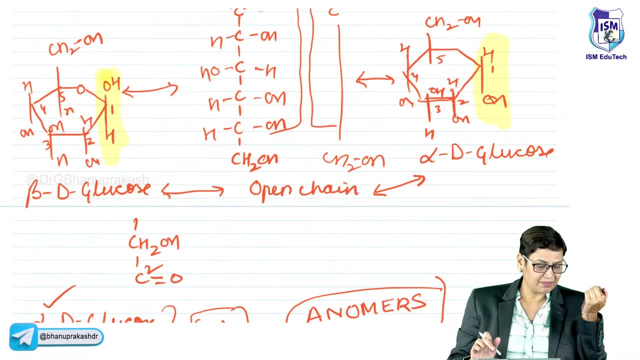 You can see the structures also. Looking at the structure, can you tell me whether it is free? Very good, Nagesh has said yes. Sagar, Sanjay, Dr Allah, Say something. whatever is there in your mind, just speak up. That is what is the advantage of a live session. 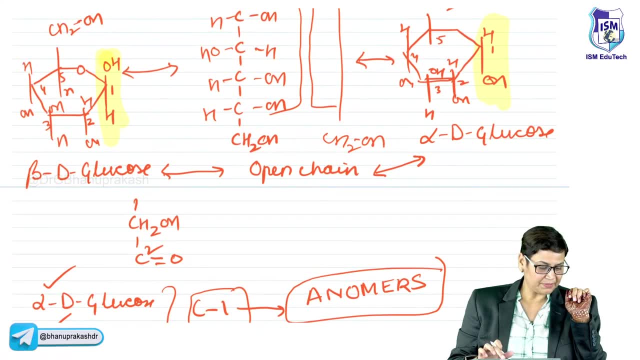 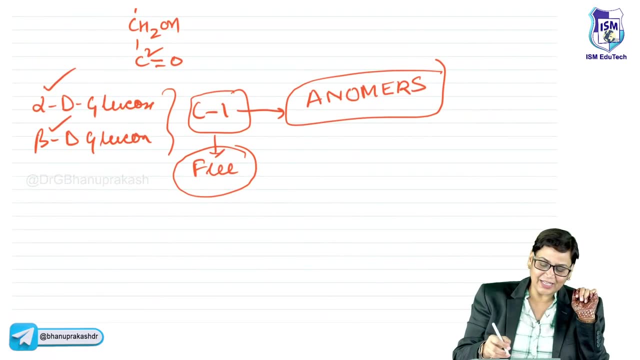 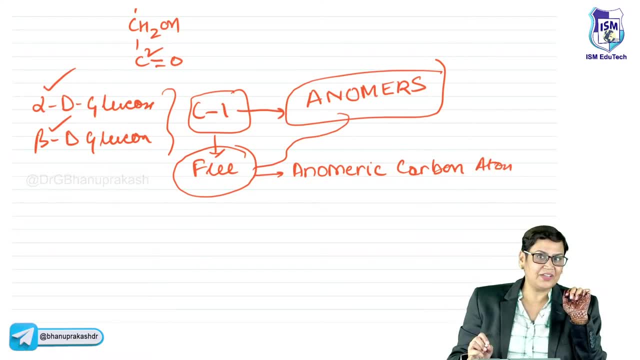 And those sugars which have a free anomeric carbon atom. concern about the canose ficar And those sugars which have a free anomeric carbon atom. concern about the canose fireplace illea more, No, no, What are you talking about? 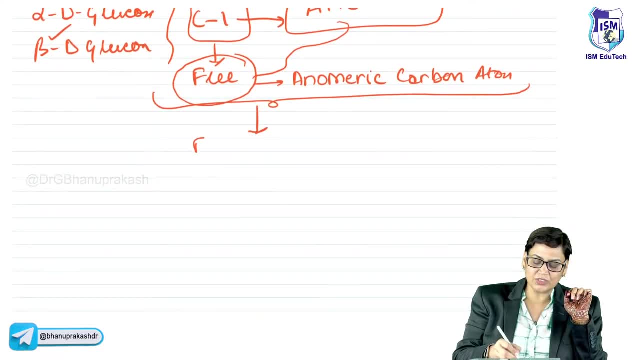 atom. they are known as a reducing very, very up the co from isomerism. we started with isomerism only and we have come to reducing, because now I'll tell you what is the significance of these reducing sugars. you know, reducing sugars kick a significance in my body. may these are. 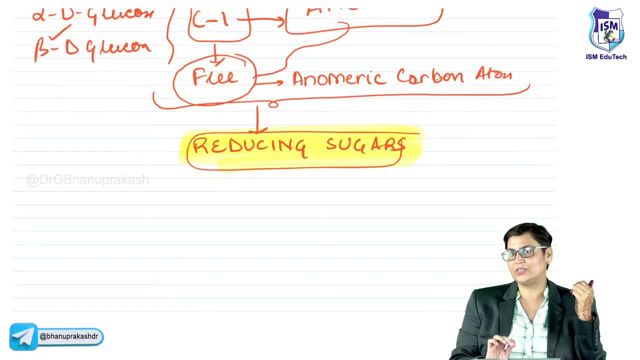 one of the very, very important abnormal constituents of urine. if we reducing, sugars appear in urine is a clear indication of glycosuria, which can lead to diabetes mellitus, which is very, very prevalent nowadays. so you can see how chemistry mixes up with by chemistry. so isn't it interesting, right? so, anomers? 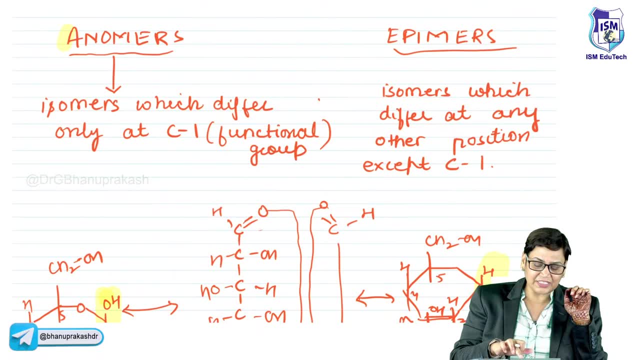 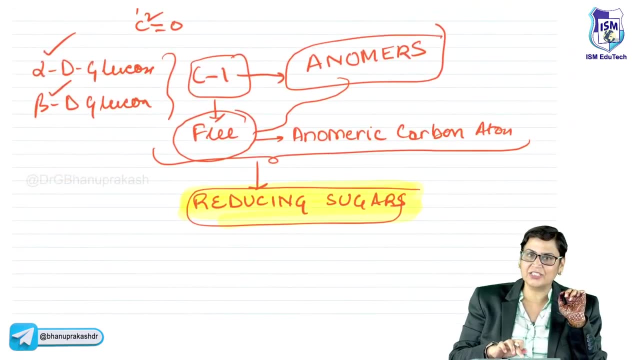 kya hai? anomers are simply the isomers which are differing only at- just remember, okay, and then they have a free functional group. and those isomers which have a free functional group, they are first of all known as anomers and secondly, they are known as reducing. 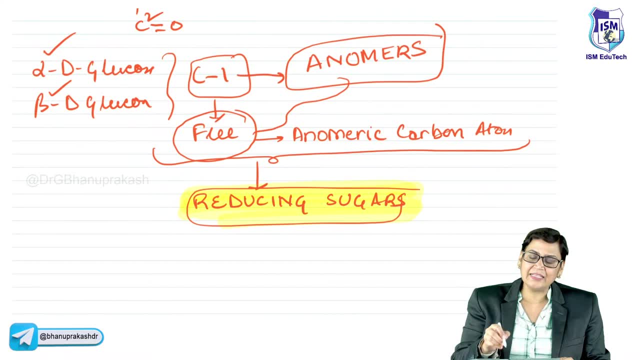 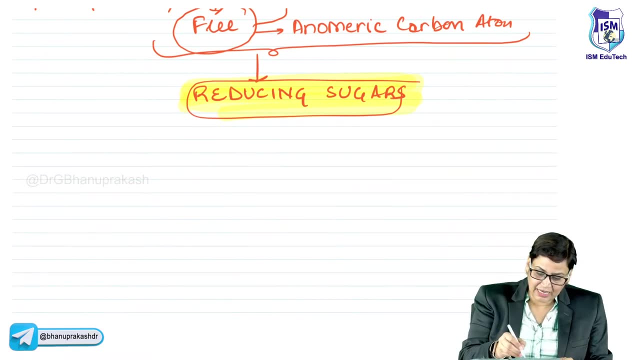 sugar. so alpha and beta are linked as anomers. then coming over to epimers, now again there is a confusion. I'll just try to sort out that confusion. epimers definition: I told you that they will differ at any other position except c1, even if I differ, carrying it away no. 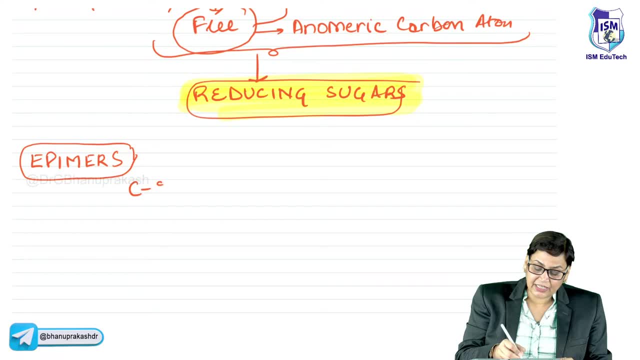 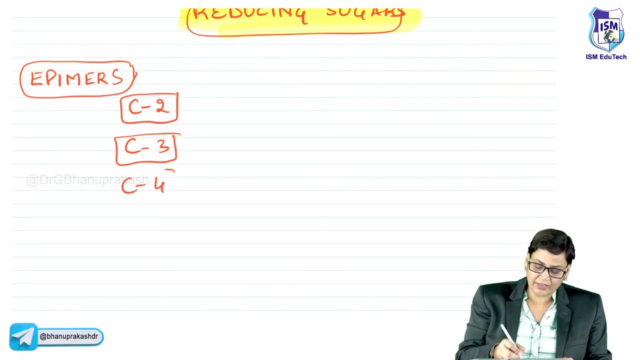 more saying gay, okay, if they are differing at c2, they will be epimers. if they are differing at c3, again, they will be epimers. c4, c5. now what are the examples of these? if I talk about c2, yes, very good, galactose is. 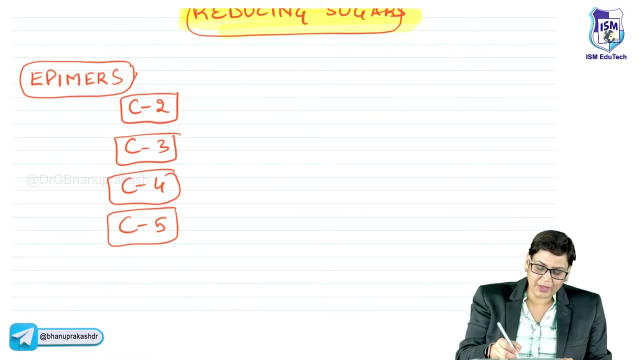 yeah, I am coming to that. yes, yes, c2 may also always remember. mannose is a c2 epimer of. can anybody tell me c3 aloes? very good, Nagesh aloes, again c3 epimer of glucose. c4, galactose, C5, let C 5. can anybody tell me c5? 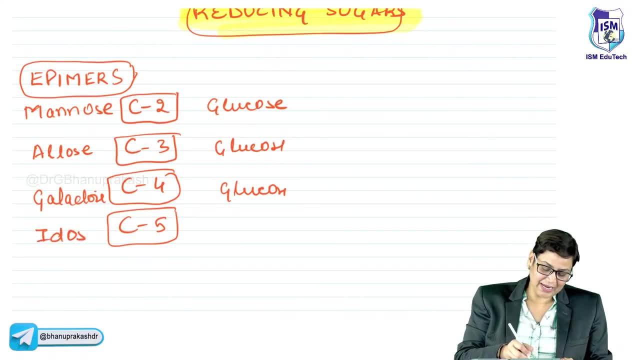 okay, I'll tell you I dose. I dose is a c5 epimer of glucose and you know the all these reactions. okay, all these reactions takes place in the liver, this galactose is converted liver and if the enzyme which is risk, see if in our body the reaction is. 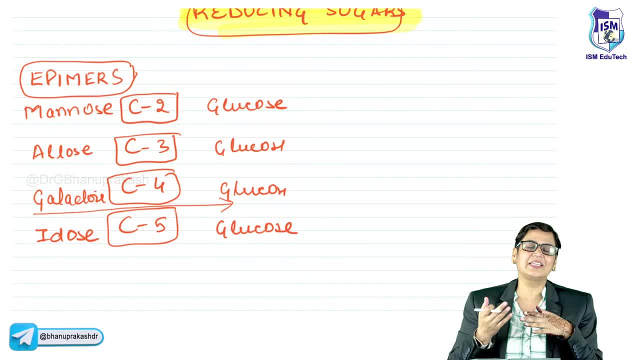 taking place is a chemistry, memca both. a catalyst is the one which is increasing the rate of a reaction in our body. the work is taken over by the enzyme, and if that particular enzyme is absent in the body, it will lead to diseases. and same thing happens if galactose is not converted to glucose. what will happen? it? 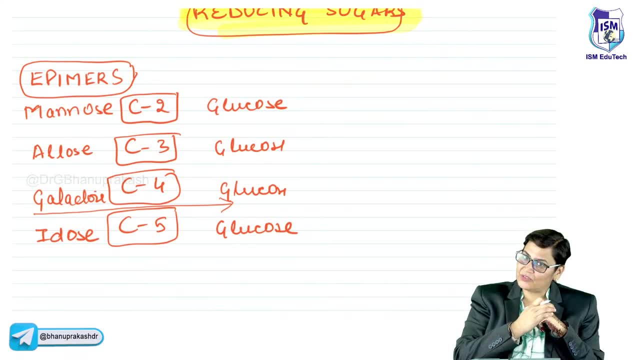 will lead to a very serious disorder, which is galactosemia, which we will be again studying in detail in the matter. right, so these are what you can see: simple: C2, C3, C4, C5, not on C1 up. now tell me these epimers, can they be reducing? 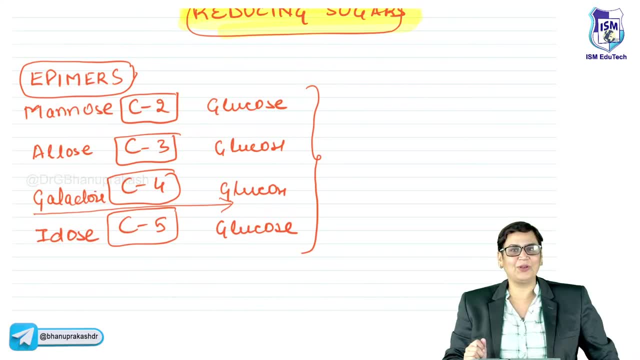 sugars, yes or no? let me see how much chemistry you people. my question is: anomers, though you know C1, differ that also. you know anomers which have a free- functional- yeah, you can say- which have C1 one free. they are known as reducing sugars. my question is: can epimers behave? 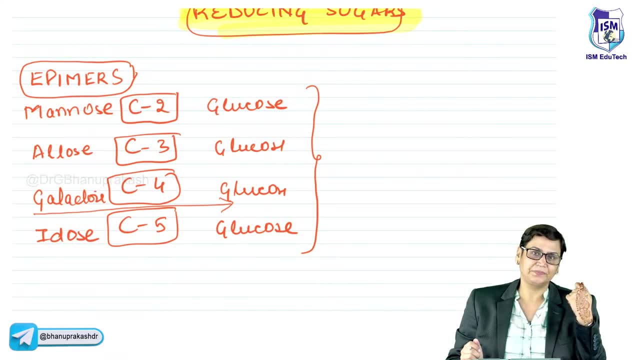 as reducing sugars or not. why no, they won't have a c1 free, you? so I'll tell you, epimers also will be reducing sugar. now why they will be reducing sugars? because in reducing sugars- key definition here- hey, they have c1 free. ok, you got my point, so see, 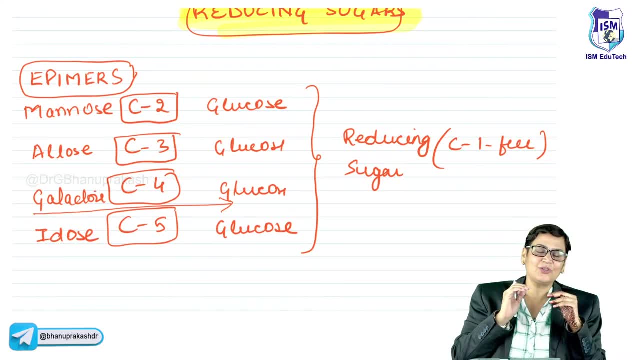 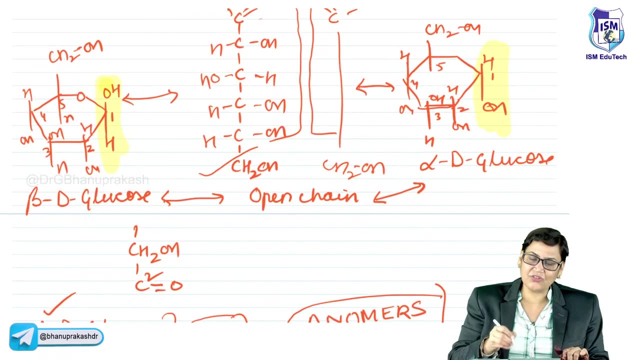 okay, see you, that's it. you. That is not ring form. actually, that is a cyclic form. This is a open chain form. I will just show you: This is a open chain form. structure of glucose: This is a cyclic. This is known as Fischer projection. 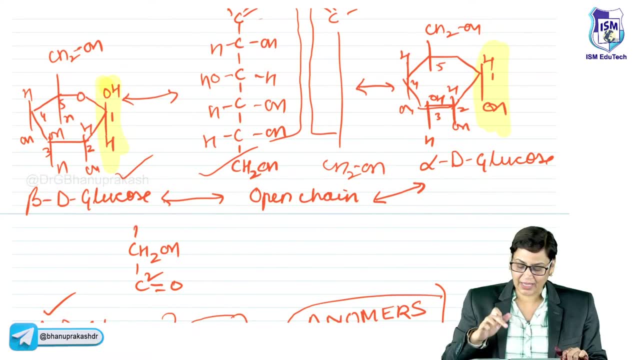 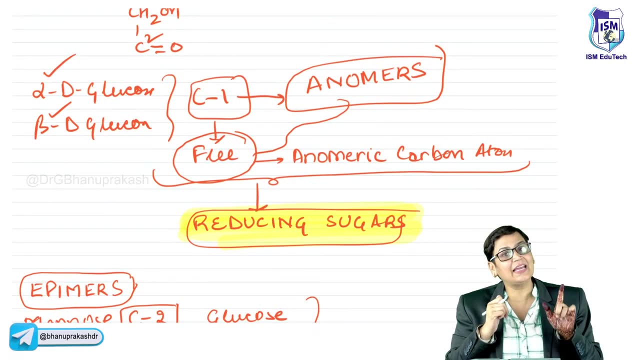 This is known as Haworth projection. Okay, And depending, coming over to this, they all have a individual identity. Anomers are differing at C1.. Okay, Alpha and beta Reducing sugars are the ones Which have free functional group, And functional group is always positioned at C1. 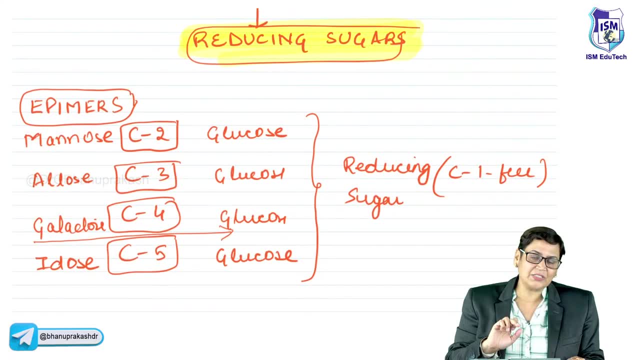 Now coming over to epimers. Epimers, kya hai. These are the isomers which are differing at any other position except C1. So C1 will be the same Whether it is alpha and beta. that is something else. Okay, But they will have C1 free. 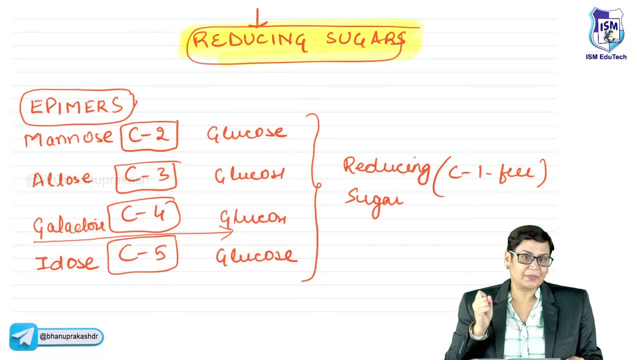 So they will be reducing sugars, Isn't it Now? you got my point, Nagesh. is it clear now? So I can say that epimers will also be reducing sugars provided C1 is free. If C1 is not free, then they won't be reducing sugars. 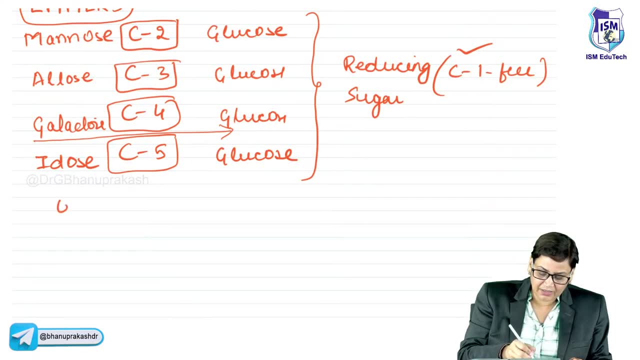 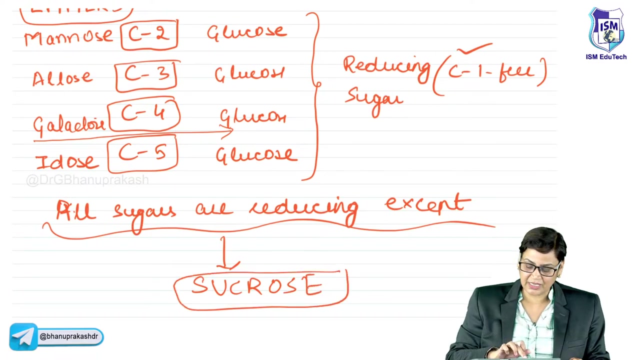 And always remember: all sugars are reducing, All sugars are reducing, except sucrose, Sucrose. You must just remember this bottom line. One more is there Three hellos, But here we will be mainly focusing on sucrose, Because all of you are familiar with sucrose. 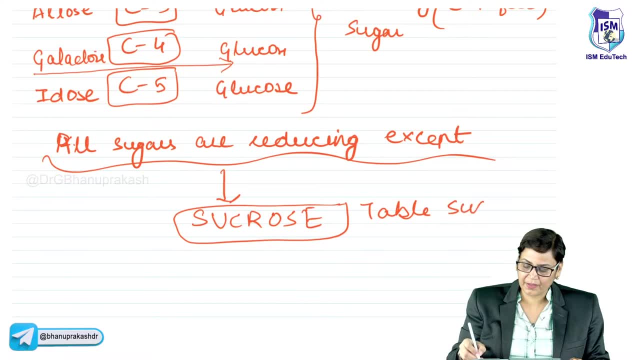 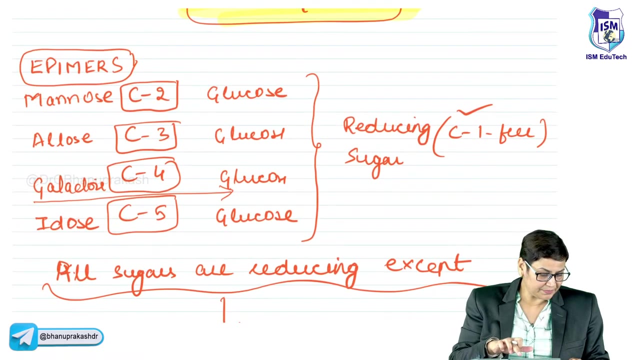 Which is the common table sugar. So, irrespective of anomers, epimers, all are reducing. Even starch is a reducing sugar Right, Even though it has one reducing end and the other non-reducing end. So these are what Is I dose. 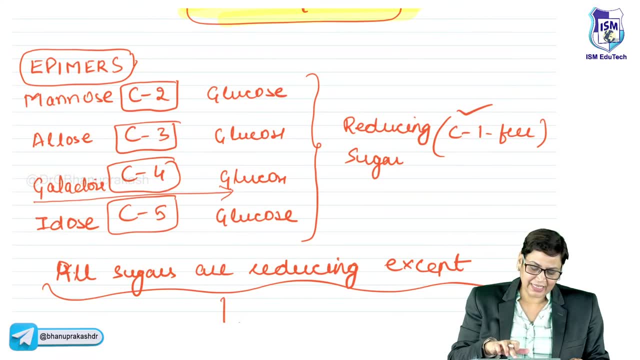 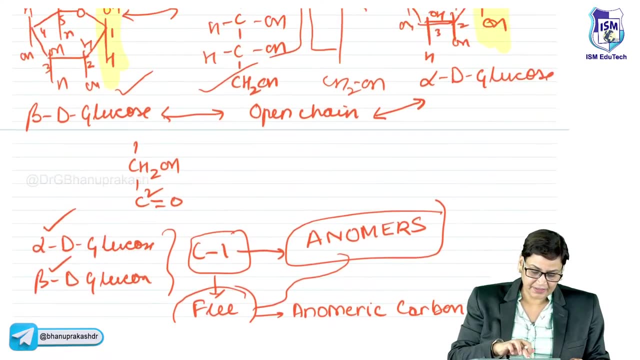 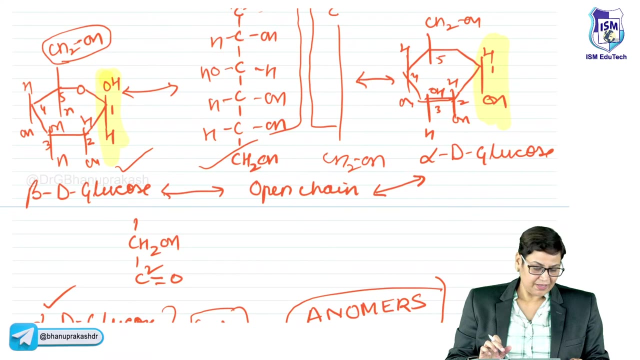 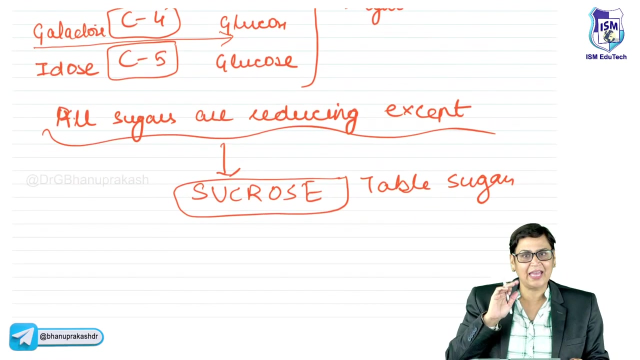 You can say that beta, yes, cyclic L-glucose. the only difference will be in the 5th position, Because if you see the 5th position here, CH2OH is there. It will be changed there, Right. So here, what we got to know is anomers, epimers and reducing sugar. 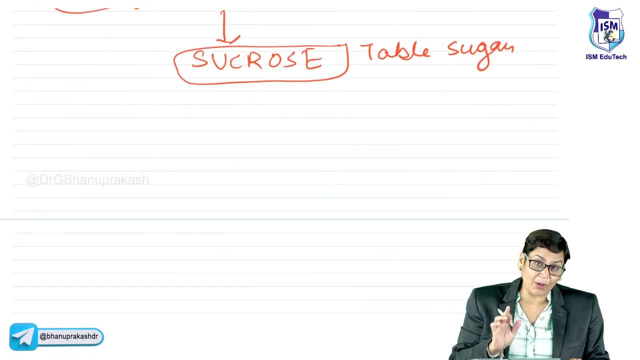 Now another important concept, since we are dealing with the properties. A very interesting property of the reducing sugars is that they have a tendency to undergo mutarotation. Muta means Rotation, means, you know, rotate Muta means within itself. So if a molecule, or you can say whenever we talk about the solution, 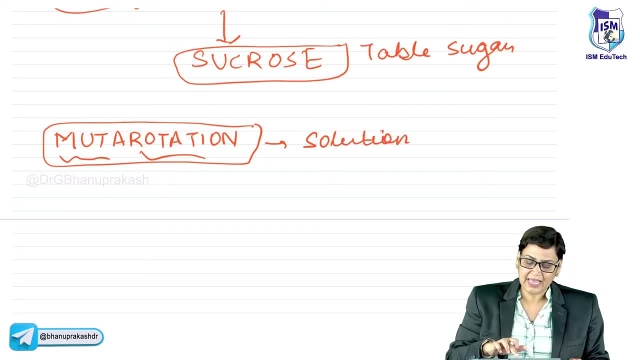 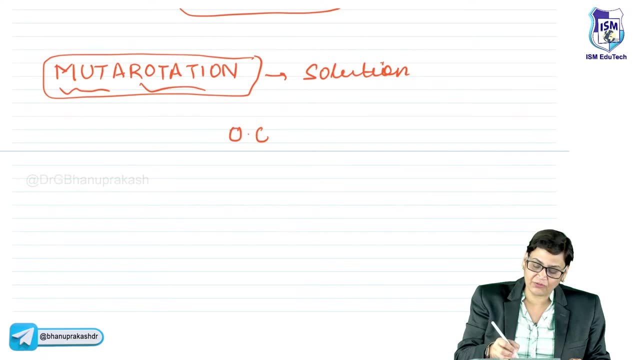 Right, And this solution is allowed to rotate within itself. It will change from the open chain form to alpha form, or it can change to beta. So we can say that all the reducing sugars have a tendency to undergo mutarotation. All reducing sugars have a tendency to undergo mutarotation. 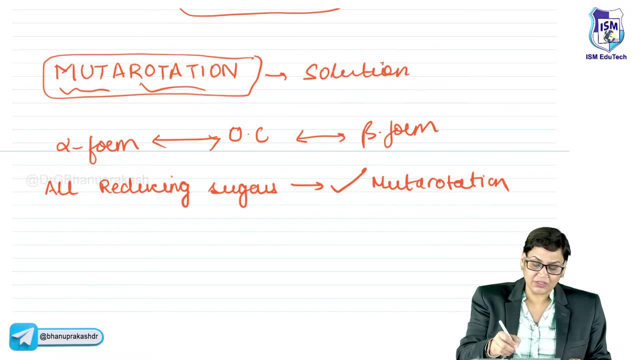 So I can say that sucrose will not undergo, do not undergo mutarotation. Muta rotation is tendency to rotate within itself. Whenever you know, whether it is glucose, whether it is fructose, whatever sugar is dissolved, it forms a solution. 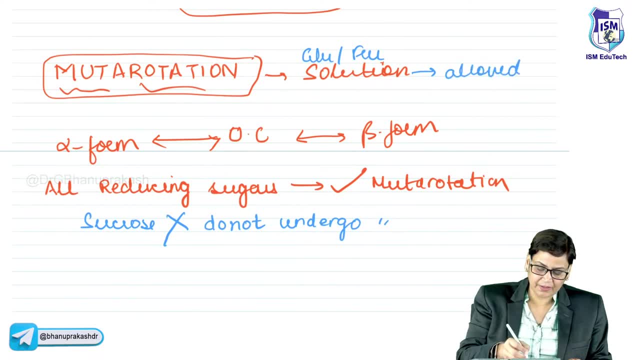 And it is allowed to rotate. Yes, Invert sugar- Sucrose is an invert sugar, So, but sucrose will not never undergo mutarotation. There is a reason behind that why sucrose is known. Okay, So what is the reason behind that why sucrose is known? 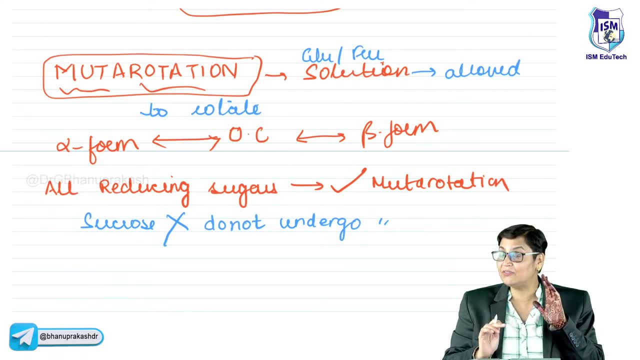 Well, sucrose is known because sucrose has the tendency to rotate within itself along the again functional carbon atom. Just remember this, because that is what I have shown here. You can see that this open form can go to alpha form, can go to beta form, or the three forms are interconvertible with respect to one another. 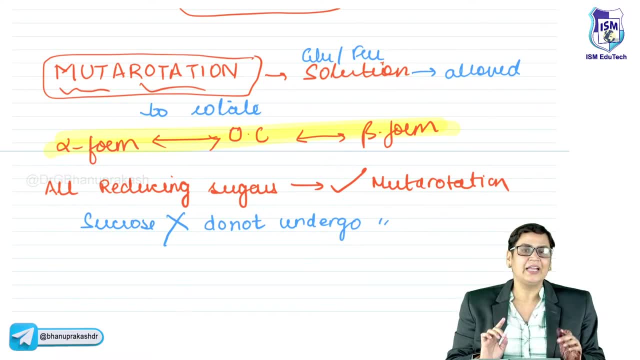 So this is a characteristic feature only of reducing sugar Tendency to rotate within itself. If glucose wants to be in open chain form, wants to be in open chain form for some time, glucose will be in that form, suppose. if glucose wants to go in a stable conformation, it might change to beta form, it might change to alpha form. 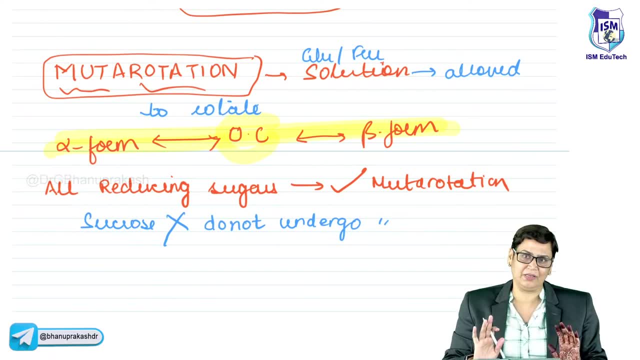 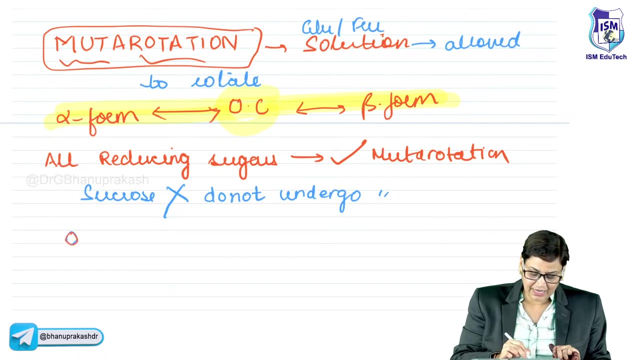 so, again, the angle of rotation will be different, but it will be stable. okay, so this is what is muta rotation, then, another important property linked to this is osa zone formation, a very important, i should say, property from examination point of view also, osa zone formation. 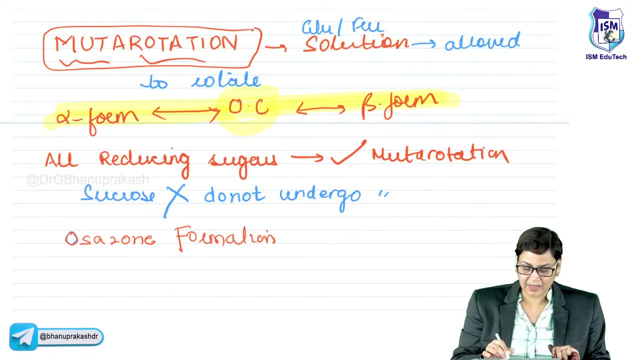 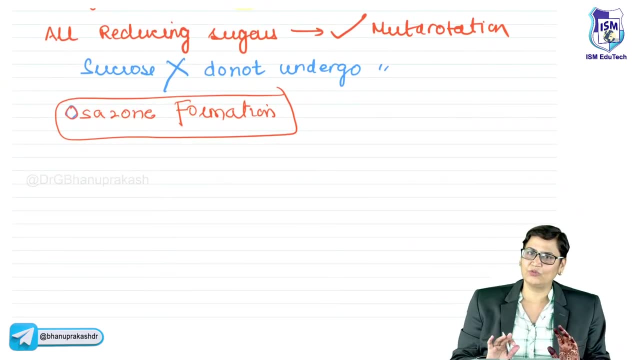 i'm now see again. i will just give you a very simplified version of osa zone formation. what happens is we simply take these reducing sugars: glucose, fructose, galactose, mannose glucose, or you can say other diacycrides, whatever reducing sugars are there. 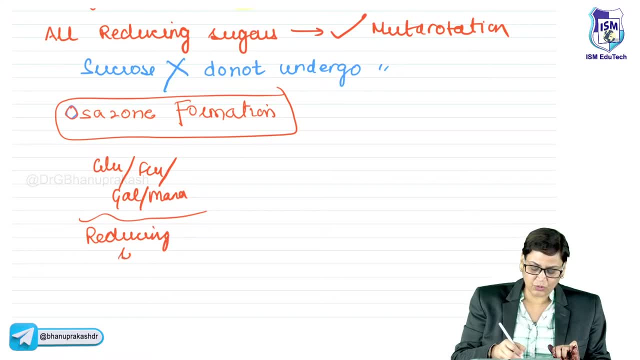 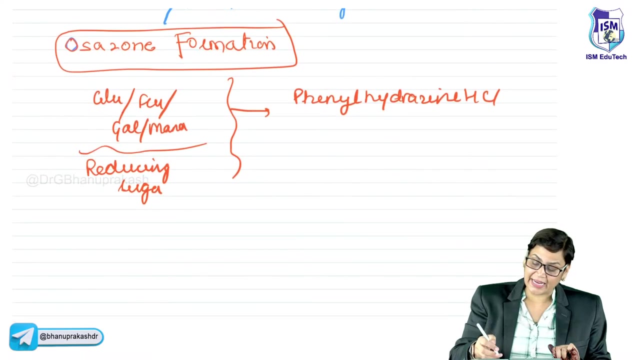 right. what we do is we make a solution of these reducing sugars and we add phenyl hydrazine into it: phenyl hydrazine hydrochloride with anhydrous sodium acid. right, we keep everything in the same order, so we have a solution of these reducing sugars: glucose, fructose, galactose, mannose. 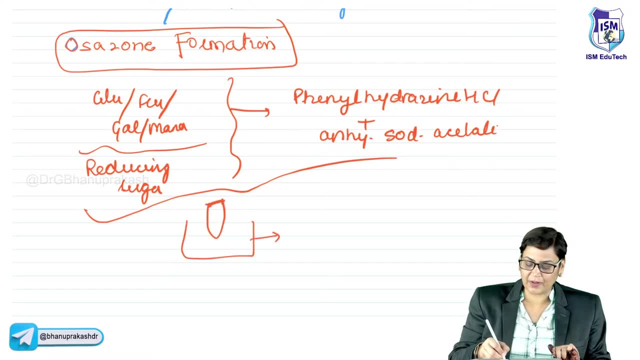 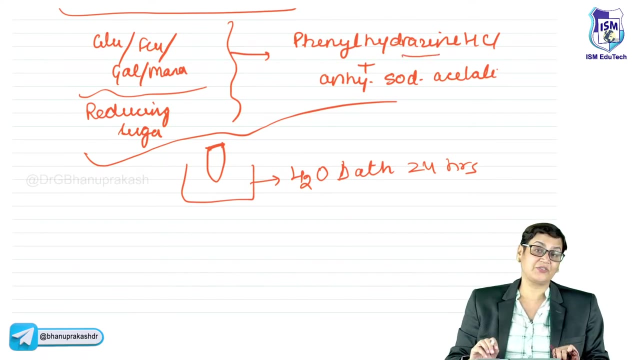 glucose fructose, galactose, mannose in a test tube like this and we keep it in the water bath for 24 hours. obviously, glucose fructose, galactose. depending upon their functional groups, they are going to phenyl hydrazine, c6h5, NH, NH 2. again, i am taking a talking. 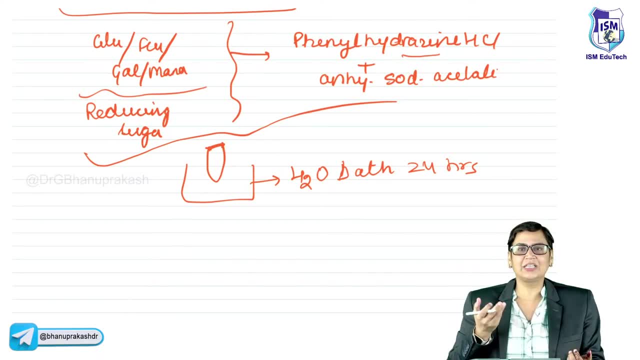 about chemistry: NH, NH 2, you know. water molecule will be lost. it is going to form a phenyl hydrazine. wherever functional group is free is going to form a glucose zone, fructosa zone, galactosa zone, maltosa zone. So this is what we are forming, what we are getting. 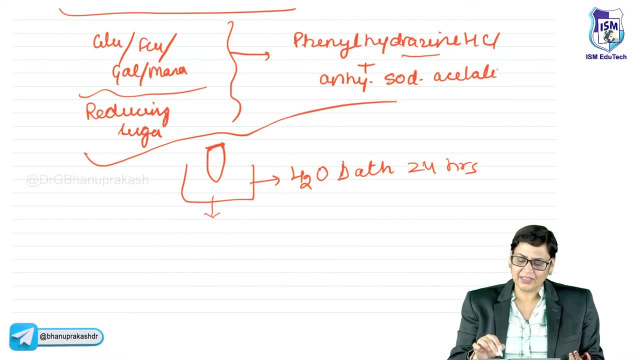 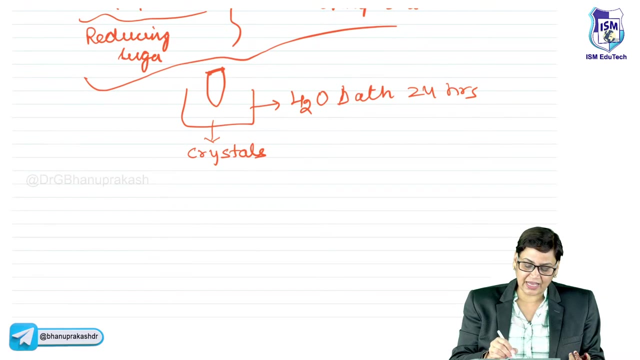 because every molecule has a tendency to form crystals. This is basically acting just to dehydrate it, because we are keeping it in the water bath, also for some 24 hours. So then what happens is formation of crystals is there, and these crystals are then taken out and we put them. 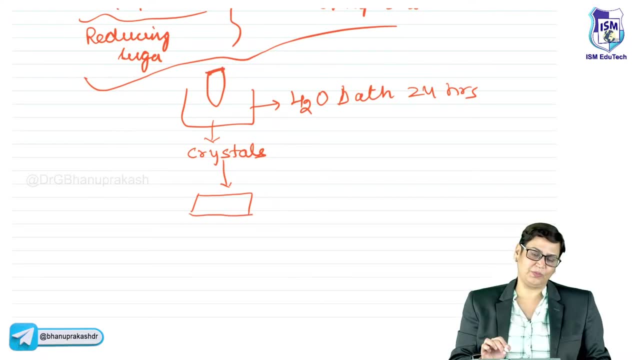 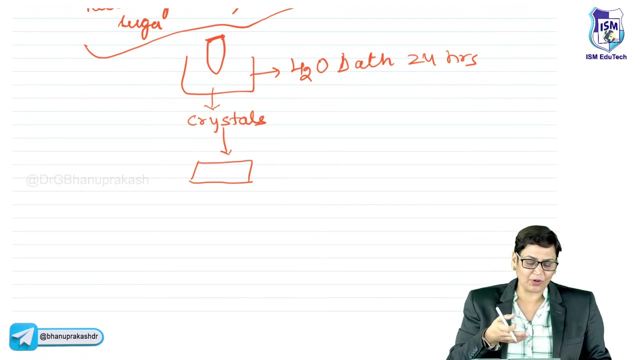 on a slide and we observe them under the microscope. So obviously we have to properly tease the crystals so that we can visualize, and you will see that I think you are going to perform this practical also in your first year. This is again a very interesting practical. So, depending 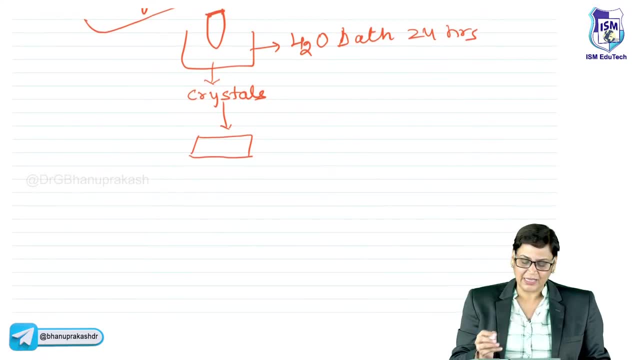 upon the shape of the crystals we identify which sugar it is. So if I talk about glucosa zone or glucose crystals, glucosa zone. So if I talk about glucose zone, so if I talk about glucose crystals, glucosa zone. So if I talk about glucose zone, 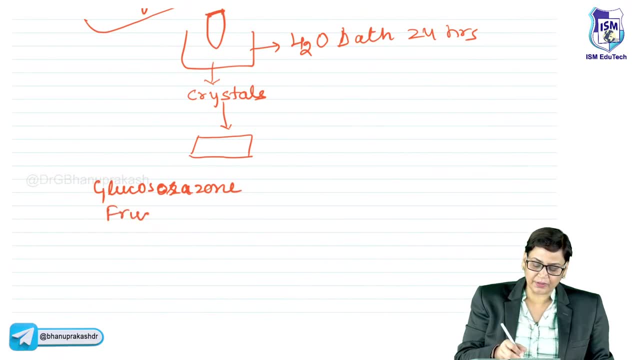 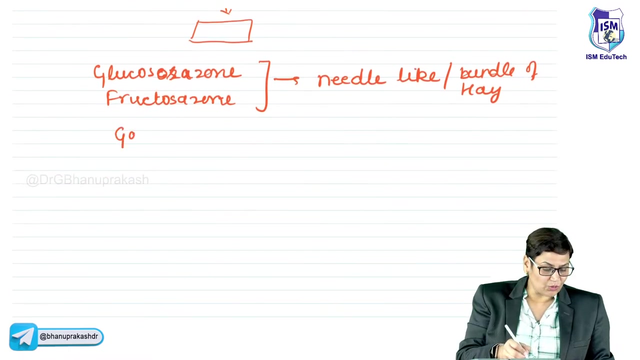 or fructosa zone. the shape of the crystals is needle like Or it's like bundle of hay. Okay, if we talk about the structure of galactose, galactose has corny and edge like, structure, Edge like, or it's like. crystals are thorny- thorny like you know. they say 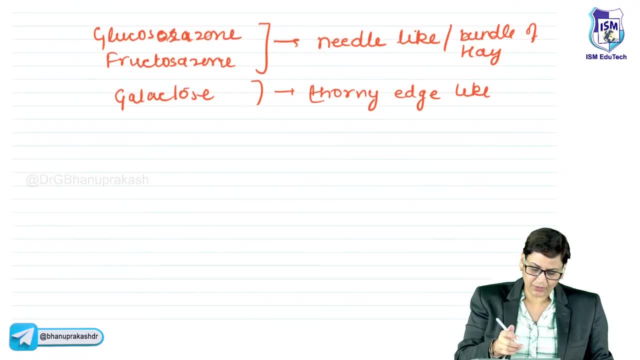 those thorns are there, just like that pointed. Okay, then, if we talk about lactose or lactosa zone, because lactose- abhi we have not discussed the structure of lactose. it is a disaccharide, But here we are focusing on the reducing sugars, So lactose also has. it also shows crystals and the shape of the crystals is needle, like So, if I talk about lactose, galactose has corny and edge. like So, if I talk about lactose, galactose has corny and edge. like So, if I talk about lactose, galactose has corny and. 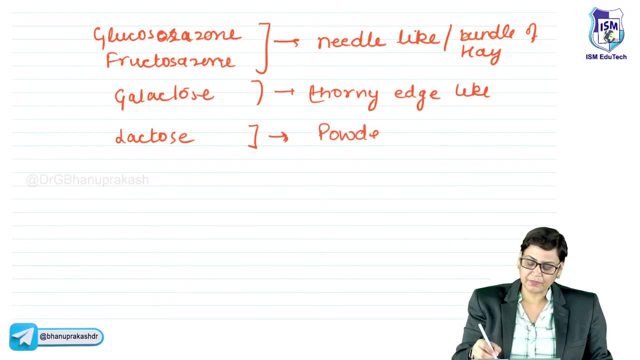 edge like. So if I talk about lactose would have partout as a total such like SNP . �� Like tension is musical tension or Renov bookstore if you want. So you can say that crux of the crystals of lactose will be powdery puff. Right. And then maltose it is known as maltosa zone and maltose is sunflower petals sunflower like petals 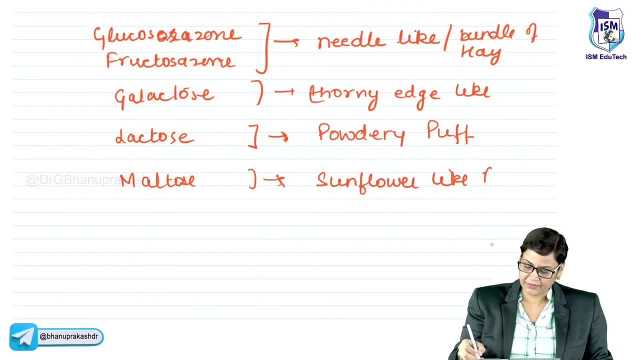 �� �� �� �� Ok Tell Me smart So you can say that osa zone formation is against particle ratio. Of course the vet may guestкт Ace max, or man of water� dataM 568 of canal particle ratio is against blood� capable of halogen detection of liquid proteins plus统 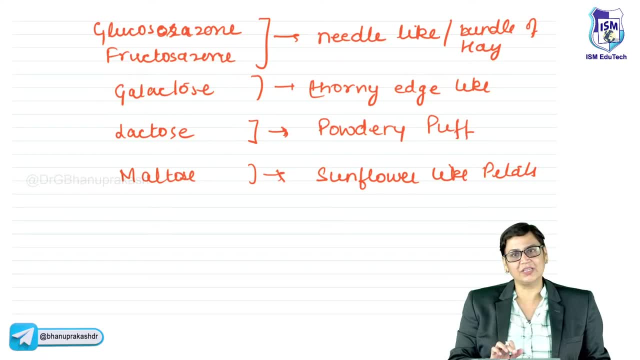 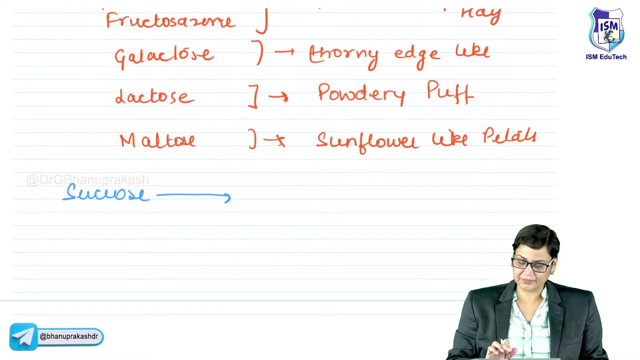 a characteristic feature of reducing very, very. we eat glucosa zone, we eat fructosa zone, galactosa zone, lactosa zone. now, depending upon this finding, can anybody tell me what will be the shape of the crystals of sucrose? you now tell me: yes, very good, no change or it will not form crystals. why it won't form crystals? 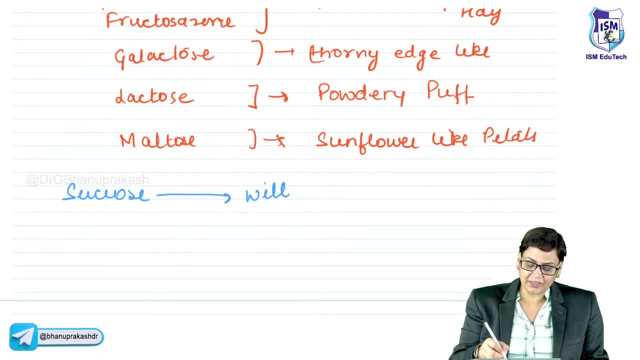 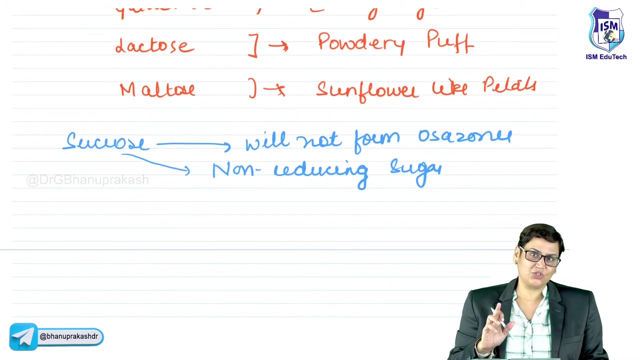 because sucrose will not form the zones reason. kya hai sucrose is the only non reason. kya hai sucrose is the only non reason. kya hai sucrose is the only non ready correct? so you can say that all reducing sugars will undergo mutarotation, except sucrose. all reducing sugars will undergo. 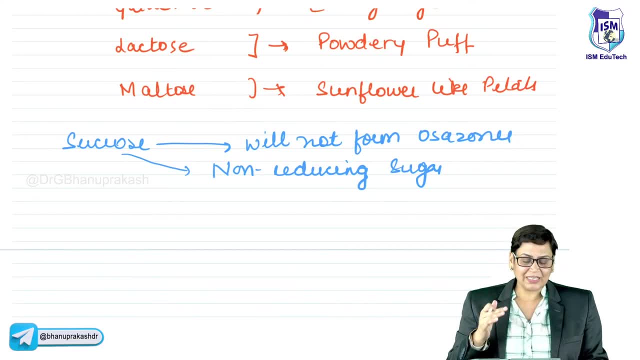 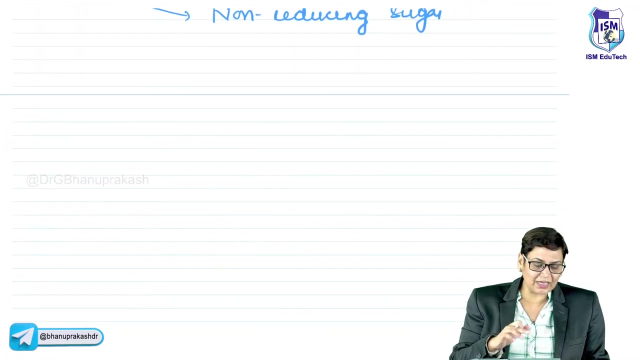 osa zone formation accepts. so these are very, very important properties of monosaccharides. or you can say: reducing, this may what we covered, anomers, we covered. so this may, what we covered, anomers, we covered anomers. we covered an epimer. then after this, we come over to the oxidation and reduction properties of 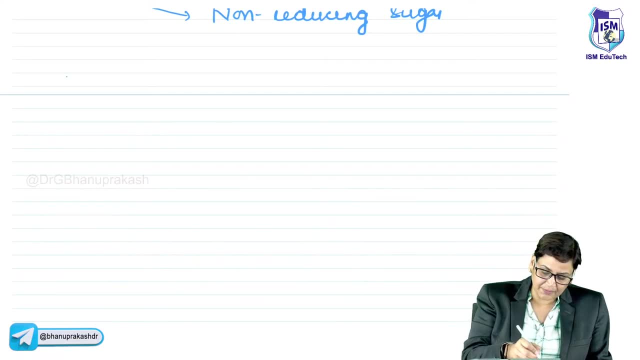 just say, for example, if we talk about oxidation up see oxidation again. i will just tell you about the chemistry part of this. you know, cho ch, oh, 4, 5 and 6. this is the structure of glucose if glucose undergoes oxidation under mild oxidizing agent. 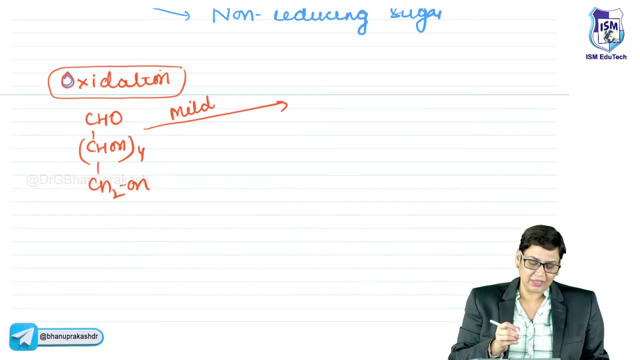 file means very light. you know, aldehyde group is more susceptible towards oxidation, they say all of you must have prepared for your, you know, this ug neat exam which may you must have studied about ascend of series conversion, this end of series. alcohol to ld, high to carboxyl isn't it. and ultra is. 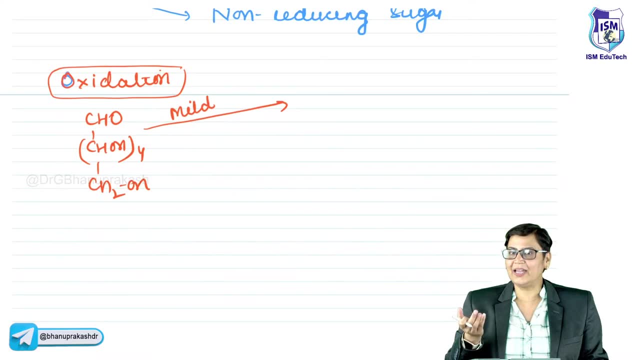 reduction. so we can say: alcohol is oxidized to ld height, ld height is oxidized. oxalic acid: here ld height is there immediately. it will be oxidized even in the presence of a mild oxidizing agent. we perform the reaction in strong oxidizing agents. both will be oxidized. 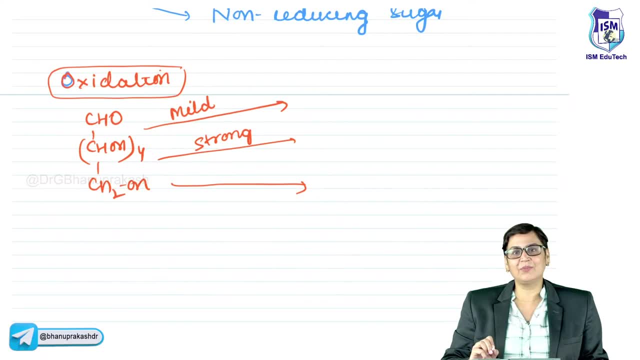 right. a question is when this reaction takes place in the body. what happens if we talk about mild oxidizing agents? simple, you can say: aldonic acids will be produced- gluconic acid, fructonic acid and so on. but in the presence of strong oxidizing agents, 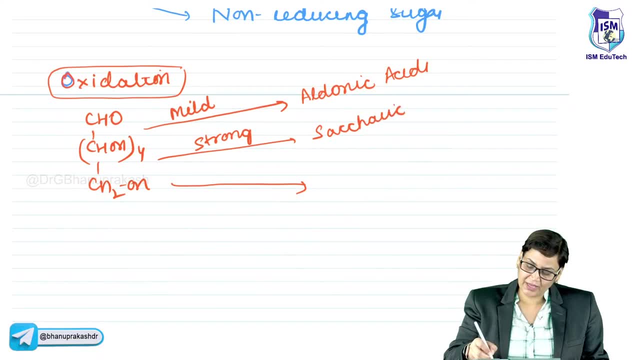 saccharic acid will be okay. saccharic acid means both the groups will be oxidized. glucaric acid is there right? and now the question arises: we have to hide this means we have to oxidize this primary alcoholic. pretend that means we are not oxidizing this aldehyde. 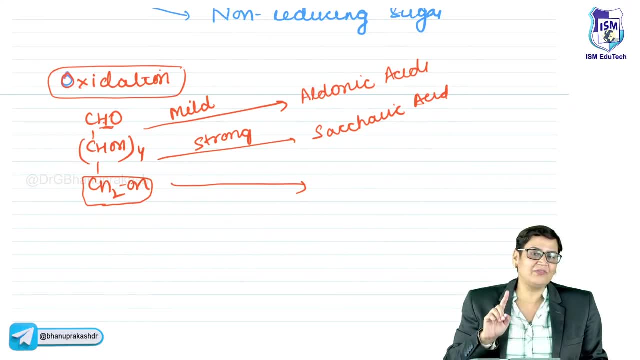 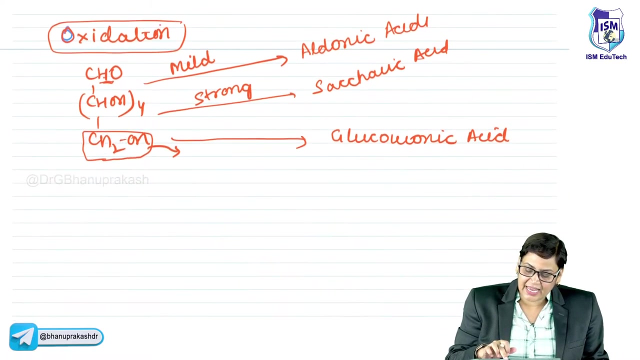 this can take place only in the body with the help of the enzymes, and that is what exactly happens here. gluconeuronic acid is there, and that is what exactly happens here. gluconeuronic acid is there, acid is produced. So uronic acid is produced when this group is oxidized, And this reaction 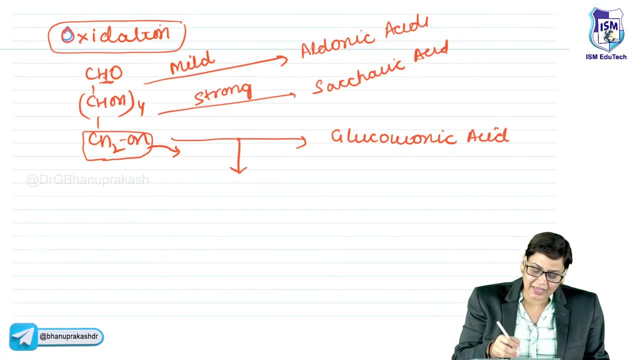 takes place by a very, very important pathway in the body, which is known as uronic acid pathway, which is considered to be a alternative pathway of oxidation of glucose, And this pathway occurs in the body just to synthesize this glucouronic acid. Most of the students 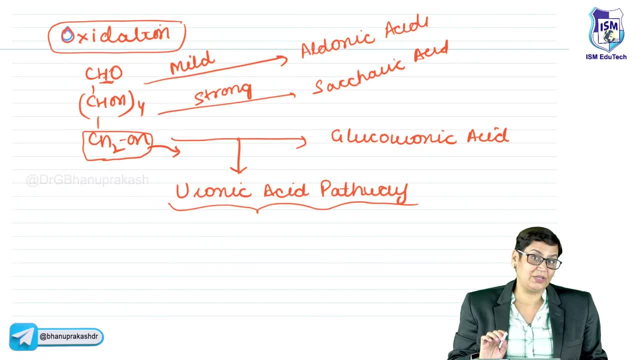 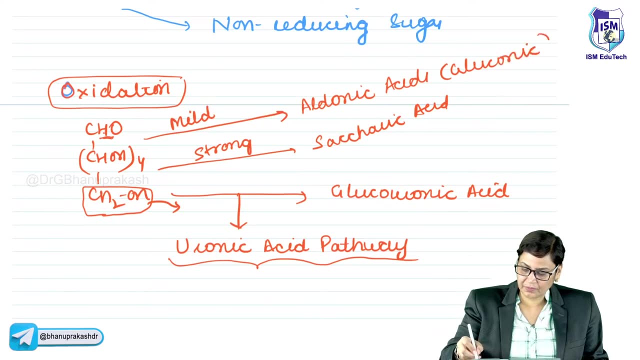 might get confused between gluconic acid and glucouronic acid. I will just write it here: Gluconic acid and glucouronic acid. By the way, just remember uronic acid means which is produced as a result of. That's why I have written the spelling also: Gluconic acid and. 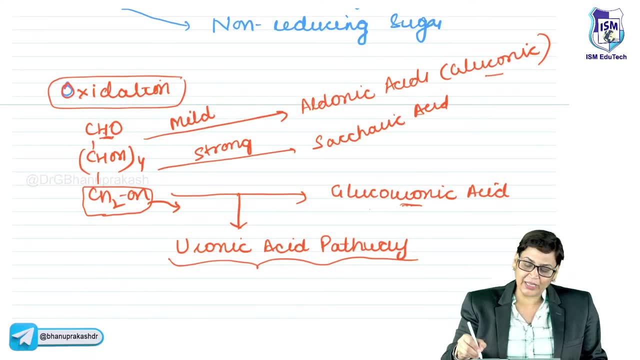 glucouronic, See the spelling. Gluconic means aldonic acid, which is under mild oxidizing acid, Glucouronic acid, which is synthesized by a uronic acid pathway. Whenever we talk about any of these things, we are talking about a uronic acid pathway. So this is a 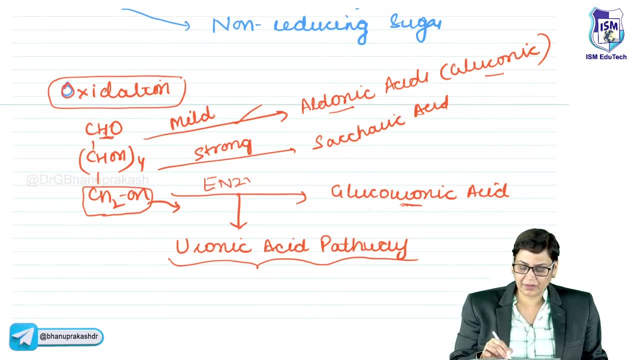 pathway. Simply write the enzyme, So this reaction takes place in the presence of the enzyme. Okay, And glucouronic acid plays a very, very important role in our body, Very important role. It is considered to be one of the very important, I should say, detoxifying. 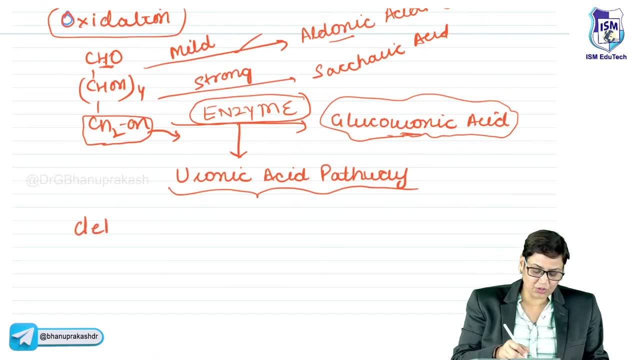 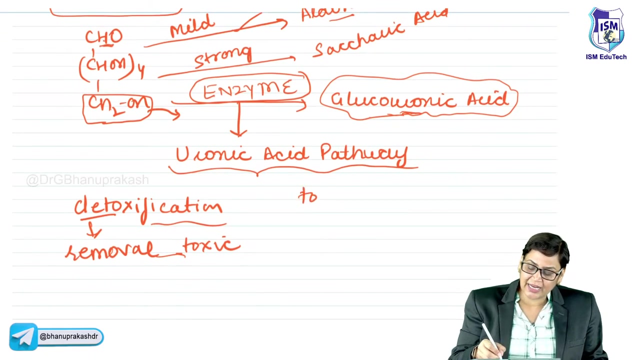 agents. Detoxify means detoxification, D means removal, Toxic means, you know, toxic, which is harmful. So glucouronic acid helps in removal of the toxic substance, Or it converts toxic into non-toxic So that they can be. 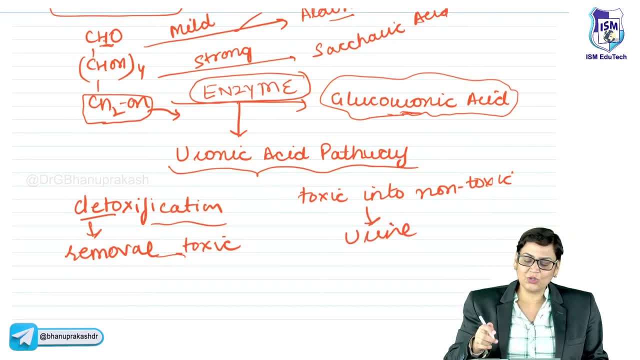 excreted in So slowly, slowly, you will study, So you will study, So you will study, So in the metabolism, that how this glucouronic acid is produced. And always remember there are so many similes in biochemistry, So do not get confused. I will show you so many. 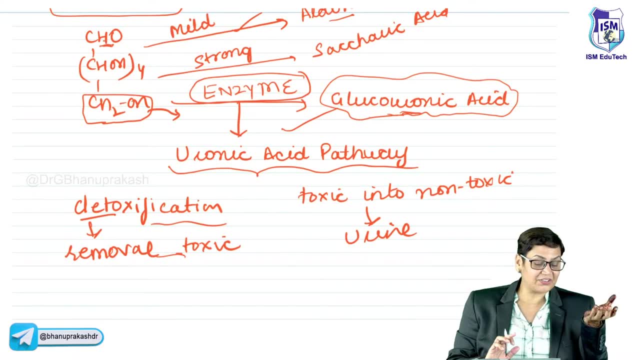 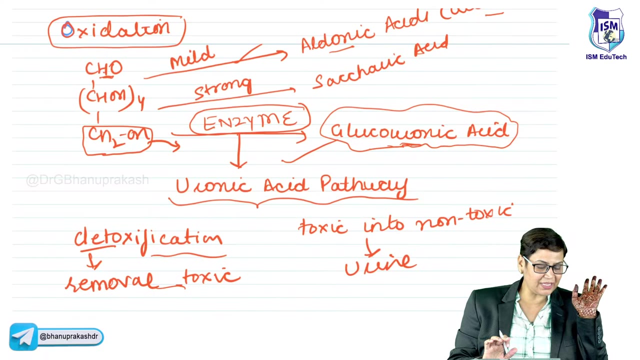 similes: Inulin, insulin. Is there dextrin, Dextrin. is there One live example is there in front of you? Only glucouronic acid and glucouronic acid. Yeah, So is not it interesting, Right? So oxidation may just remember one thing: that glucouronic acid is a very important. 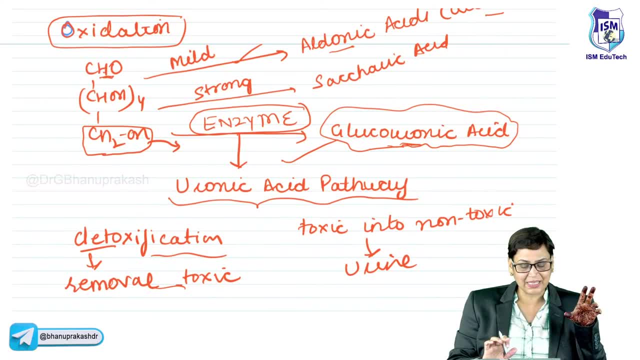 thing So in the metabolism, that how this glucouronic acid is produced with the help of enzymes And rest is in the presence of either mild oxidizing agents or strong oxidizing agents. Clear, Then, coming over to the second property: reduction. 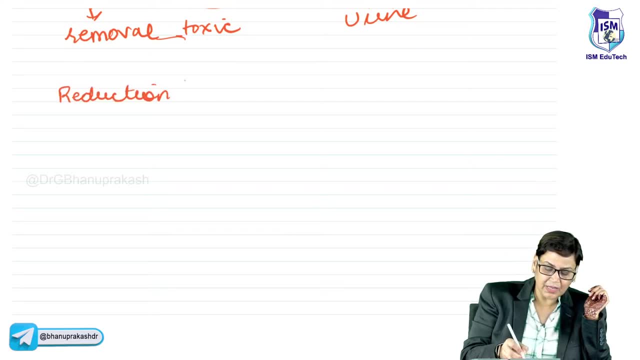 Now see reduction ke liye. always remember it is actually the enzyme, Because enzymes, I told you, they are the ones which are catalyzing the reactions. So the enzyme is deoxylic dehydrogenase. Okay, Now again, I will give you one very simple concept. If I talk about 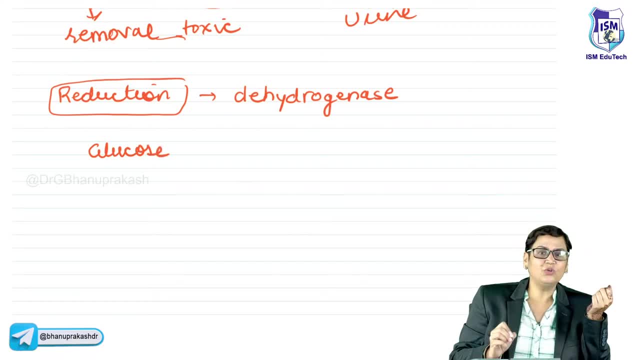 glucose. Glucose is a aldohexose, So the enzyme responsible for reducing glucose will be aldol, either dehydrogenase or, I can say, aldol reductase. If I talk about fructose, again the enzyme will be reductase. If I talk about galactose, the enzyme will be reductase. 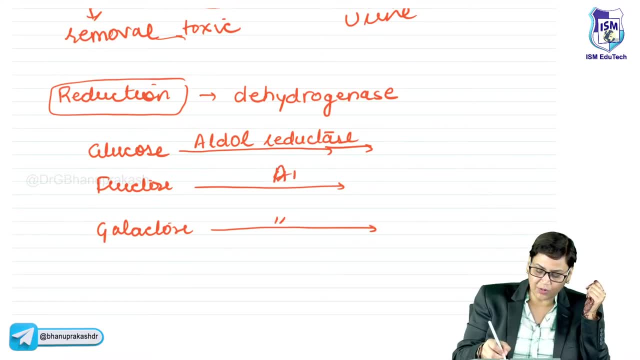 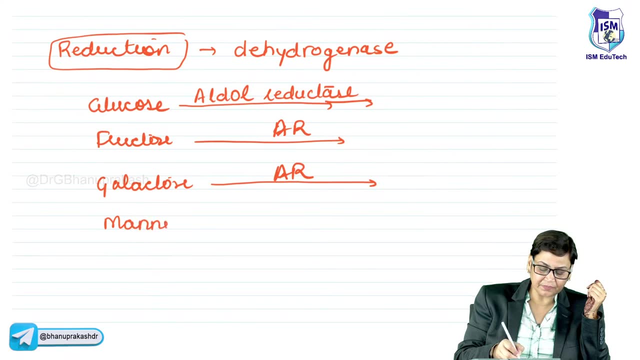 I will just write the plot form: AR. And similarly, if mannose is there, the enzyme is again aldol reductase and the product will be reduced. Okay, Now one very, very important concept that we need to know about this enzyme is: this enzyme consists of zinc also sometimes. 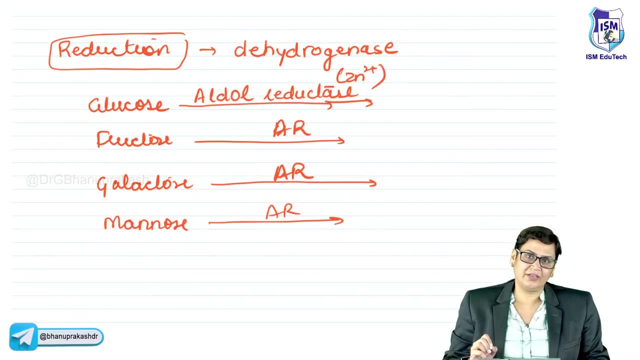 Zinc acts as a co-factor for reduction. Zinc is the major co-enzyme or factor for dehydrogenase, But sometimes it acts with reductase. Okay, When more enzyme is there again. don't get confused with alcohol. dehydrogenase We will be after chemistry of carbohydrates And the thing is that, as it is very important to you to always be aware of this And do not forget to make the revision. See, you have seen this video. we have topology of a molecule: How The enzyme has the function of the enzyme, So it has the function of the enzyme, So that 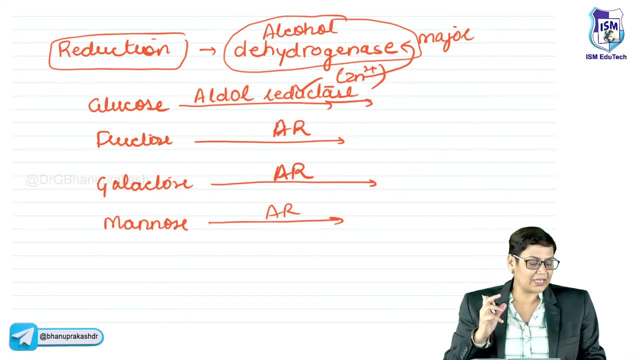 carbohydrates. we will be taking enzymes. Then I will show you what is the basic. Yes, I am telling you better. The enzyme will be reductase. It is not ketal reductase. It will be keto reductase. It will be keto reductase. It is not ketal. Ketal is altogether a different. 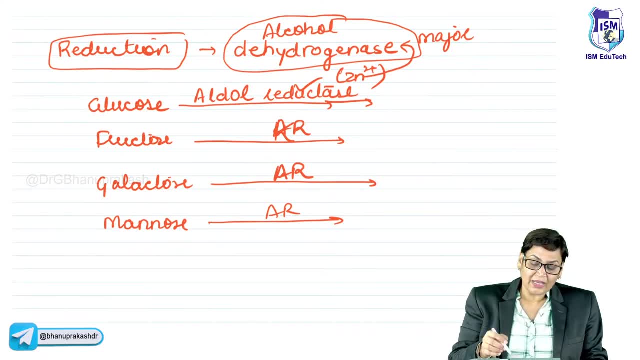 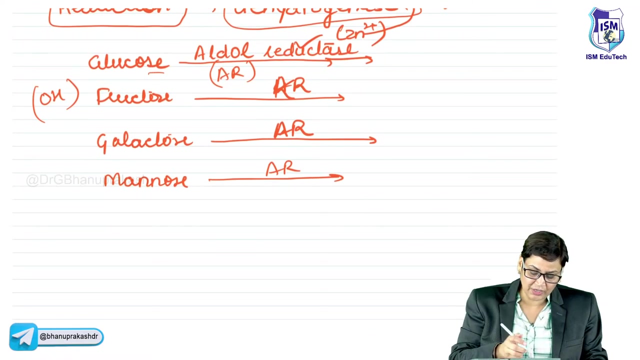 product: Okay. So alcohol dehydrogenase- we always write it as ADH- Okay. And aldol reductase is AR, Means glucose, which has aldol, Aldol means OH. actually We can also say fructose is aldol reductase, Because if you look at the structure of fructose also, 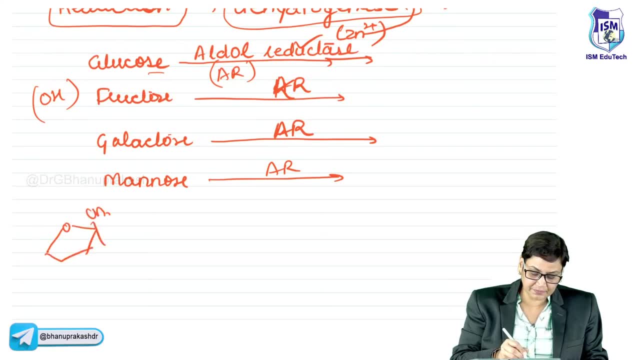 fructose also has this type of structure, isn't it? OH, is there? Okay, So aldol is coming. Aldol means it is coming from ole, Ole is coming from this OH. So even if we write it as aldol reductase, then also it. 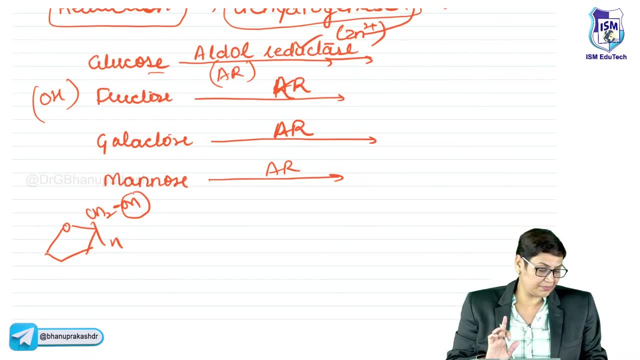 is correct, So don't get confused. Okay, It is oxidation of this. So glucose and fructose are going to form sorbitol, Right Sorbitol. If we talk about galactose, galactose will form galactitol, obviously. 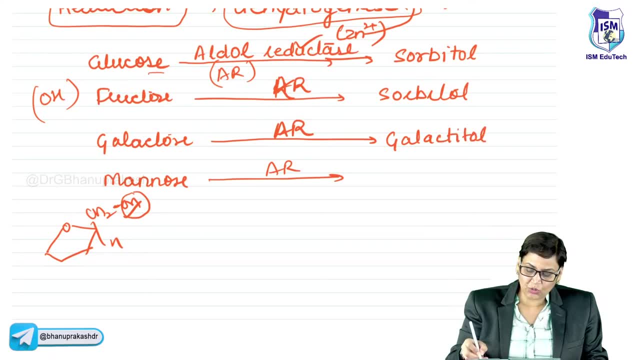 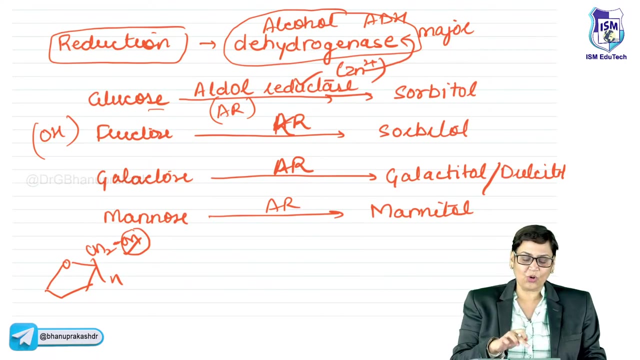 Galactitol, But it is also known as dulcitol In some books. it is given as dulcitol And mannose will form mannose. Okay, So you can say: here we are talking about reduction, So all the reducing sugars will have a tendency to undergo reduction in the presence of enzyme. 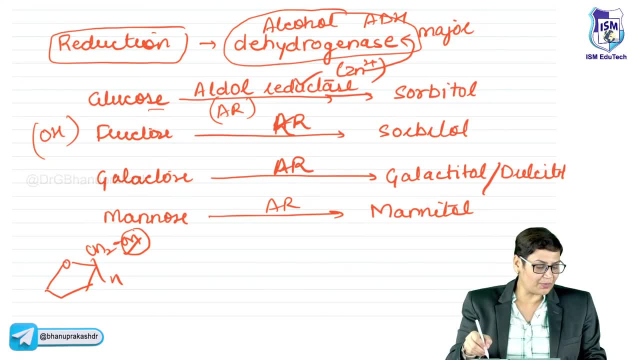 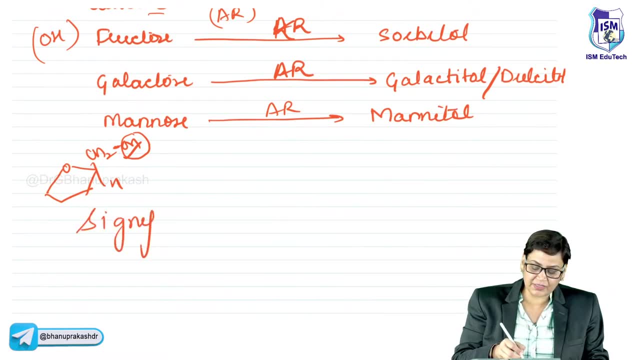 aldol, reductase, Sorbitol, sorbitol, galactitol, mannose. This is so important that we can help elevate our brain to develop good brain function for a long time. Hey, If you have any questions, you can ask me in the comment section. Thank, 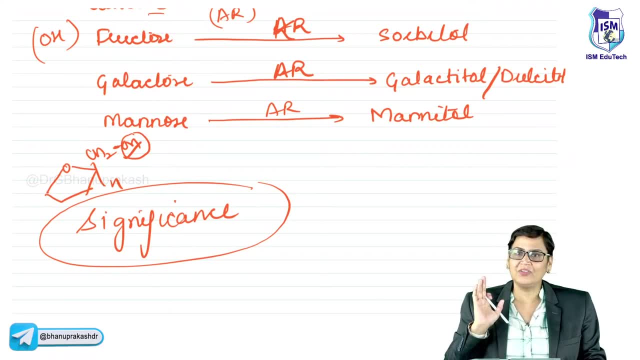 you very much. Awesome, Thank you very much. Thank you very much for your question. Thank you, Thank you very much. Thank you very much about the universal sources. carbohydrates are the ones, and you know excess amount of carbohydrates are converted, fats also and they are stored. 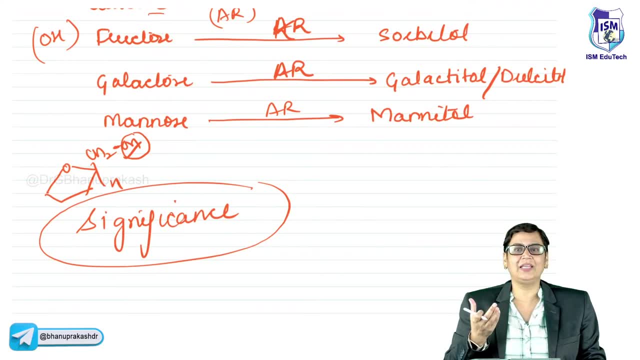 in the form of fats. proteins are required for them, for building up of the muscle mass, and fats are the instantaneous sources of energy, because even when fats break down, they form a intermediate, which is more or less. really this only okay. so what is the significance of this? up now? see, we are. 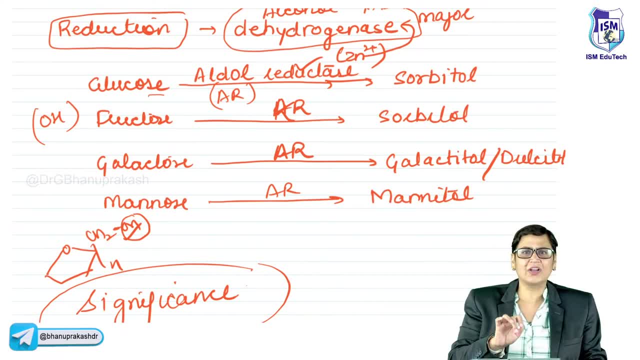 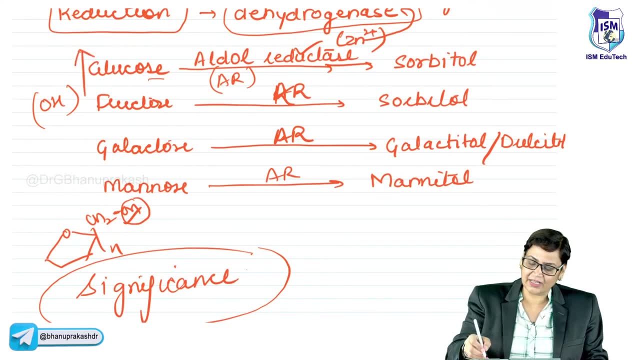 having carbohydrates, we are having glucose, fructose, whatever we are having, whenever there is increased concentration of glucose, obviously the concentration of this will increase fructose. this will increase galactose. this will increase mannose. this will increase glucose. this will increase mannose. this will increase glucose. 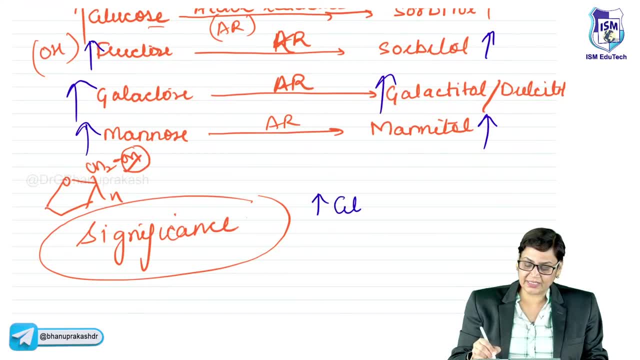 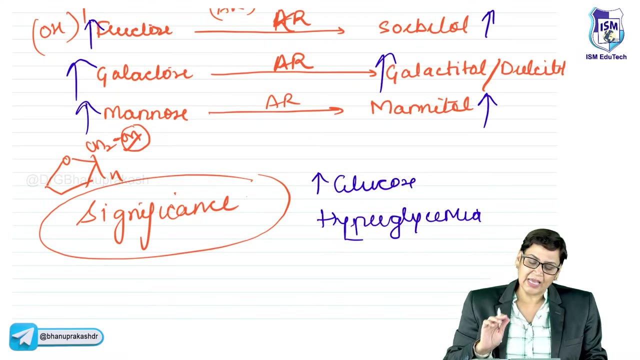 now here the twister rises if the concentration of glucose increases. remember, this condition is known as hyperglycemia. glycemia actually comes from the glycemic index. basically so hyper is increased concentration of glue. now see, whatever energy we are getting we are getting by the breakdown of glucose. okay, so glucose is giving energy to the eye. 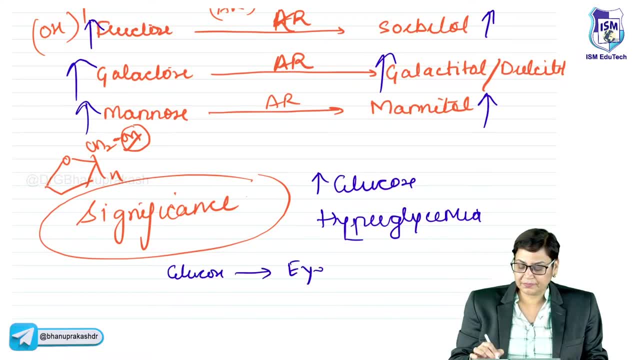 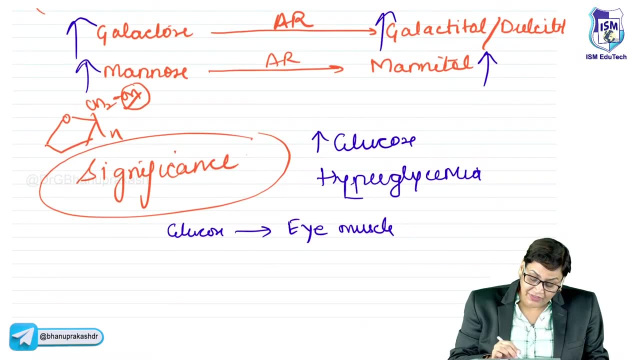 muscle is also eye muscle is also contracting, linking so many functions. so what is happening is: if the concentration of glucose increases in the eye, obviously there will be increased concentration of sorbitol. now just try to understand this, okay. in case of hyperglycemia, what is happening is concentration of glucose is 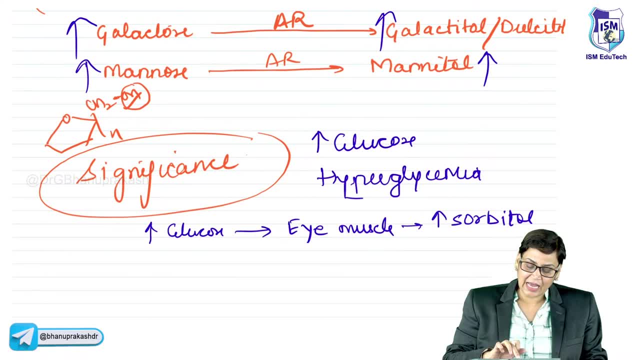 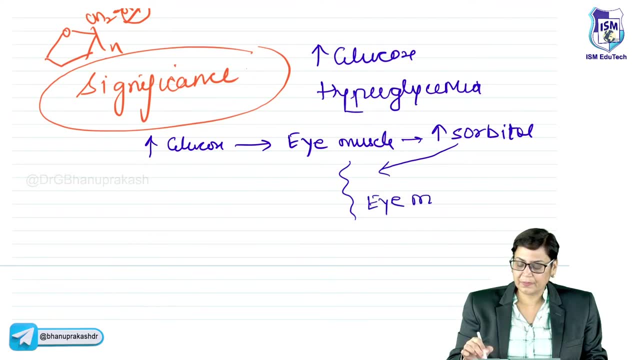 increasing concentration of sorbitol also increase up the. the tragedy with this sorbitol is it cannot cross The eye membrane. when it cannot cross the eye membrane, it is concentration will keep on increasing. keep on increasing sorbitol. it is an alcohol. it will increase the pressure. 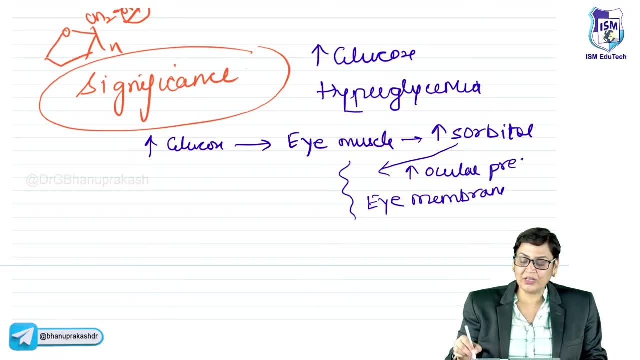 inside, which is known as ocular the. what will happen is it is like a balloon. balloon may visit the level of water increases it, my burst all Same is the case here, and that is what we say during hyperglycemia or during diabetes mellitus. the worst effect is on the eye. 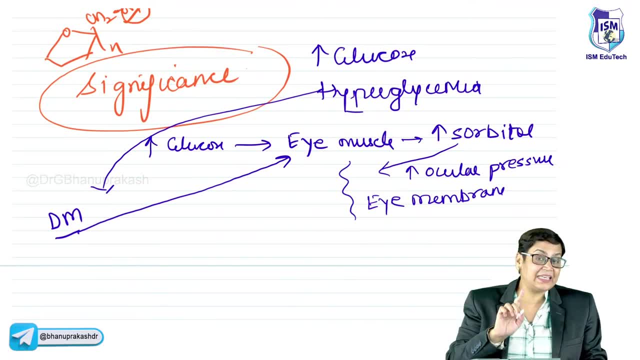 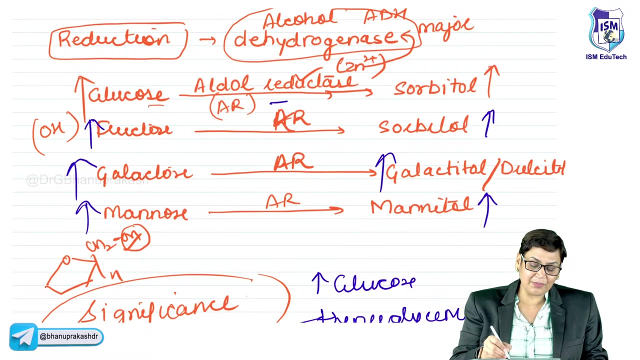 The reason behind that is there is increased concentration of sorbitol in the eye which cannot cross the eye membrane, thereby increasing this ocular pressure, thereby leading to the formation of cataract also. Now it can be reversed- again I will come to that- if we give that patient inhibitors of aldol reductase. but once the damage is done, it can be controlled, but it cannot be completely reversed. 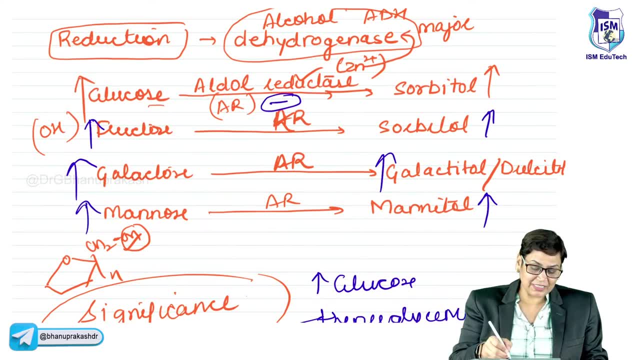 We can control it. So what happens is, if we give them these inhibitors, aldol reductase, what will happen? we will try to minimize the concentration of sorbitol, but once it has increased, There may be, you know, the blood starts oozing out from the eyes also. so what we do is we regress the blood vessel so that no more, you know, blood comes out. 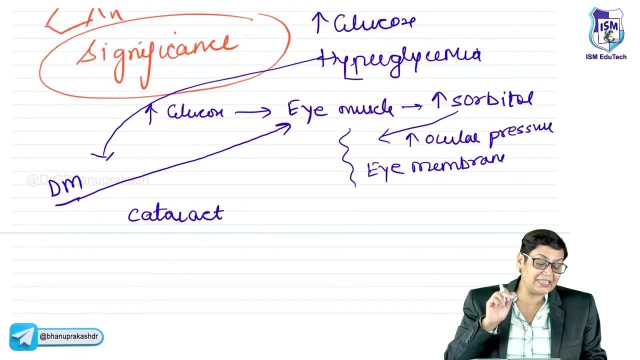 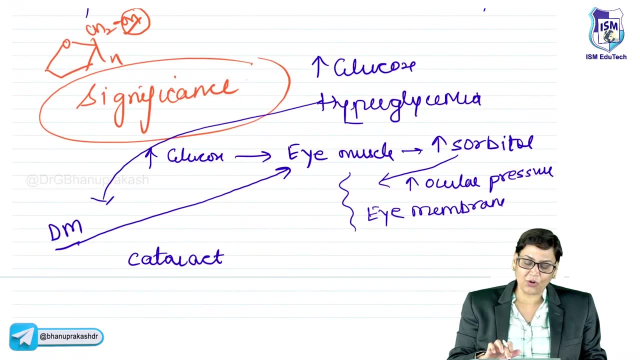 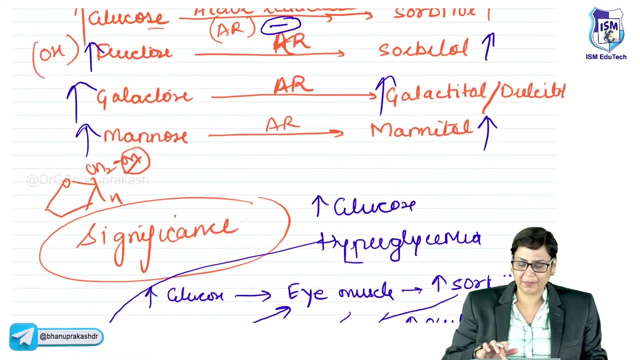 So the reason, the biochemical reason behind this is increased concentration of sorbitol, thereby increasing the ocular pressure. So most of the drugs which work on they actually they are aldol reductase inhibitors, which will try to minimize the level of sorbitol. 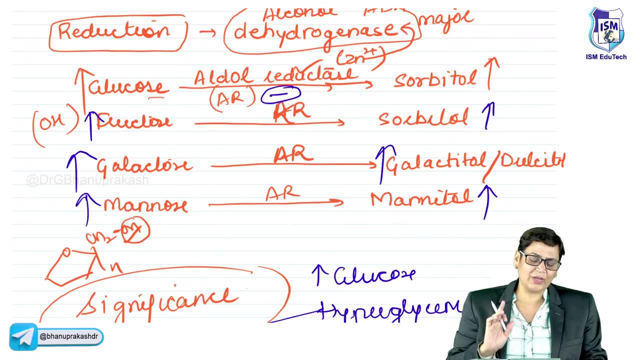 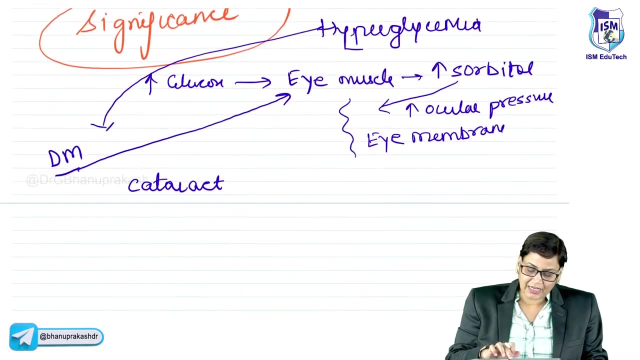 Right. So this is one very, Very important- you can say reducing properties of, and the biochemical significance also of this. coming over to galactose, galactose also leads to formation of galactitol, right? So we, right now we will be discussing, when we will discuss the metabolism. I will tell you one very important metabolism. 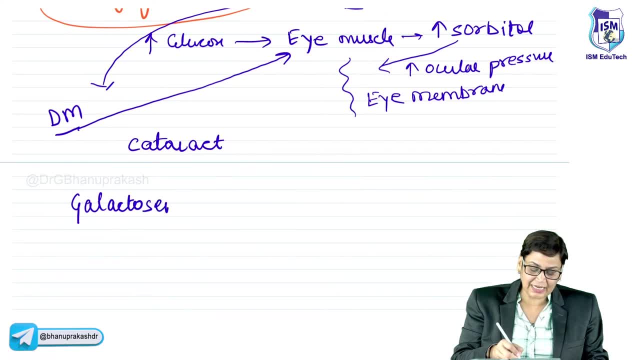 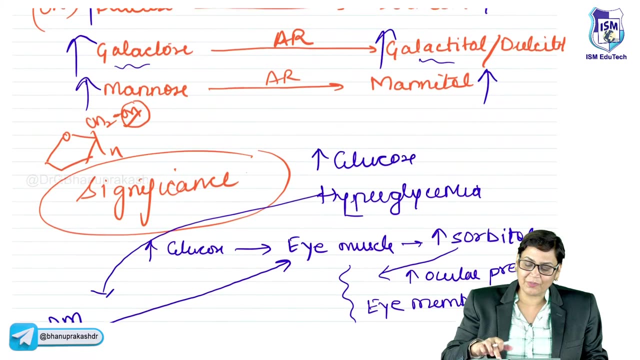 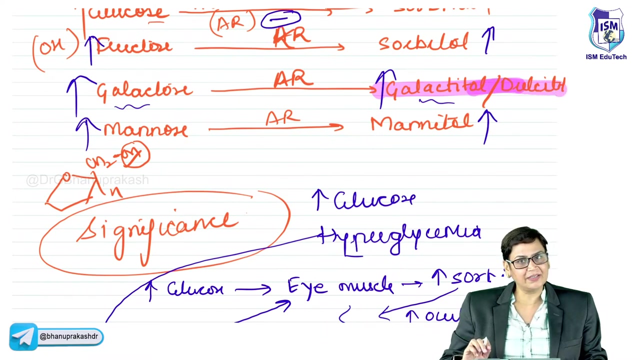 Yeah, inborn error of metabolism of galactose, which is galactosemia. Semia is blood, Whenever the increased concentration Of galactose is there in the blood. so what will happen? again there will be increase in the concentration. yes, very good, Nagesh galactosemia. so what will happen is there will be increased concentration of this galactitol. again there will be formation of, but again we will come to that the cataract formed by sorbitol and by galactitol will be different. there it is no flaky cataract, here it is bilateral cataract. 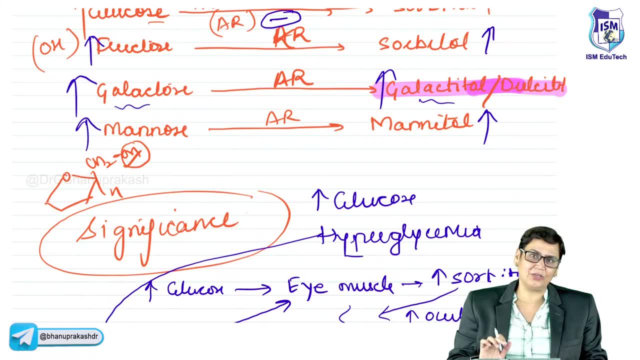 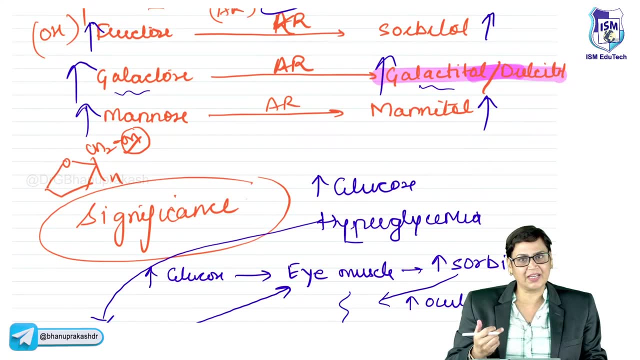 So we will be discussing when. we will discuss the metabolism, Right? so these are what these are: the reducing property. then, coming over to mannose, which is again a reducing sugar, it forms mannitol. now what is the significance of this mannitol? this mannitol decreases the intracranial pressure. 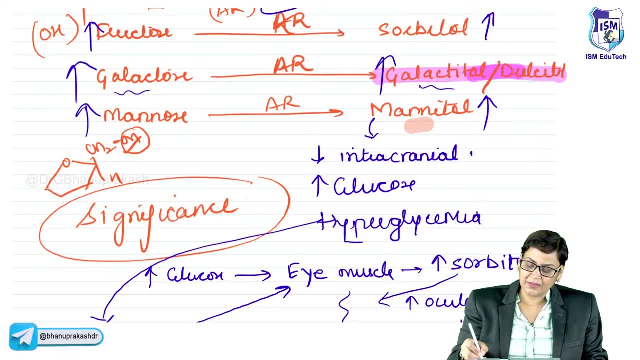 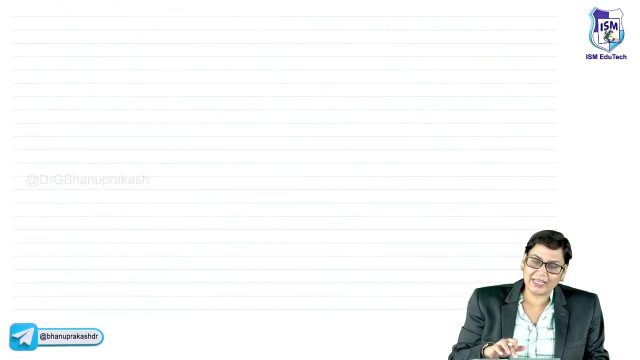 So in any injury, what will happen? this mannitol is given, so it will immediately decrease that Which Is there to heavy flow of. yeah, Right, so this is what this is the reducing. So today, what we have discussed in today's live session, let me just quickly summarize it. what we have discussed this: we have discussed the properties of 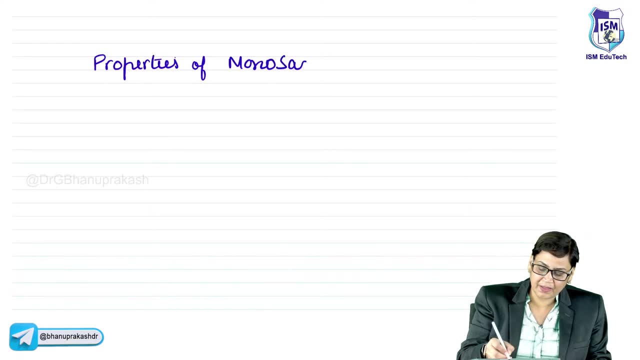 Mono securite Right and what properties I have basically focused on. We have focused on anomers, If you're getting at C1.. We have discussed about epimers, if you're getting at any other position except C1. Then we have discussed about reducing sugars. 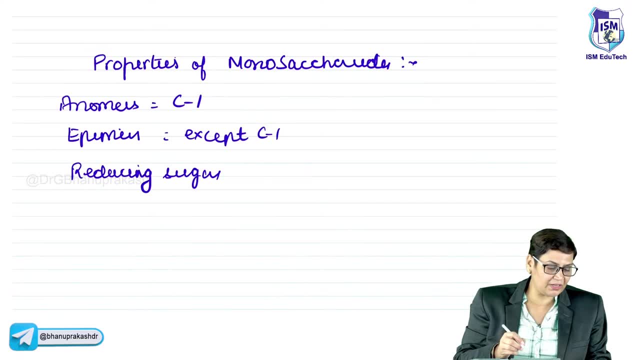 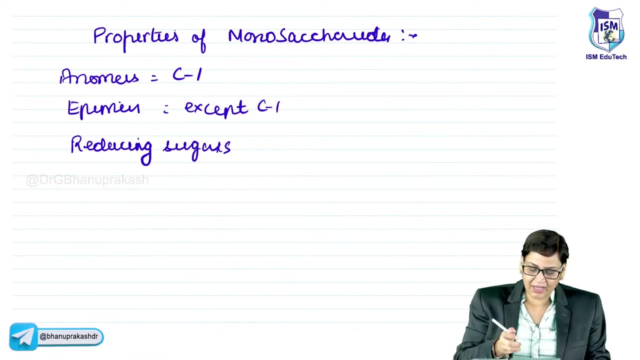 The reason I'm just by. I'm giving you the gist of the lecture so that in case of any confusion, you can ask me. now also Reducing sugars we have discussed, Which have free functional group. okay, then again, non-reducing sugars also, and reducing. 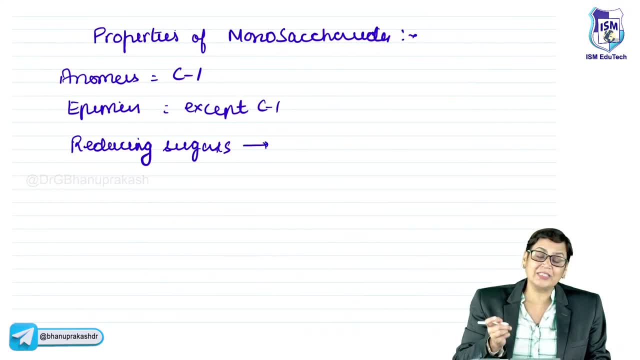 sugars, car in next session, we are going to discuss what is the biochemical significance of these reducing sugars, as just now I told you that this is a very, very important abnormal constituent of your right. then, above all, we have studied about stereo isomers and we have studied about optical ISO. 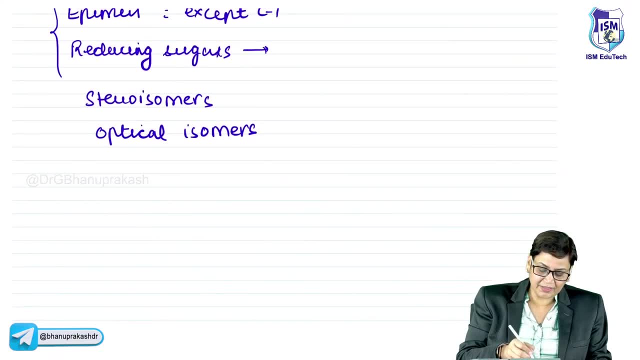 you, along with the properties oxidation and reduction. so I hope whatever we have discussed is clear to all of you. timing- better timing- will be intimated to you. so in the next session I will try to finish up with the entire chemistry of carbohydrate. so if you guys have any confusion you can ask me. 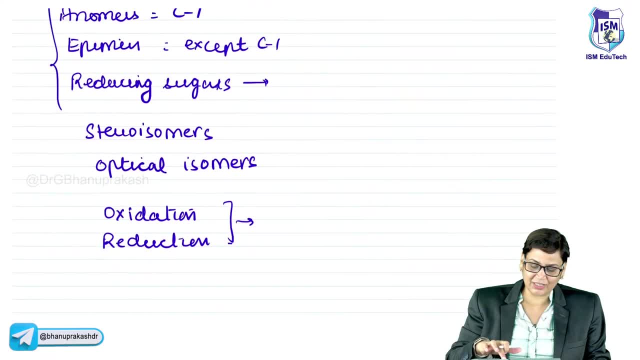 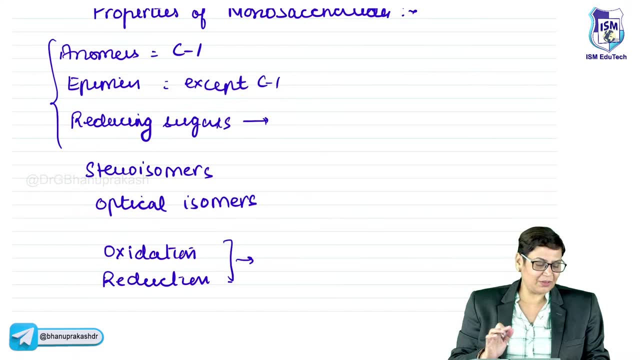 and if you have any questions, please feel free to ask me in the comment box. okay, ground control of this with thisuição. you can ask me in the next session also. okay, I mean automatically will be, we will intimate you about the timings. well, we wind up ok. 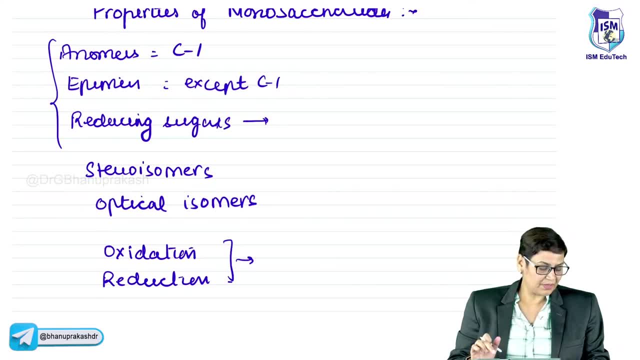 okay, my pleasure Sunday. yeager, you're my pleasure, pleasure. so, yeah, thank you, Dr Abhijit. so see you guys in the next class and try to circulate about my class with your other friends also, so that maximum students can attend the class, because it's like you know, there is a saying in English: the more the merrier, so it will be an. 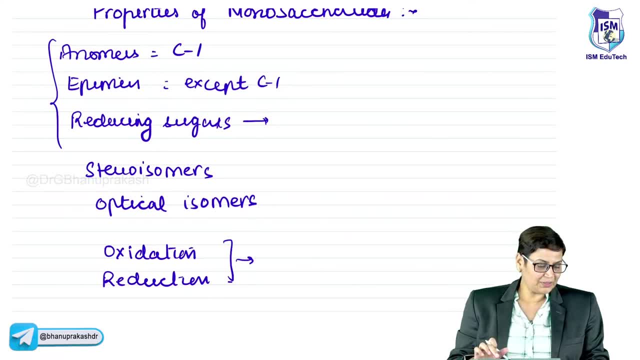 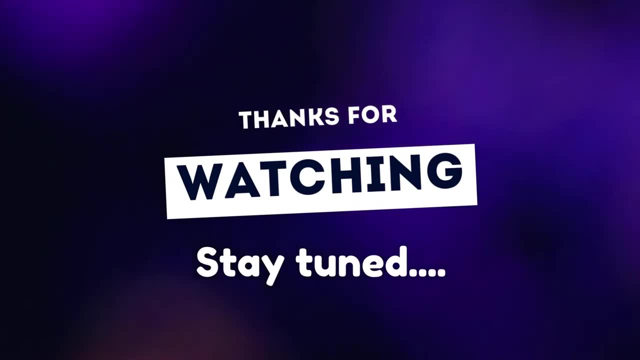 open discussion. so good night, all of you. see you all in the next session. bye you.